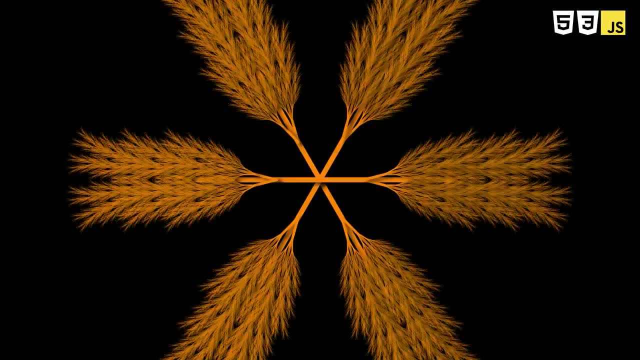 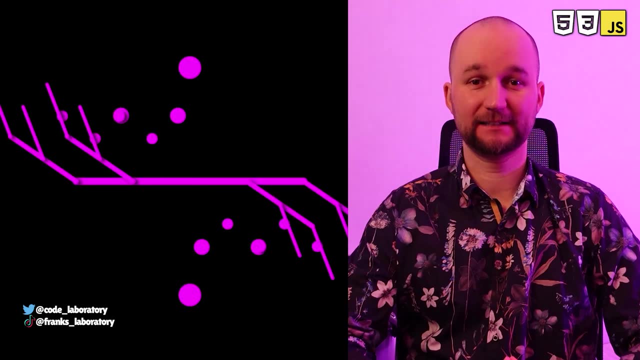 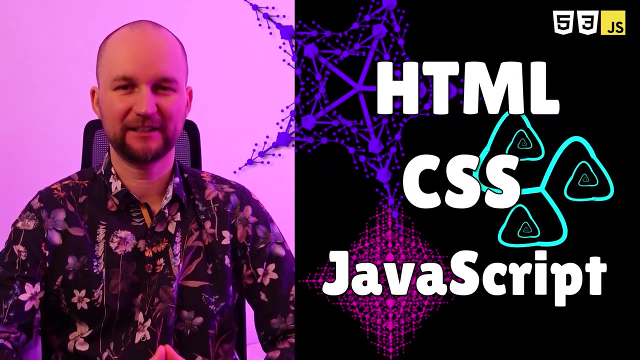 In this class, we will go from drawing a simple rectangle and a line on canvas to beautiful, complex mathematical shapes. Join me and make your unique piece of art with HTML, CSS and JavaScript. Generative art is art that has been completely or partially created by an. 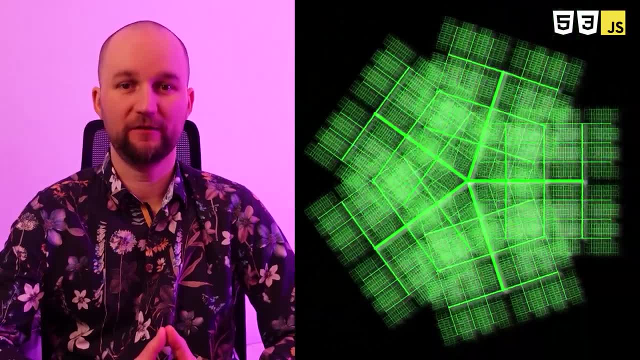 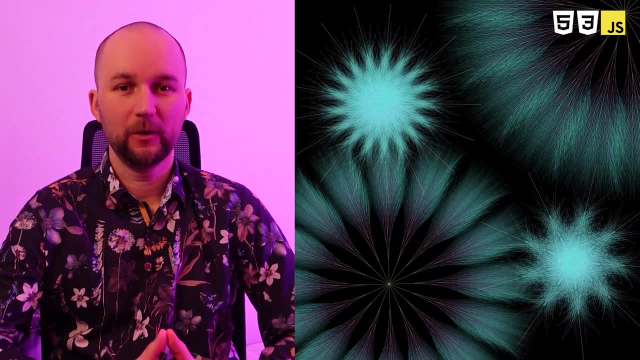 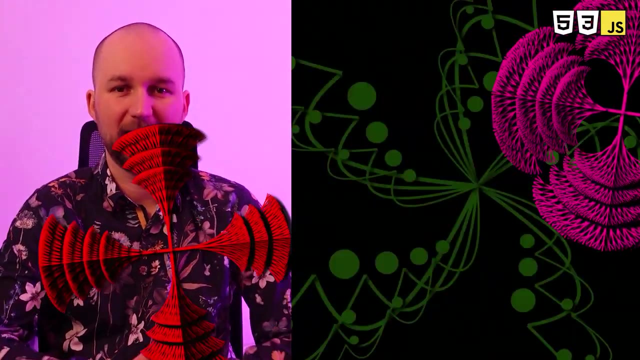 automated system. In today's lesson we will create a program with vanilla JavaScript and we will give it some ground rules, such as what selection of colors to choose from and what shapes to use. We will let JavaScript to randomly decide which combinations of properties and values from ranges we predefined will be used. I like to think of generative art. 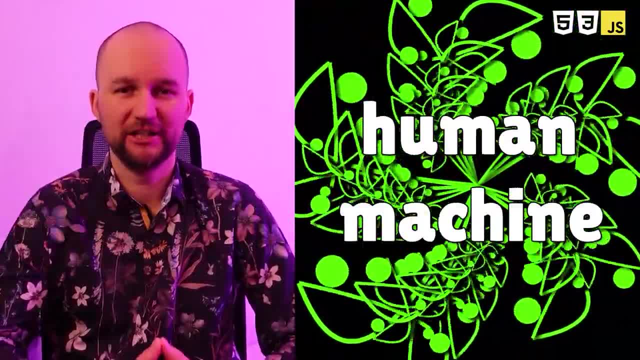 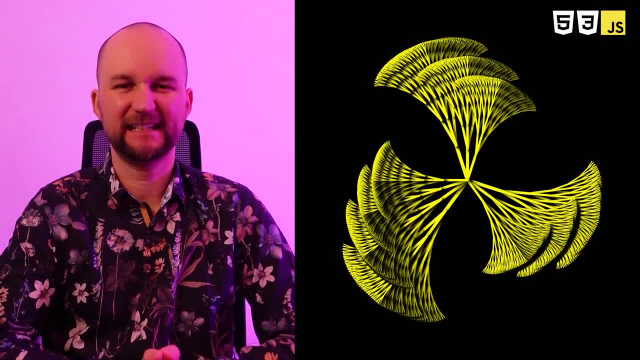 as something that's been partially made by a human, partially by a machine. How much autonomy we give to the machine is up to us. Have you decided that this year you want to become really good with HTML, CSS and JavaScript? Then this video is for you. Welcome to my. 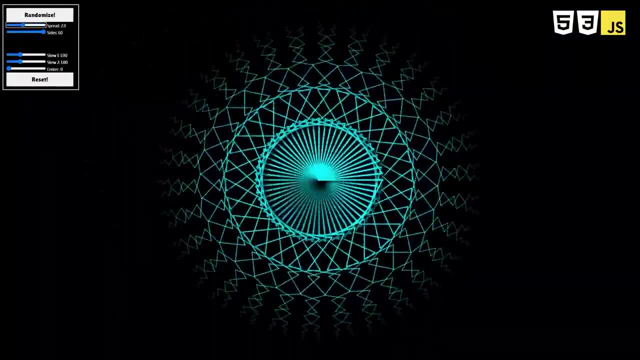 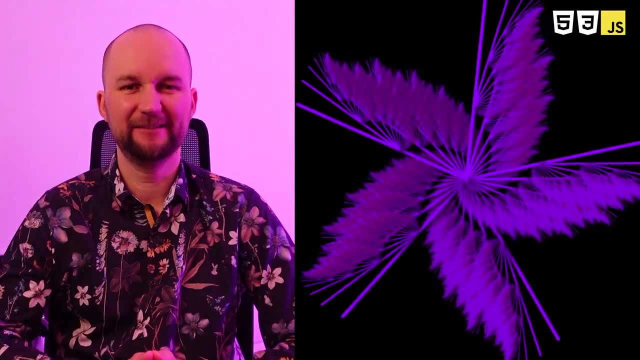 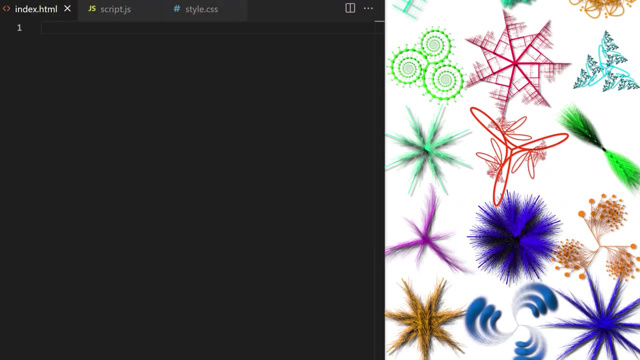 HTML Canvas Crash Course. Today's class is for beginners. Let me give you the tools and techniques you need to bring your creative ideas to life and to take your front-end web development skills to the next level. Have fun. Today's class is for beginners, so I will write the code in a procedural way, line by: 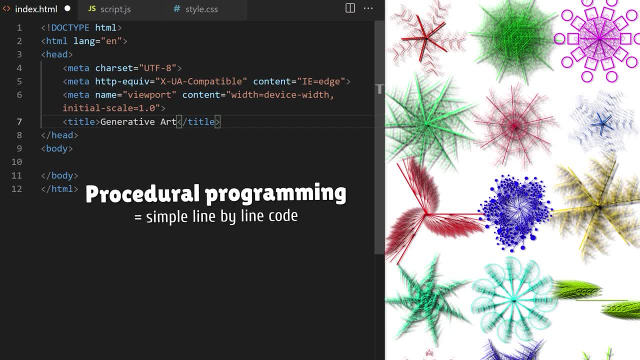 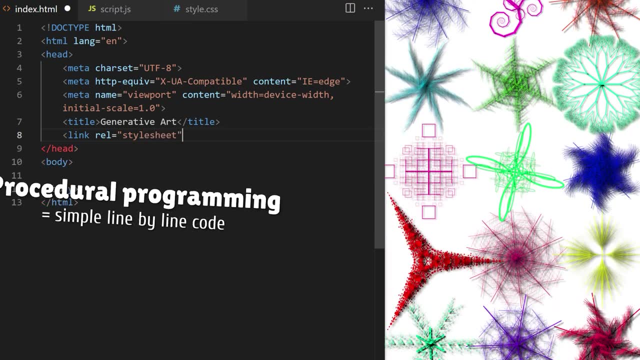 line as simply as I can and we will focus on understanding how everything works. If you want to go more advanced and learn how to use vanilla, JavaScript and object-based oriented programming to render many complex fractal shapes as my new fractal rain effect, 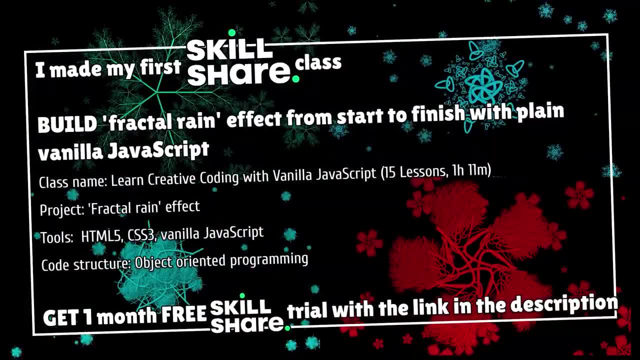 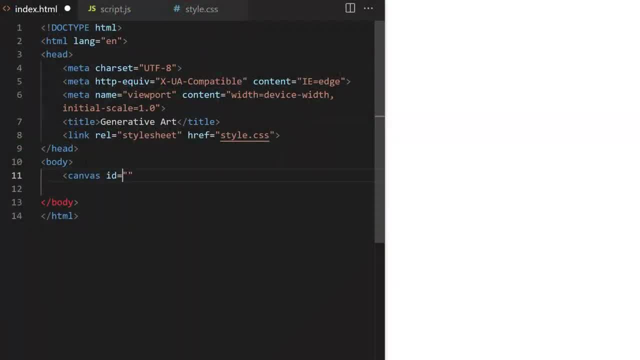 I will be revealing some special techniques in my first Skillshare class. You can sign up for a free Skillshare trial and watch this and many other classes with the link in the description. This is just a simple blank web page. I gave it some title. I linked CSS style sheet. I. 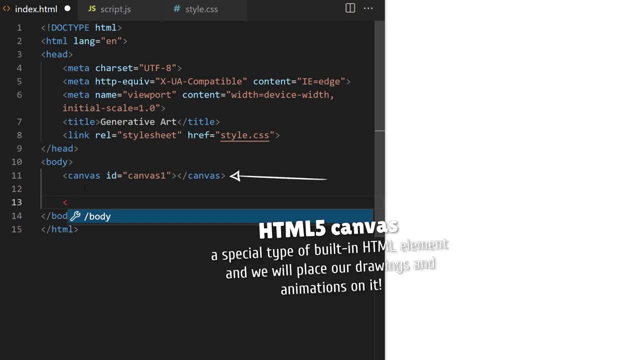 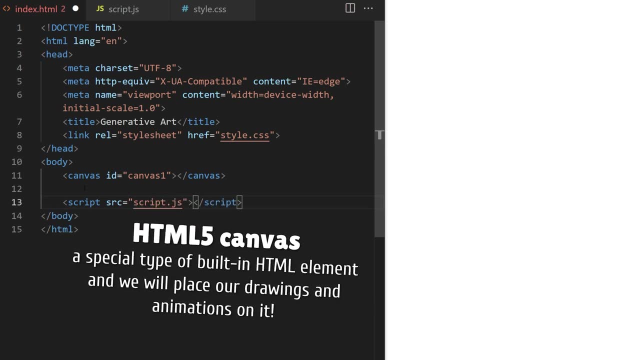 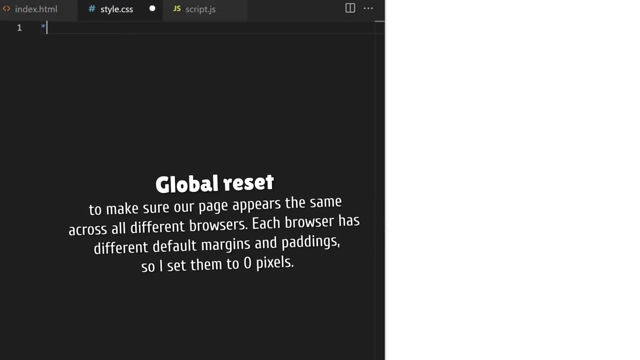 created HTML5 canvas element with an ID of canvas1.. This is a special type of built-in HTML element and we will place our drawings and animations on it. I will also link scriptjs file which will contain all JavaScript logic In stylecss. I do a global reset to make sure our page appears the same across all different. 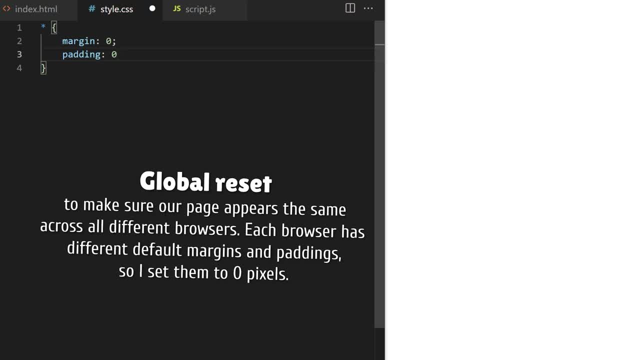 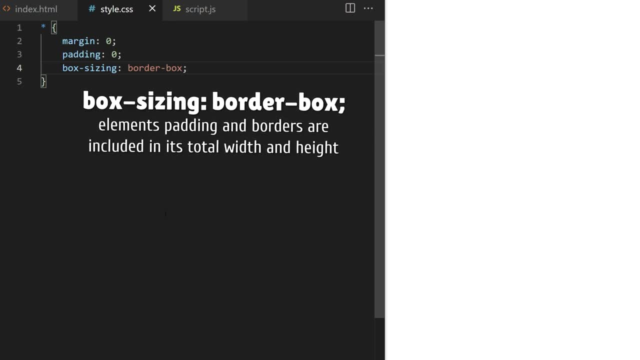 browsers. Each browser has different default margins and padding, so I set them to 0 pixels and I set box size into border box, which means elements, padding and borders are included in its total width and height. This makes creating layouts much easier. I take my canvas element and I give it blue background, just so that we can see where 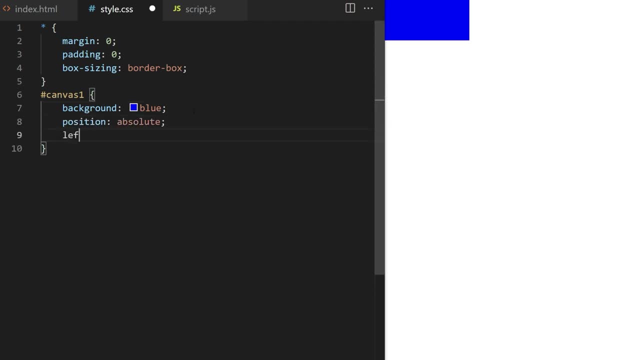 it is right now. I give it position absolute and I set its left and top positions to 0 pixels. In scriptjs I wrap all my code in event listener. We will listen for load event. Load event fires after all assets on our web page, such as all HTML elements, all images and all style. 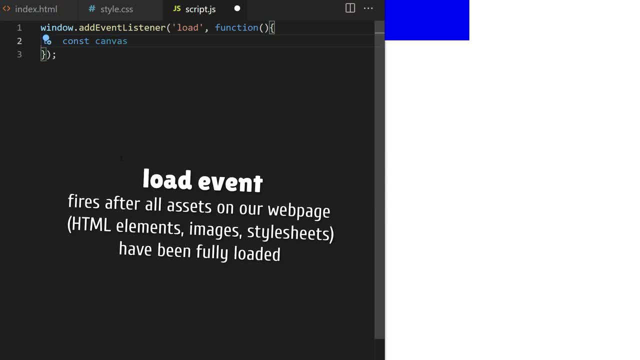 sheets have been fully loaded. Only after everything was fully loaded, we will run this code and set canvas up. I create a constant variable called canvas and I point it towards our HTML5 canvas element using getElementById, Ctf, CTX. shortcut for context is this: canvas variable from line 1, dot, getContext, and I pass it 2D. 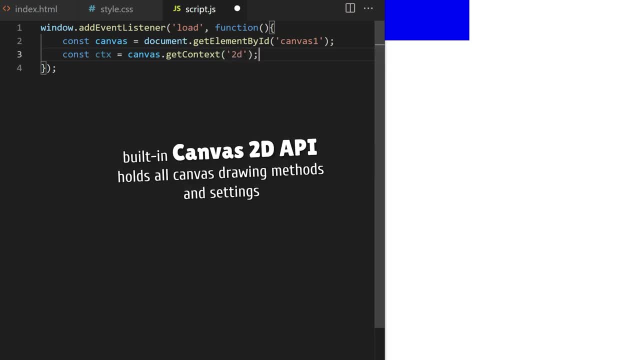 This creates a special instance of built-in canvas 2D API which holds all canvas drawing methods and settings. If you consolelog ctx, you will be able to see them. I set canvas width to the width of browser window and height will be the height of browser. 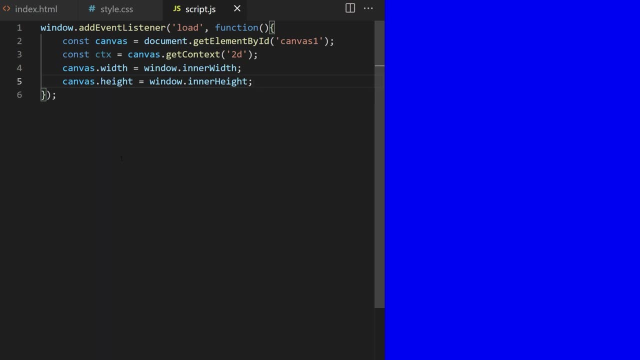 window. If you are new to canvas, the one thing you have to understand is coordinate system. Our canvas is this entire blue area. We have horizontal x-axis which starts from position zero on the left and increases as we move towards right On the positive direction on horizontal x-axis. 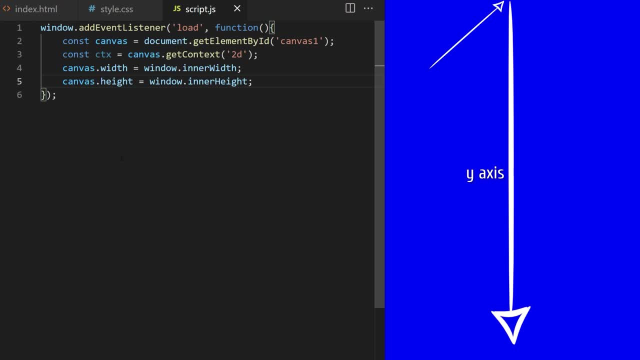 We also have vertical y coordinate which goes from position zero up top and increases as we travel down. So, for example, coordinates 200,200 will be here, 200 pixels from the left edge and 200 pixels from the top edge. Now let's look at our canvas from the horizontal x-axis. 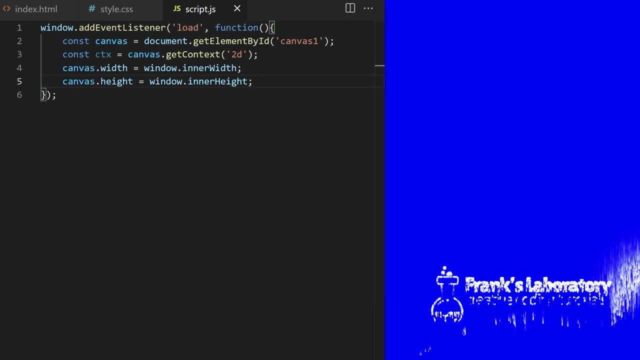 In our canvas at the bottom we will have the axis index and the horizontal x-axis as the left axis. We will also find theics and sets which our canvas is all putting to the left methods, and I can call all of them from this ctx variable we have here on line 2.. I can, for example, 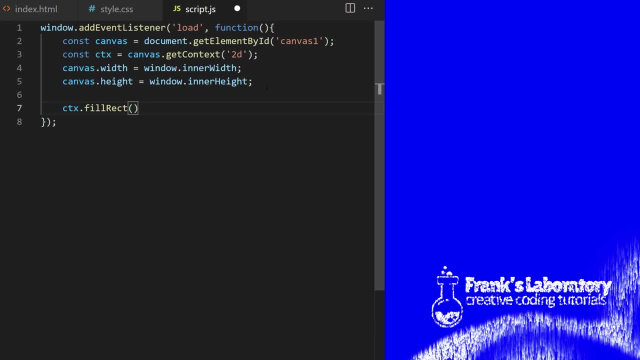 call fillRectangle method. that expects four arguments and it will draw a rectangle shape on canvas. We need to give it starting x and y coordinates and width and height of that rectangle. so I pass it, for example, 10- 10 as starting x and y and 100- 100 as width and height. I can change. 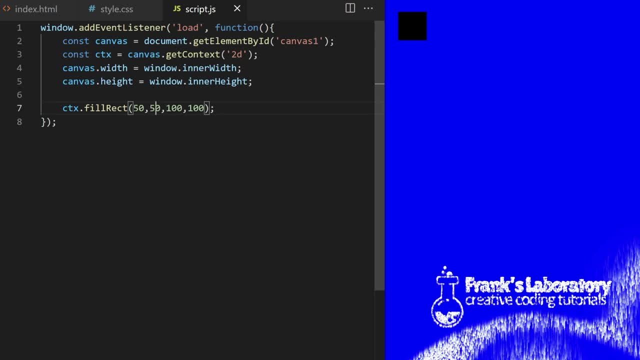 these values to move it around canvas. If you consolelog ctx and look for its fill style property, you will see that by default it's set to black. We can override that default value by declaring it. here I can say: ctxfillstyle is, for example, green and everything that comes after this. 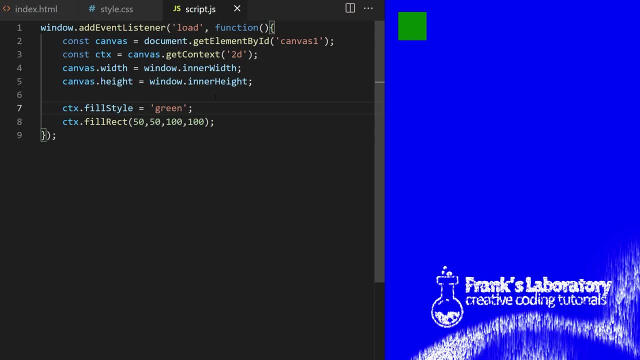 declaration in my file will be filled with green color unless I change it to a different color later in my code. We can also use built-in canvas methods to draw a line. Line is considered a path and to draw a path we can use a line. We can also use built-in canvas methods to draw a line. 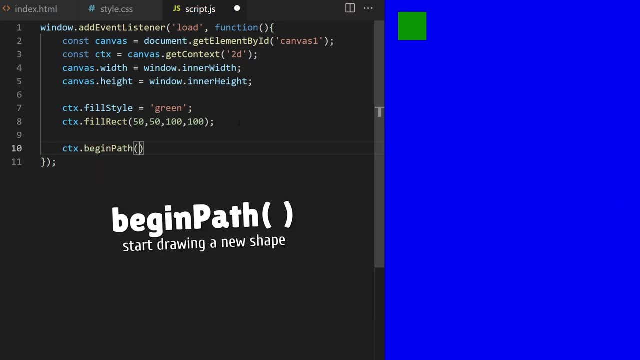 To draw a path on canvas, we need to start by calling beginPath like this. Think of it as if we are placing a pencil on canvas. We are telling canvas: we want to start a new shape. This will also automatically close a previous path if this is not the first shape we are drawing. To draw a 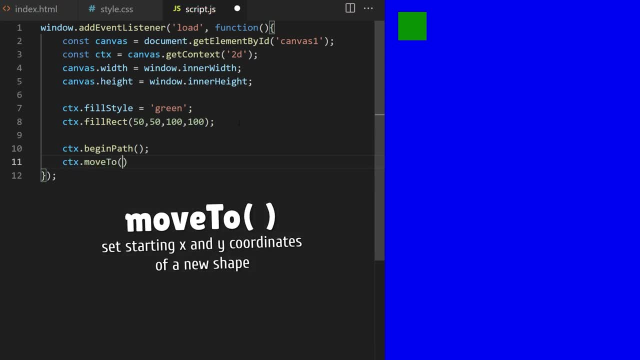 line. we set its starting x and y coordinates by calling built-in moveTo method. Let's say I want my line to start at horizontal x coordinate 200 and vertical y coordinate 200. Then we need to give it ending x and y coordinates. We can also use built-in moveTo method to draw a line. We can 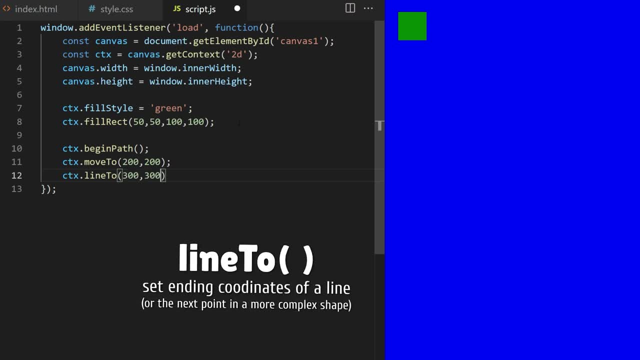 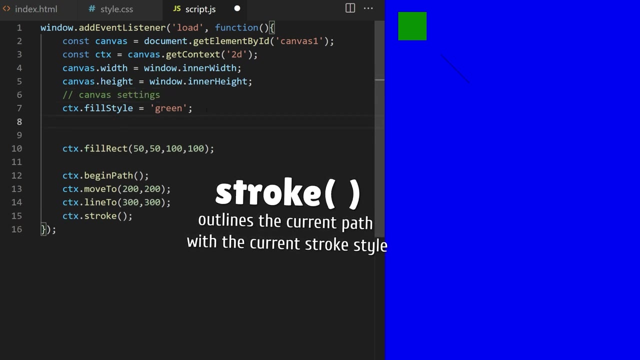 also add a line to the end of the line using line2 method. I want my line to end at coordinates 300, 300.. We have a thin black line here. Let's change some default canvas settings to make the line more visible. Line is a path so it doesn't react to fill style color. I can set stroke style to. 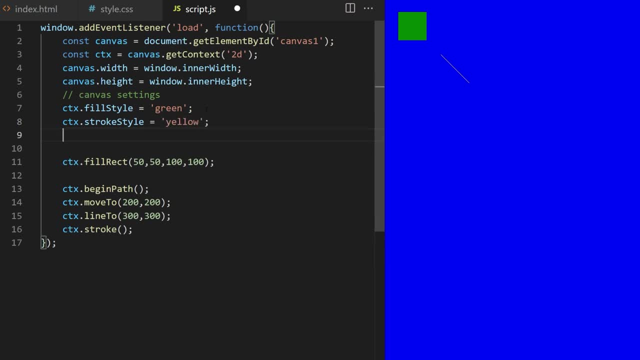 give it a different color. Let's do yellow. I can also make the line wider using built-in line width property. There are many other things we can do with this line. Look at what happens when I set linecap property to round. It gives both endpoints of the line round edges. So right now we are 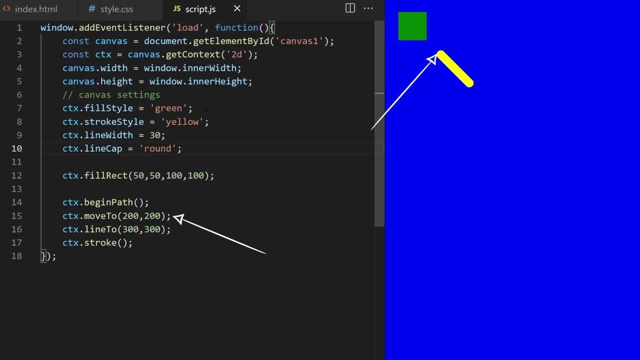 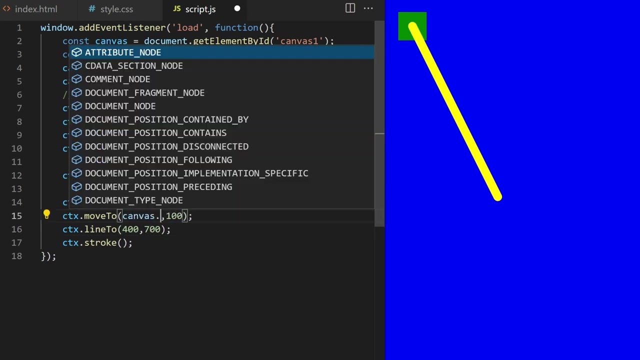 drawing a line from coordinates 200, 200, as declared in moveTo method, and the line ends at coordinates 300, 300, as declared in line2 method. I can adjust these values to draw my line anywhere I want. What? if I want my line to start exactly in the middle of canvas, I can pass it, canvas. 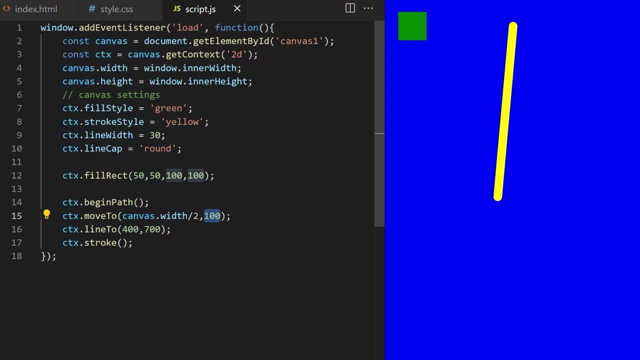 width from line4 divided by 2, which is the middle of canvas horizontally, And canvas height from line5 divided by 2, which is the middle of canvas vertically. So now, these are the starting coordinates and these are the ending coordinates. I adjust the ending coordinates. 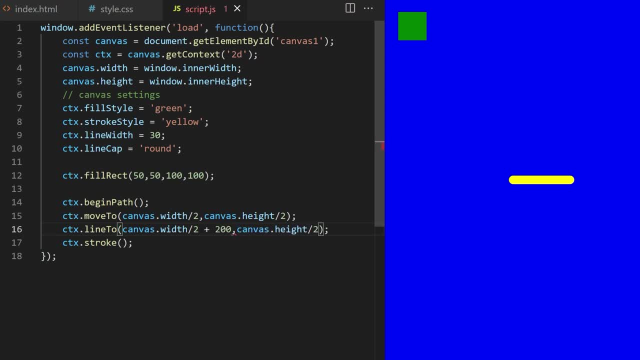 as well. like this Line will always be drawn between these two points. We can give it any values we want. We are drawing fractals today, so let's create a new area for global effect settings. here I will have a variable called size. It's a let variable because I will be changing its value. 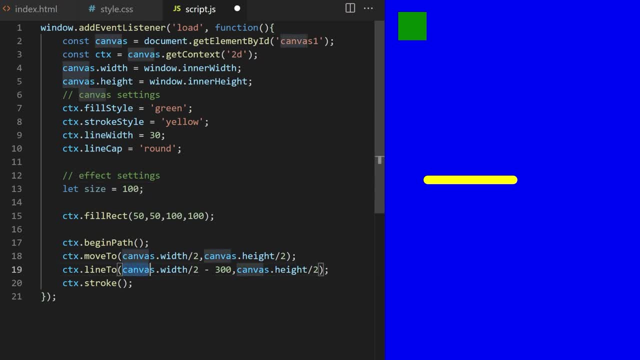 to make it a little bit smaller. I can also change the value of the line width to make it a little more responsive. I set it to 100 pixels and I replace this value here. Now, as I change the size value, the length of the line changes as well. I remove this rectangle. What if I want to rotate? 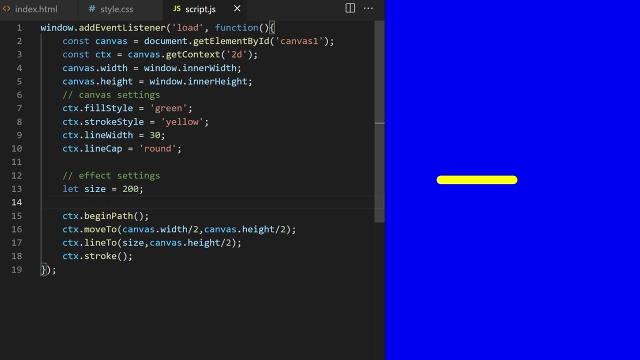 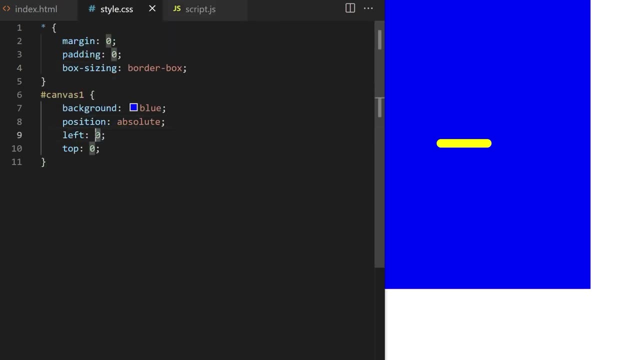 my canvas drawings To better see what exactly is going on. I will make my canvas only 80% of browser window, both horizontally and vertically. In CSS I center it in the middle of the page by giving it left 50%, top 50% and bottom 50%. I can also change the length of the line to make it a little bit. 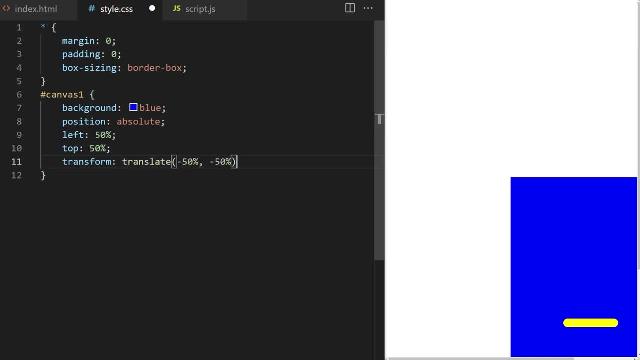 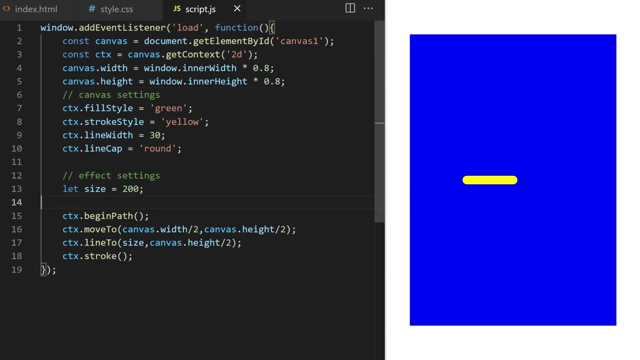 smaller. I also change the width to be 50% and transform translate: minus 50%, minus 50%. So now blue area is canvas element. white area is body of the web page. I will draw a new rectangle and this time I want it to cover the entire canvas, so I draw it from coordinates. Its width will be canvas. 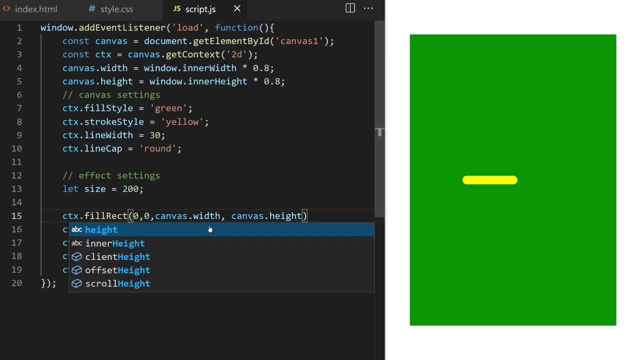 width and height will be canvas height. Notice that shapes are drawn as JavaScript runs through this file line by line, from top to bottom. I'm drawing green rectangle first. I'm going to draw rectangle And line is drawn after, so it will be drawn on top of it If I drew line first. 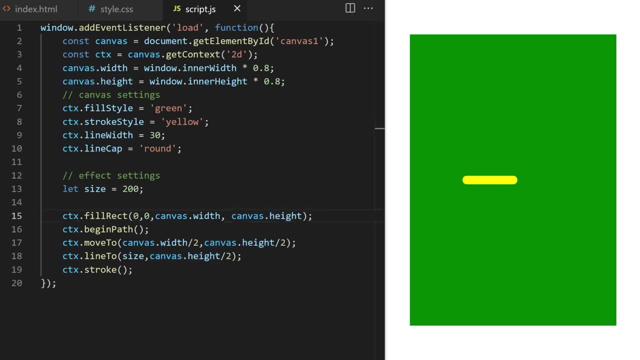 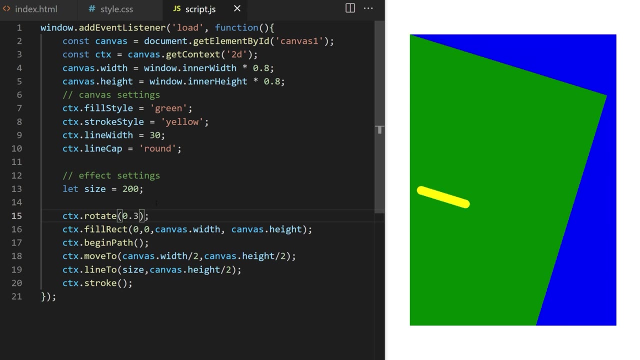 and then rectangle. rectangle would be covering the line Canvas. rotation is simple, but it's not intuitive unless someone explains it. Let me show you how it works. I call built-in rotate method here You can see that it rotated: green rectangle and yellow line, Blue color behind it is canvas. 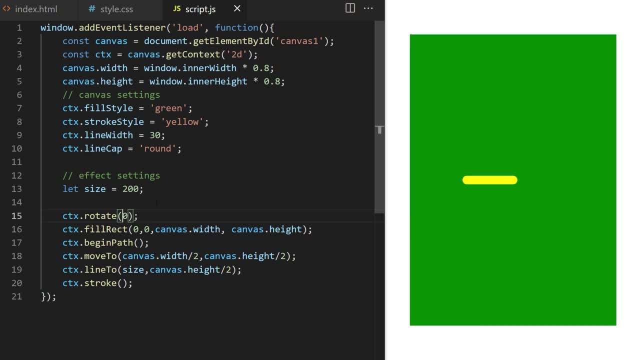 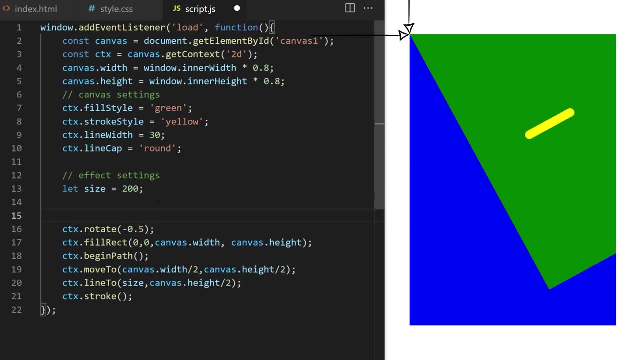 element. If I change rotation angle, it becomes clear that rotation center point is the top left corner of the page. I can also change the size of the rectangle to be the same length- Here you can of canvas coordinates 0, 0.. We can move rotation center point around by using built-in translate. 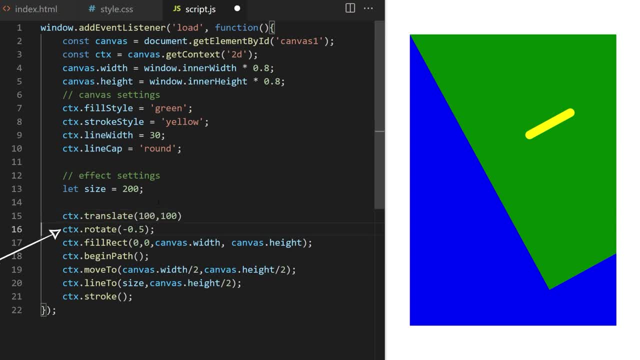 method. I need to call translate before I call rotate. for this to work, I translate rotation center point, what would be normally coordinates 0, 0 on canvas to coordinates 100, 100 and then we rotate from that point. If I change rotation angle again, you can. 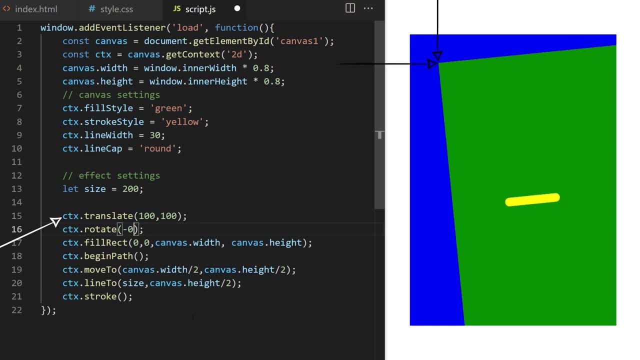 see that rotation center point changed and translate method also changed. what is considered coordinates 0, 0. so this green rectangle that should start from coordinates 0, 0 actually starts from coordinates 100, 100.. If I give translate different values, you can see it. 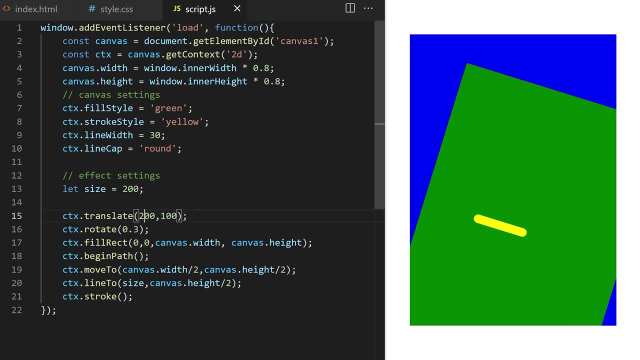 moves both rotation center point and those 0, 0 coordinates with it. Translate method also sets center point for scale in canvas. If I call built-in scale method and I pass it two mandatory arguments for horizontal and vertical scale, you can see that everything. 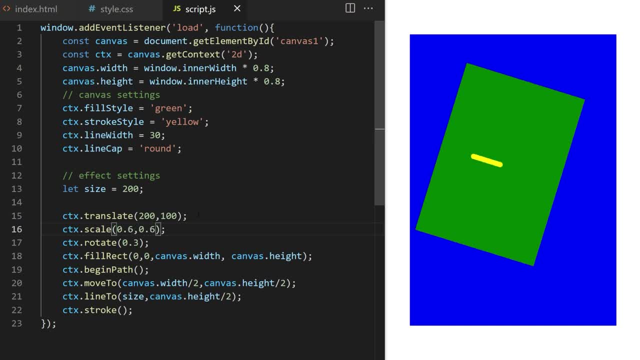 shrinks towards the coordinates I declared in translate. You can play with these values and see what happens. It's very important to understand how translate method affects rotation, center point, scale in center point and coordinates 0, 0.. Also, keep in mind that javascript files are read and executed from top to bottom. 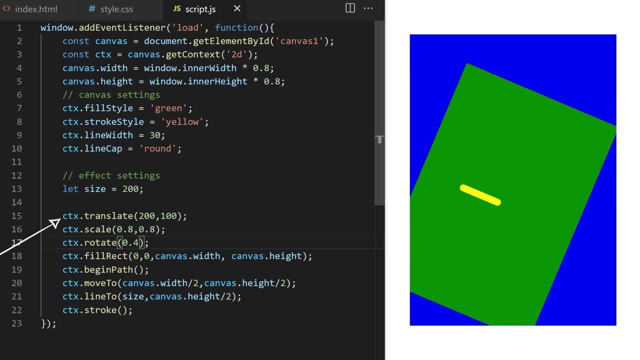 So in simple procedural code structure like this, these translates, scales and rotates only affect rectangle and line because they are drawn after it. If I drew another rectangle but put that code here before my translation, it would only affect rectangle and line because they are drawn after it. If I draw another rectangle but put that code here before my, 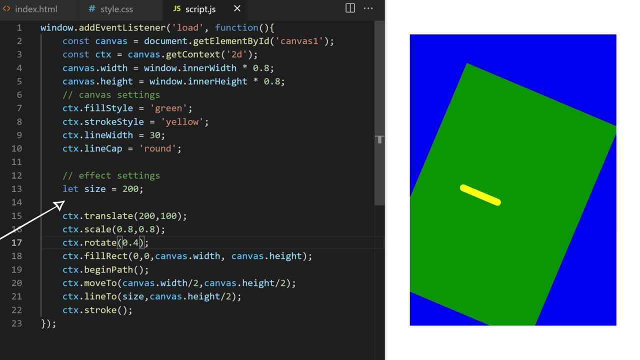 translation, it would only affect rectangle and line because they are drawn after it. If I draw another rectangle but put that code here before my translation, it would only affect rectangle and line because they are drawn after it. I think, playing with this for a while and passing different arguments to translate. 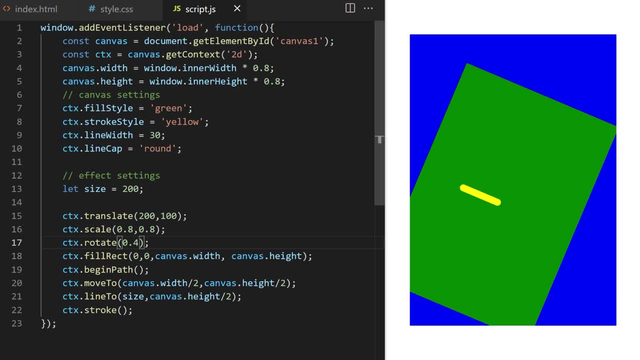 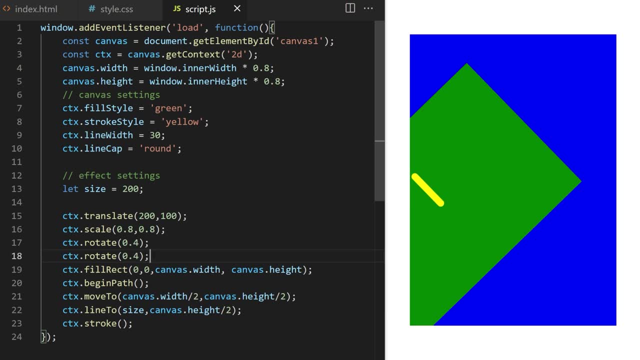 scale and rotate will make it very clear what exactly is happening. The last important thing about translate scale and rotate canvas methods we need to understand is that they add up. If I declare rotate three times, it gets applied three times and rotates canvas further every time we call it. It doesn't override itself. the 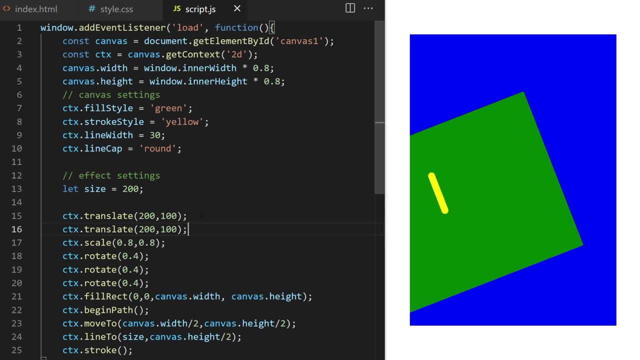 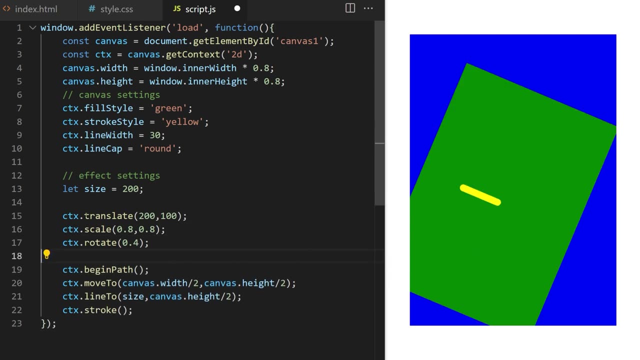 way CSS transforms do, It just adds up. Same goes for translate and scale. By calling translate twice, like this, I'm actually translating two coordinates: 400, 200.. It adds up Same with scale If I take the code that draws green rectangle and I place it before translate scale and 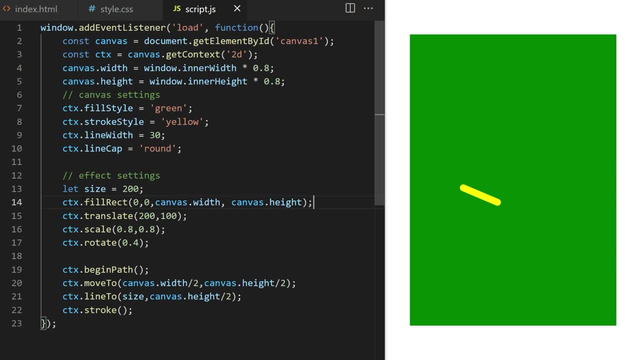 rotate, it will not be affected by them at all, But the yellow line that is drawn after will still remain translated, scaled and rotated. I put the green rectangle back by doing this. Sometimes in our projects we want translate, scale and rotate to only affect certain shapes. 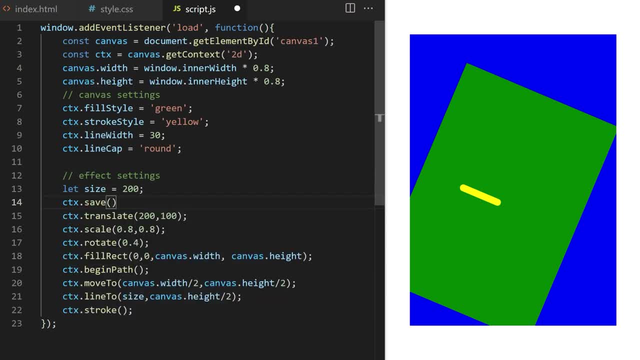 and then we want it to reset back to normal so that other shapes remain unaffected. For that we have two very useful built-in methods called save and restore. I will call save here, before my translate, rotate and scale, and I call restore here. 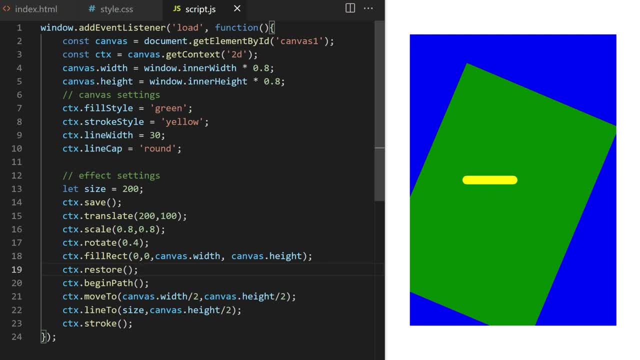 after I drew green rectangle, but before I draw yellow line. Now you can see that green rectangle is translated and rotated again. That would be the end. If I take a look at other tools before I draw yellow line, I would notice that when I drew 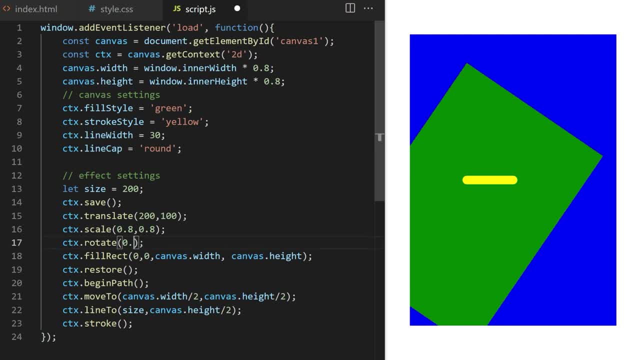 translated, rotated and scaled, but the yellow line is not affected. Built-in canvas save method saves the entire state of canvas, not only translate, rotate and scale, it saves all canvas properties and their settings at that point in our code base, including things like fill style. 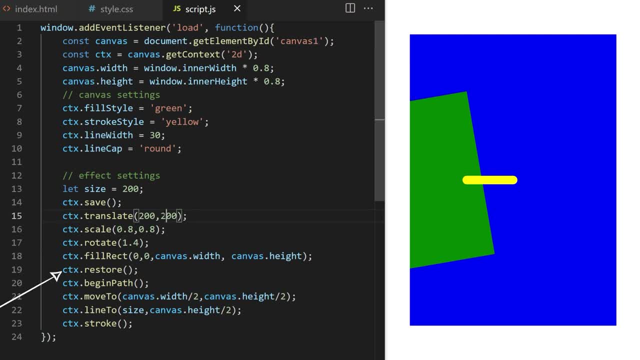 line width and so on. When we call restore, it restores the most recently saved canvas state for us. So in this case we save canvas, we translate, scale and rotate, we draw rectangle, we reset things back to default. so we removed all translating, scaling and rotating so that the 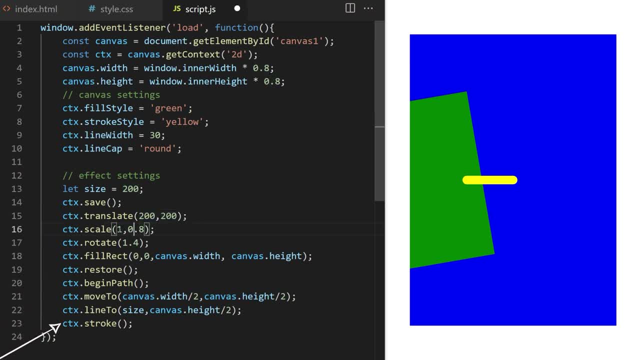 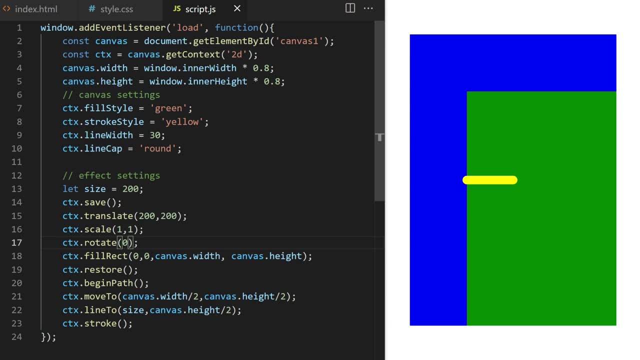 yellow line that is drawn after is not affected by these. Whatever I do in this area between save and restore will affect the green rectangle but not the yellow line shape. This is all we need to know to create fractal shapes on canvas. Let's translate: rotation, center point and what is. 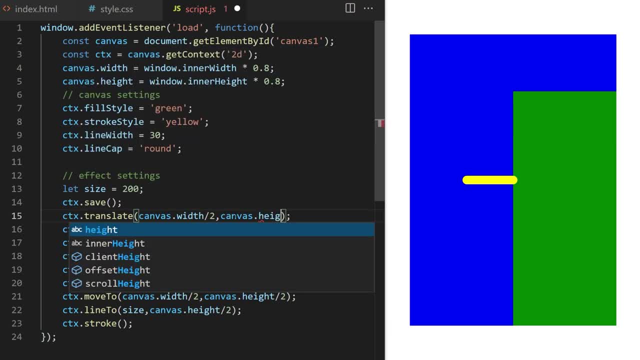 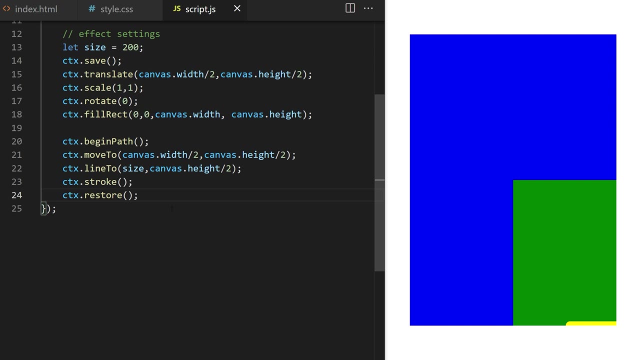 considered coordinate 0,0 from the top left corner to the middle of canvas element, both horizontally and vertically. I will take, restore and place it after the code that draws our line. That way the line will also get translated, rotated and scaled. I want the line to spin around the middle of canvas, so we 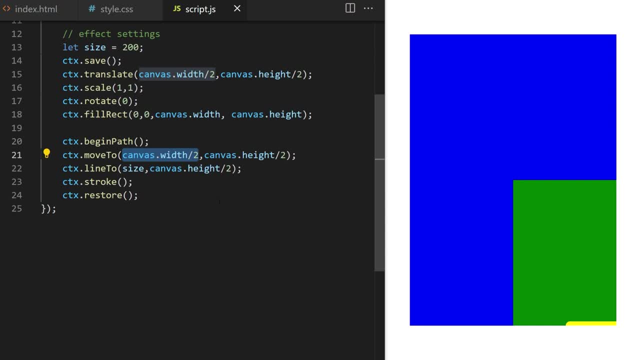 can create one of the symmetrical fractal shapes I showed you in the beginning. On line 15, we are translating rotation center point, and also the point that would be considered coordinate 0,0, to the middle of the canvas. If I want my line to be in the middle of canvas, I have to set its. 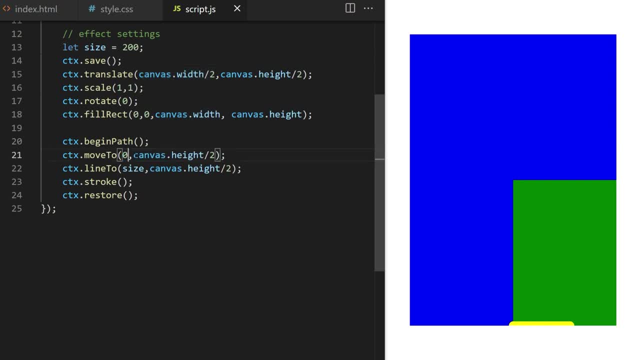 starting x and y coordinates. So now, because we used translate method, starting coordinates of my line are here and ending coordinates are here. If I rotate my canvas, you can see that rotation center point is the middle of canvas. Perfect, Let's comment out the green rectangle. What if, in this space, before I call, 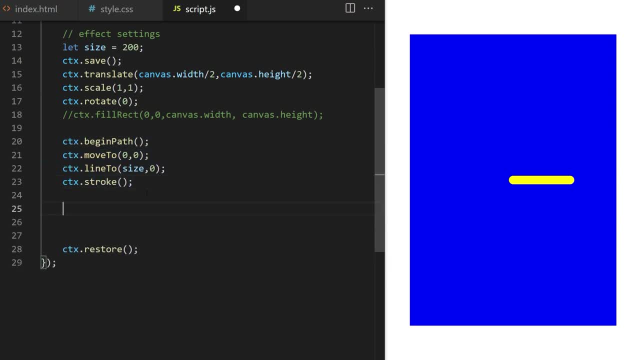 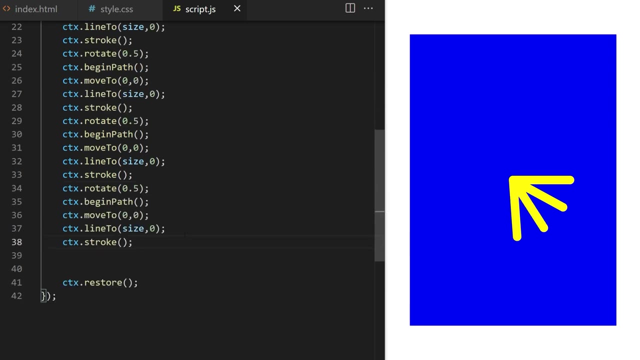 restore, I put more code to draw another line. Now we are drawing two identical lines on top of each other. But how about? I draw one line, I rotate canvas and I draw the other one, And then I rotate and draw another one and another one. 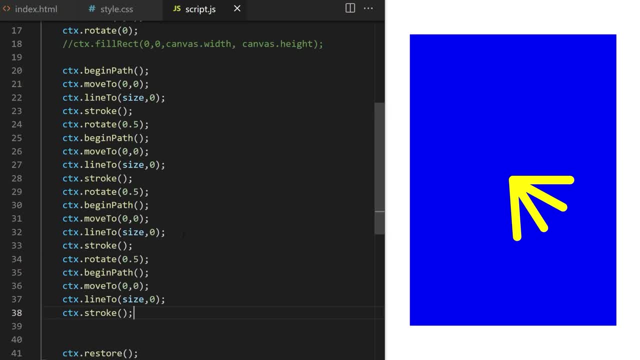 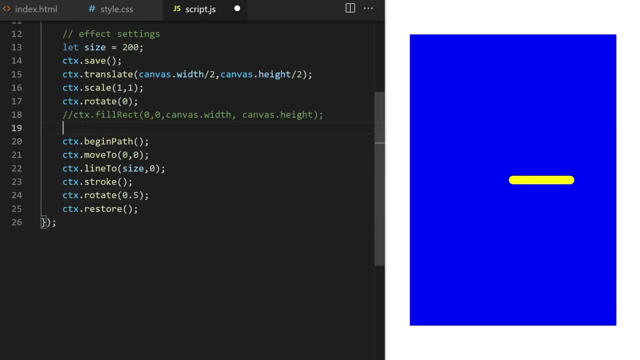 You can see that rotates add up. When you see a lot of code repetition like this, it usually means it's a good time to use a loop. I delete all the additional lines and I create a for loop. It will start at index 0.. As long as index is less than size variable, increase index by 1.. Let's create. 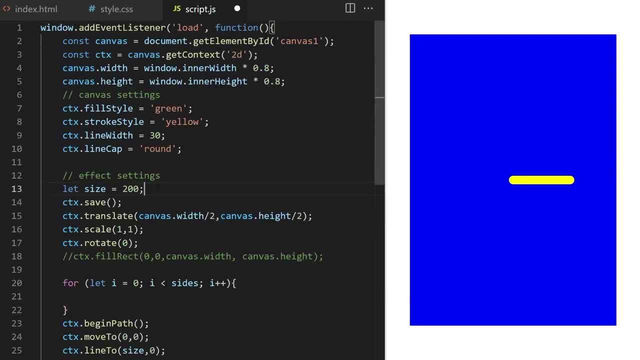 this size variable. It will determine how many lines we will draw and how many lines we will draw And, in the final effect, it will determine how many sides will our fractal shape have. Let's first give it 2.. I put this code inside for loop Each time this for loop runs. 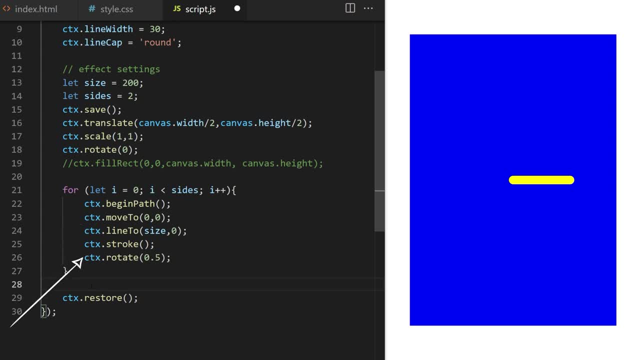 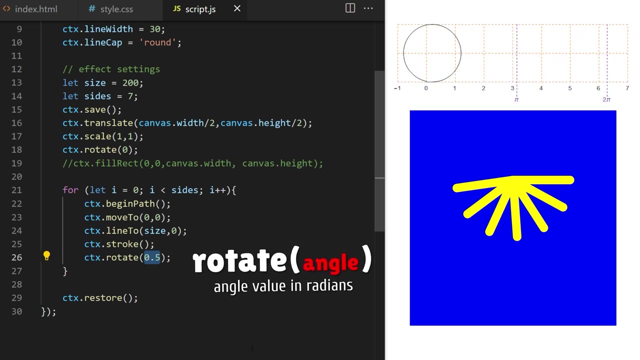 we will draw a line, Rotate canvas by 0.5 radians and we will draw line again as the for loop continues. Now I can increase sides to add more lines rotated around the center of canvas. Rotate method doesn't take angle value in degrees, It needs a value in radians. Half circle is 180°. 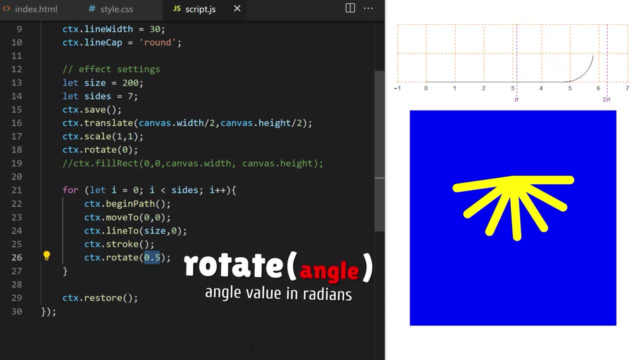 Which is approximately 3.14 radians. It's exactly the value of pi. So if I rotate by mathpi, we rotate by half circle before we draw the second line. Mathpi times 2 is roughly 6.28 radians or 360°. So full circle, which means we drew a line, rotate it around the whole circle. 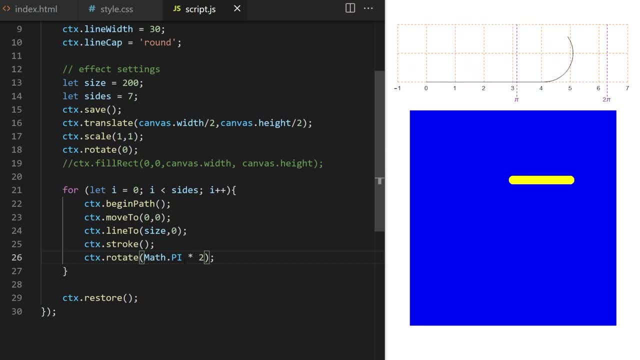 and we drew a line again. So now our lines are covering each other. What if I want to rotate by a value that splits the circle into slices, depending on value of sides variable from line 14.. I can say: mathpy times 2, whole circle divided by. 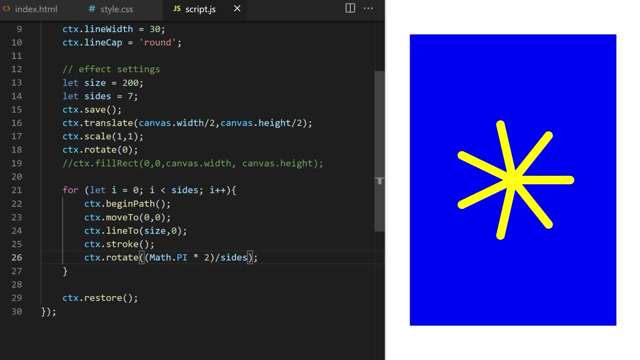 sides, so 7.. Each time we draw a line, rotate canvas by one seventh of a circle. Now, when I increase sides, lines will always rotate so that they slice the whole circle into number of sides with equal size. Look what happens if I reduce scale. every time we draw a line, We get this spiral shape. 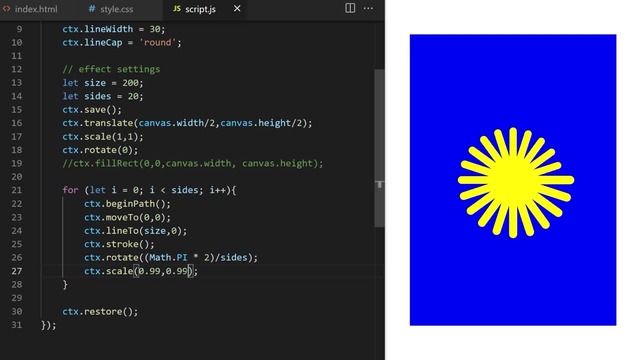 We draw a line, we rotate and scale canvas so that the next line in the upcoming for loop will be rotated and scaled down. Scale also adds up same as rotate. as the for loop runs. I can also displace the starting coordinates by adjusting translate between each loop. These are relatively 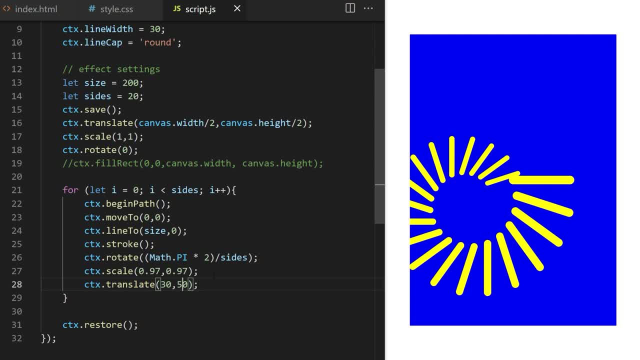 simple shapes. but keep in mind, all of this can be done with more complex fractals and we will build it. by the end of this tutorial. You can create fractals of many different shapes and sizes when you understand the principles we just covered. I delete translate and scale here. Now that we understand how to draw lines on canvas and how to 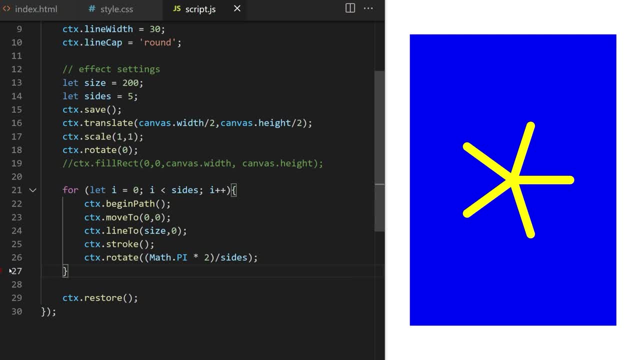 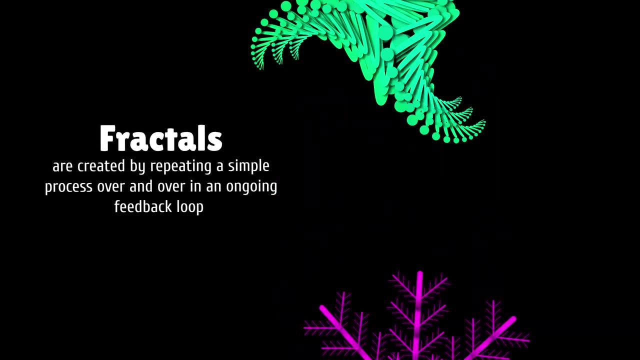 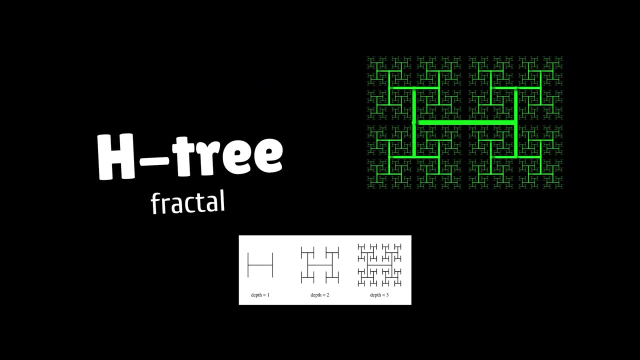 translate: rotate and scale. let's learn about fractals. Fractals are created by repeating a simple process over and over in an ongoing feedback loop. To better understand what this means, let's have a look at my favorite type of fractal. Today's code base will be inspired by so-called H3. 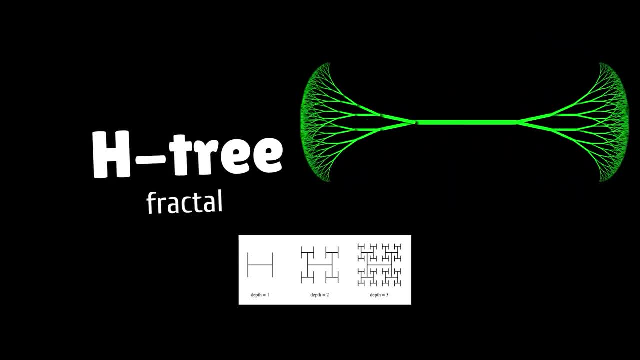 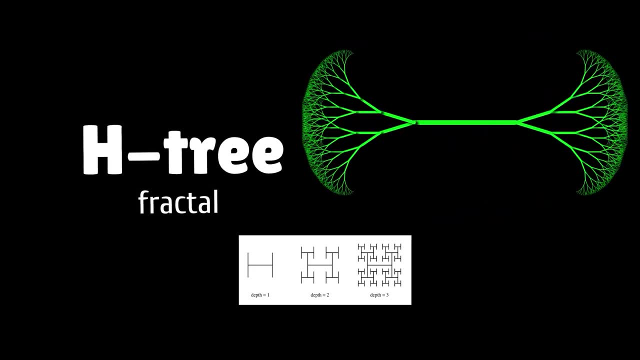 fractal. This is the base shape. When we increase complexity, we get smaller version of that shape at the end of each branch and if we repeat the process again, we get even smaller shapes At the end of all the endpoints. we can repeat this over and over and get into smaller and smaller details. Notice that. 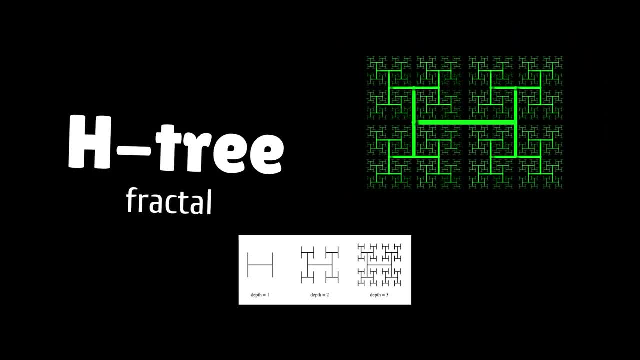 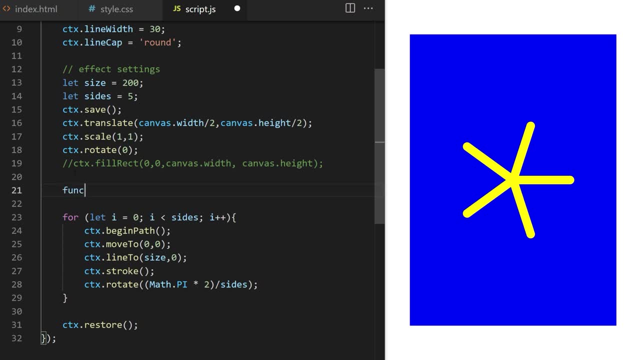 in H3 fractal, the lines are always branching out in the right angle, but if we adjust this angle, we can create beautiful fractal trees and many other things. Let's create a custom function. I call, for example, drawBranch. The job of this function will be to draw a line, rotate canvas and call itself. 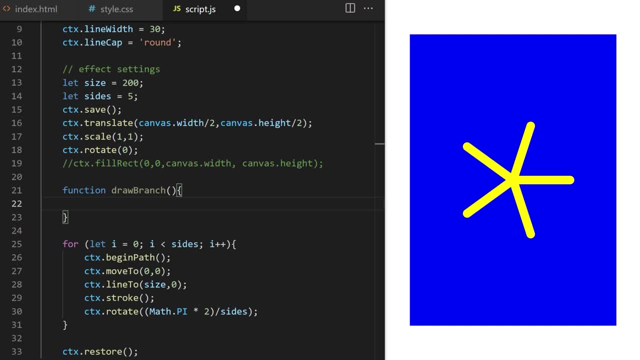 another segment of that line under a different angle. Depending on how many times we allow drawBranch function to call itself, we will get different amount of segments and overall different fractal shape. Let me show you what I mean. I start by drawing a line, so begin path, move to method, to 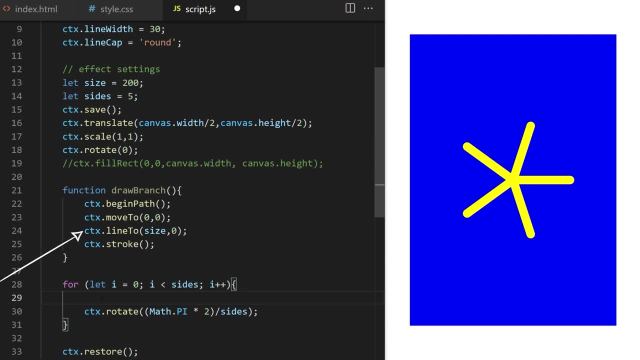 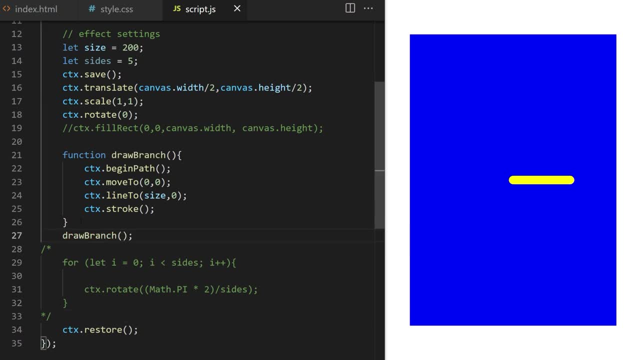 set starting coordinates, line to method to set the ending coordinates and stroke style to actually draw the line. I comment this part out Now. when I call drawBranch, it just draws a simple line. Now I want this function to call itself to draw another segment. but we have to be careful. 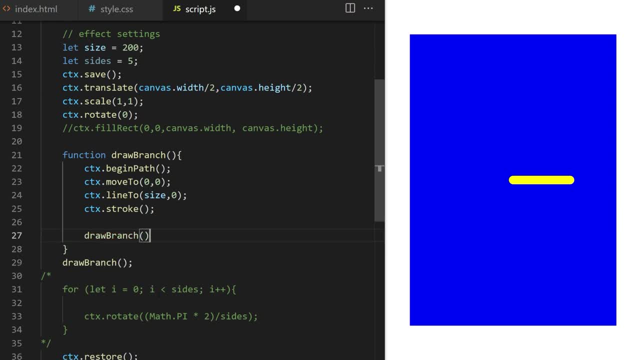 here, because if I just simply call function from within itself, we can create an endless loop and some older browsers might freeze. New browsers will be able to deal with it, but we need to fix it anyway. I need to introduce some kind of limit, some kind of counter that increases every time the 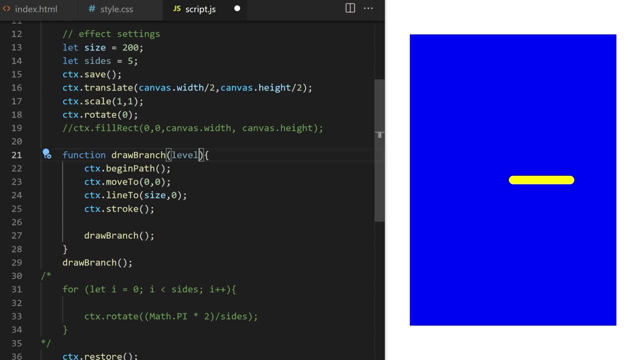 function calls itself and when we reach a certain threshold, the loop will stop. It will prevent the function from doing that. So I create a new variable and I call it level, and each time function calls itself, I increase level by one like this: I need to put level here as well, so that it expects that. 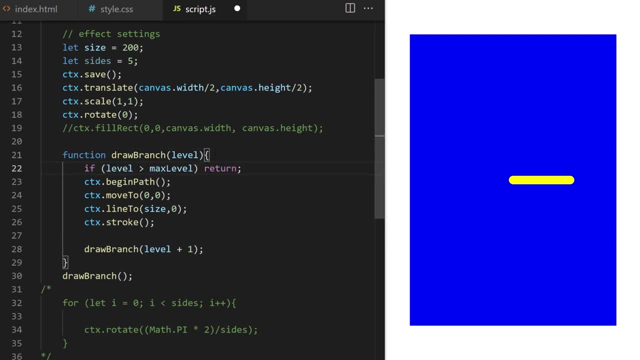 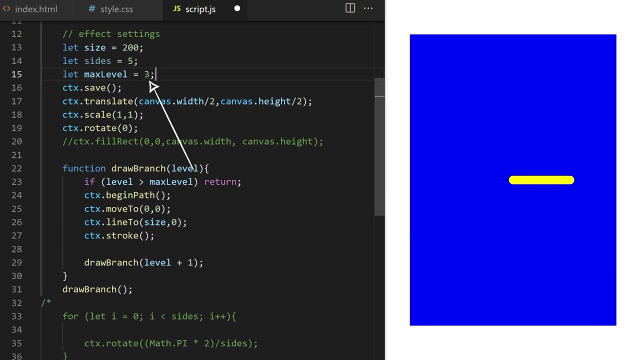 argument and inside I say: if level is more than max level, return. Return is a special keyword in javascript and it is used to exit from a function. When return runs, function immediately stops executing its code. I declare that max level up here and I set it, for example, to three. 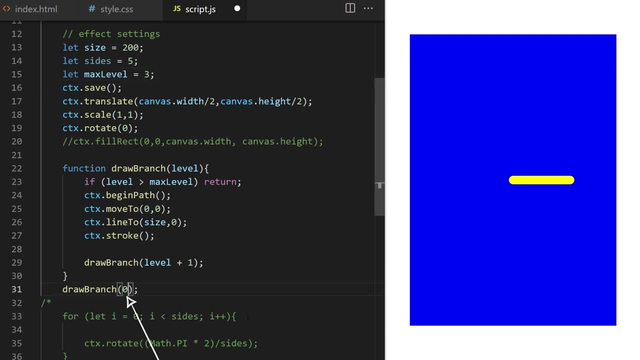 Now I just need to pass it initial value for level, which will be zero. Every time we draw a segment, we rotate canvas by 0.5 radians. I can also scale the canvas between each segment. Let's try 0.9, 0.9.. 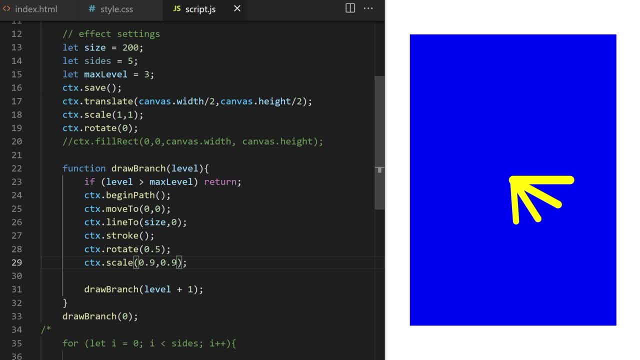 Before I rotate, I can also translate that rotation center point along the branch. Let me show you. Look what happens if I translate by additional 50 pixels horizontally. Now we get each new segment on the branch growing from the middle of the previous one. 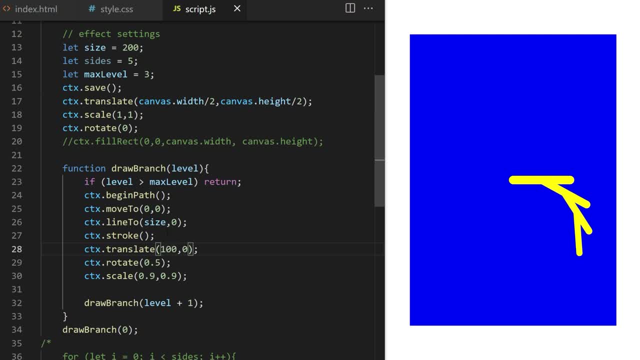 I can change where my segments connect by translating two different values here. I can also change rotation angle between each segment like this, and I can also play with scale. Now we drew a simple branch that consists of four segments. We get four segments because we set max level here on line 15 to 3.. We call drawBranch and pass it level0. 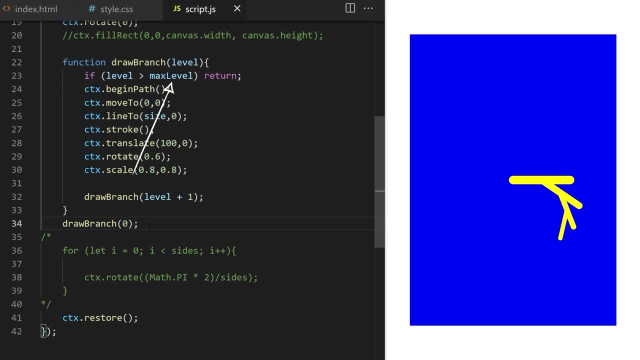 DrawBranch function checks if level is more than max, level 0 is not more than 3, so this code runs and draws 0. a line, then translate, rotate and scale happens and draw, branch calls itself and increases its level by 1.. 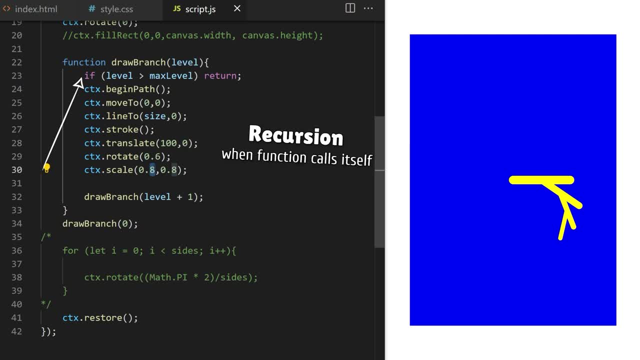 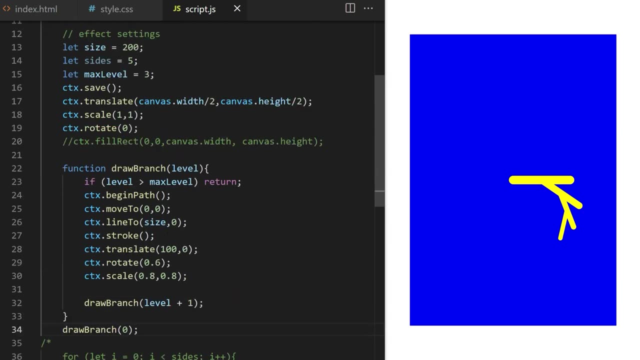 That repeats over and over until level is more than max level. Recursion in programming is when function calls itself. It should have some termination condition so that function can stop repeating itself when that condition is met. We gave it that condition on line 23.. 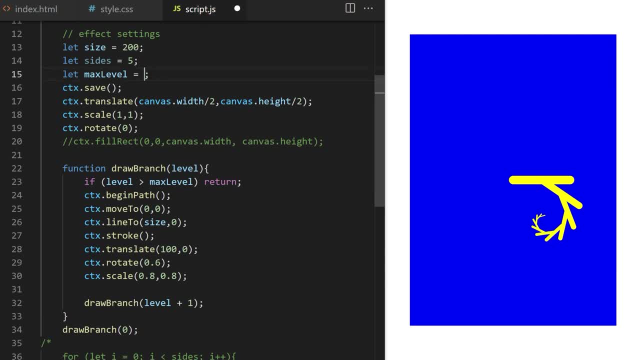 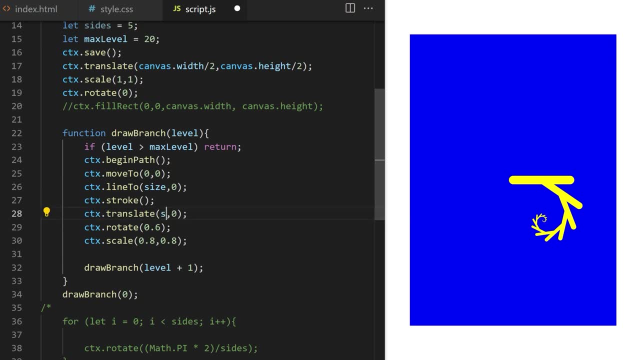 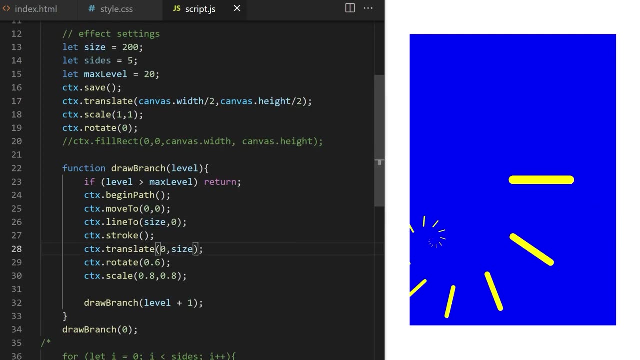 If I increase max level we get more segments because it takes more repeating calls on draw branch before level reaches max level and recursion stops. I can change horizontal x value. I passed the translate method to change where each segment splits from its parent branch. If I want each branch to split into two smaller segments, I can wrap this part between save. 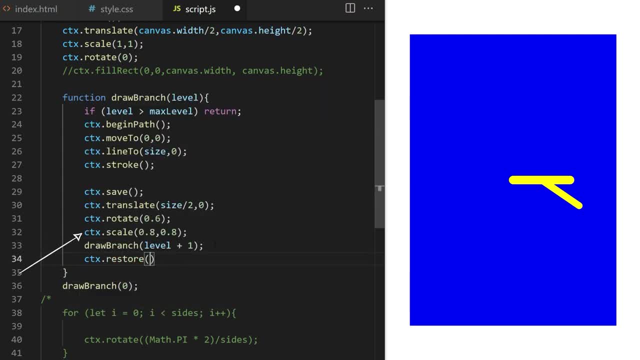 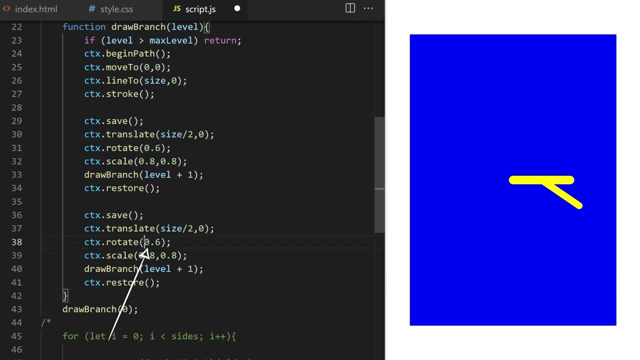 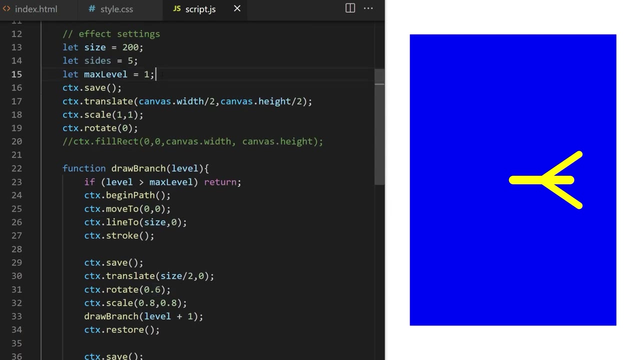 and restore So that this translate rotate and scale only affects this draw branch call. I copy this block and I pass rotate negative angle value to rotate that second splitting segment in the opposite direction from the parent branch. Let's put that angle value in a variable. 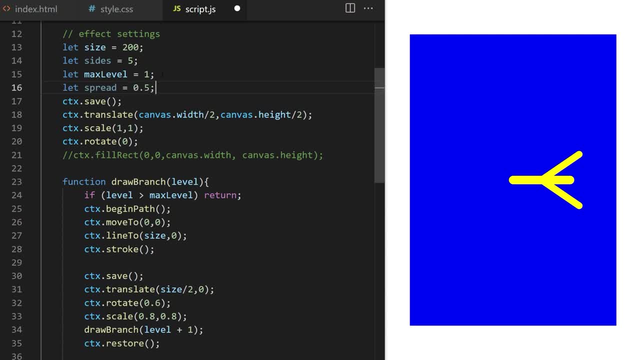 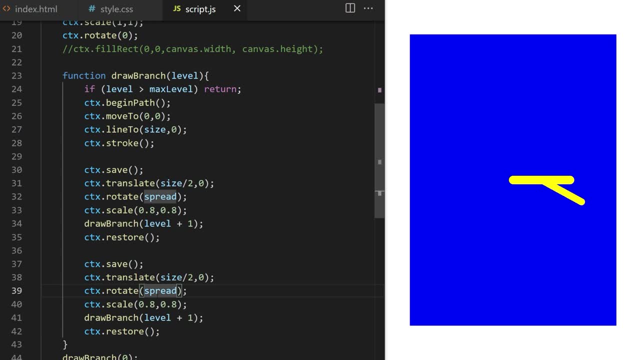 I will call it, for example, spread and I set it to 0.5 radians. Now I replace it here and here. This second one will be a negative value. so minus spread. Look at what happens as the angle by which we rotate branching segments increases. 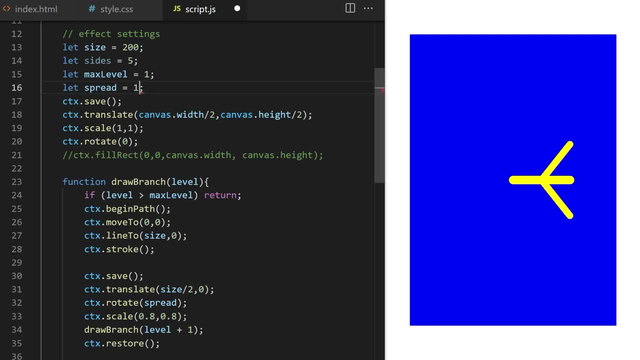 I think this shows really well how secondary branches grow out from the main branch. What if I want to have even more branches growing from the main branch? Let's say I want 2 on each side, so 4 in total. I create a variable I call branches and I set it to 2.. 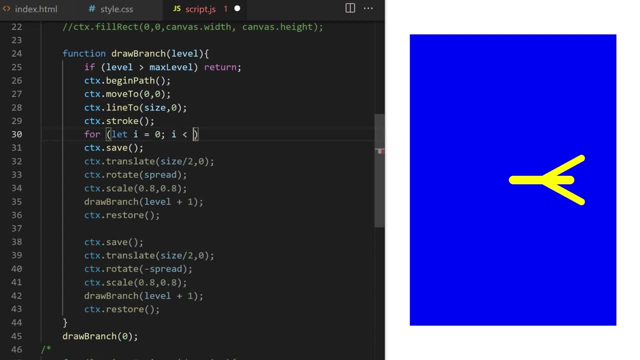 I create a for loop. i is equal to 0.. As long as i is less than branches i++, I put this entire code block here. I create a for loop. i is equal to 0.. As long as i is less than branches i++. 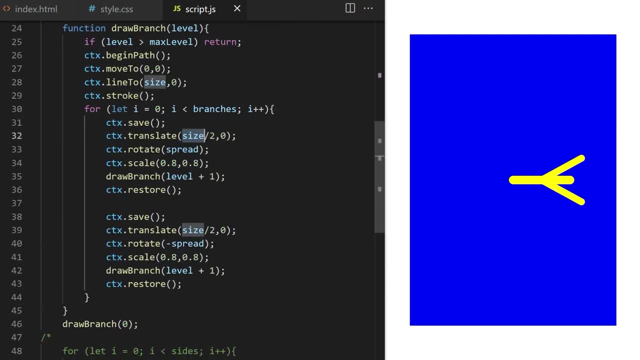 I put this entire code block here. I create a for loop. I create a for loop. I change horizontal value. I pass to translate call: Let's set it to size of the main branch divided by branches variable. we just created times index from the for loop. 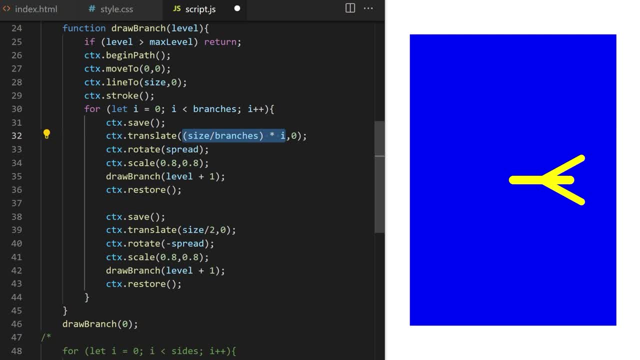 This needs to be in brackets. Let's do the same thing for the opposite segment. Now we have 2 sets of segments growing out from the main parent branch. What if I want them to move along and grow from the other end? I can simply do that by saying size minus size divided by branches, times i. 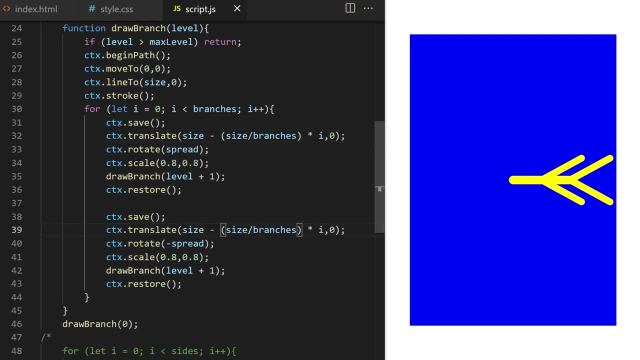 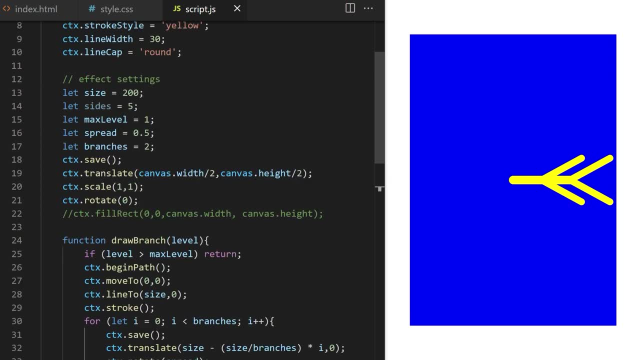 This little formula might not be very clear and intuitive, but if you play with these values for a while, it will become clear how it moves segments along the parent branch. I can change angle here on line 16.. Look at what happens when we set branches to 1,, 2,, 3,, 4, 6.. 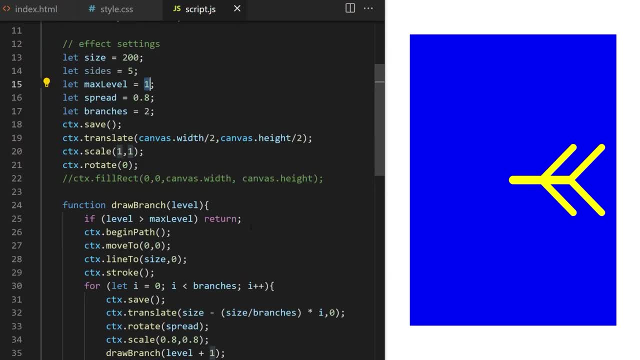 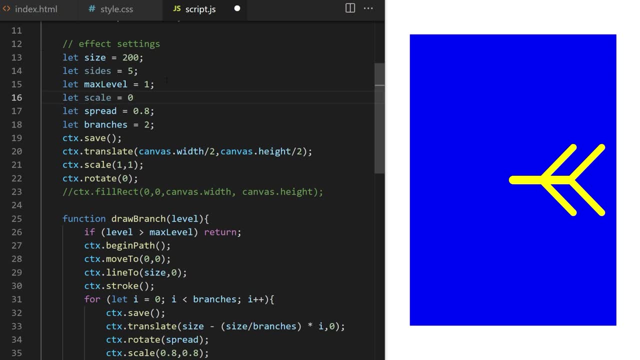 Let's go back to 2.. Look at what max level does. It will give the fractal shape another level of depth. To see it clearly, I need to adjust scale. Let's put the scale value into a variable. I set it to 0.7 initially and I replace all these values we passed to canvas scale method. 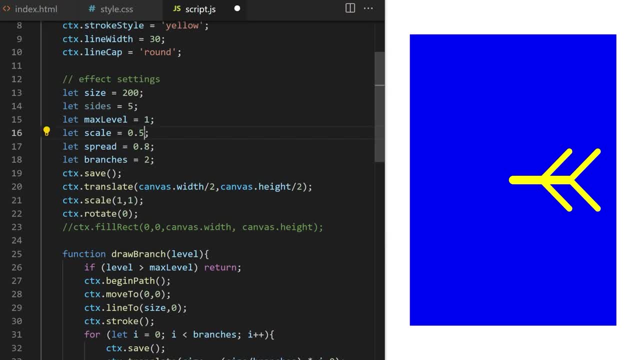 with this new scale variable. Now I can just change the value here. You can see that next set of branches is only 50% scale of the parent branch. If I set max level to 3, each of these small segments will grow its own 4 segments. 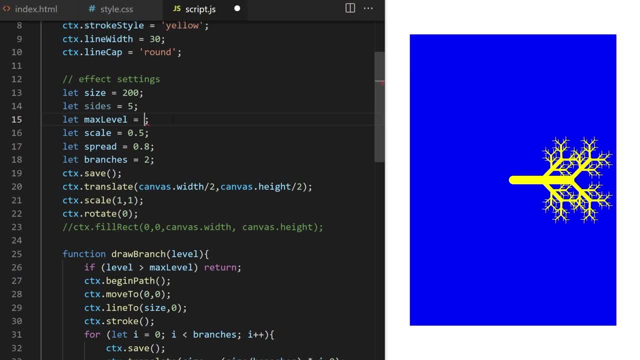 Max level 4 will add another level of depth. I hope you can see what's happening. we have a fractal now. I will set max level to 3 for now If at any point in this course your fractal shapes take too long to render the easiest. 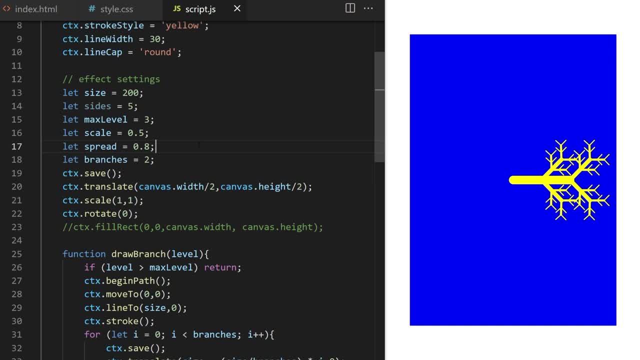 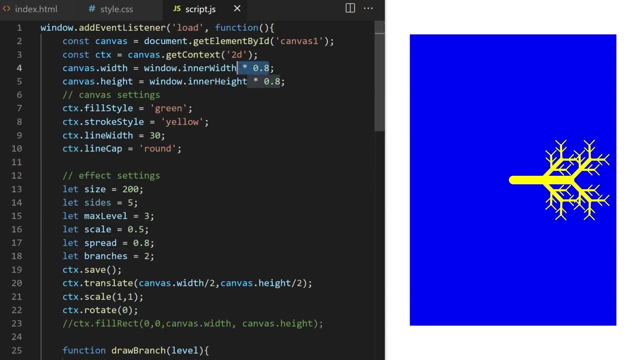 thing to do is to come here to max level variable and set it to a smaller value. Doing that will radically decrease the number of operations needed to draw the fractal shape. I set my canvas to cover full width and height of browser window here. 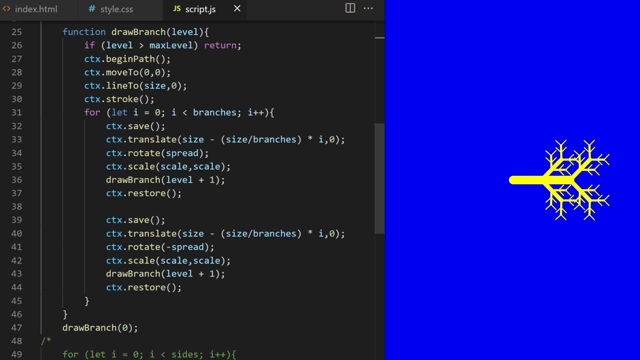 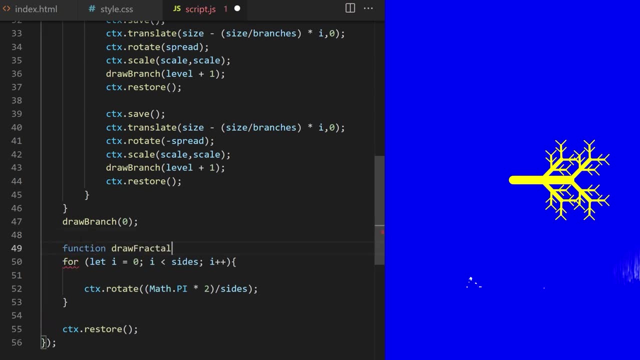 Now we have the code to draw a single branch in our fractal. If I want to make a circular fractal shape, I uncomment this part And I declare another function. I call, for example, drawFractal. I put this for loop inside and I call draw branch from within the for loop. 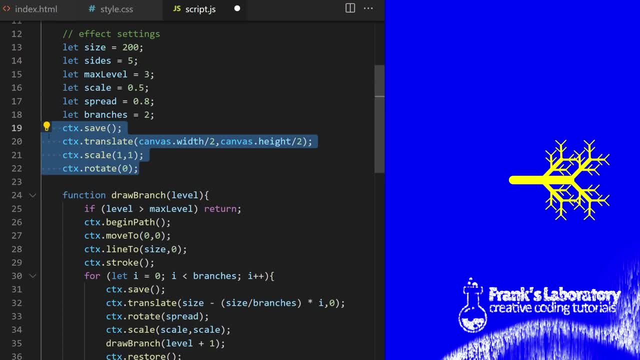 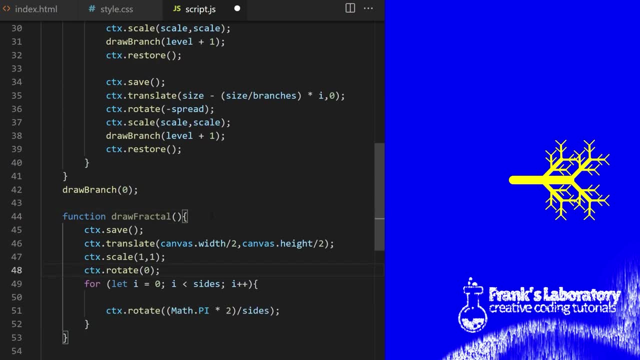 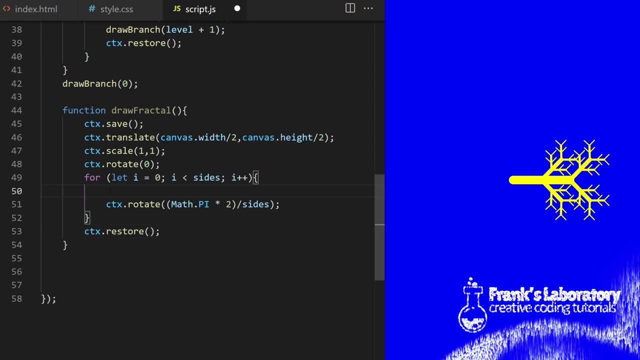 I delete this line. I commented out earlier. I cut safe translate scale and rotate calls from up here and I paste them inside my draw fractal function outside the for loop. I am saving canvas online 45, so I need to put restore inside that function as well. 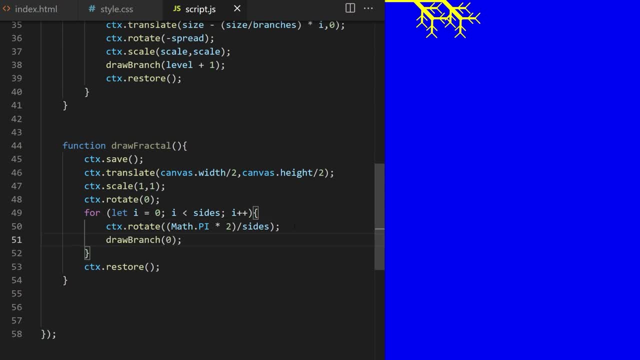 Finally, I take drawBranch call and I put it inside the for loop. I save the canvas on line 45 so I need to put restore inside that function as well. Finally, I take drawBranch call and I put it inside the for loop loop. We have declared custom draw fractal function. let's call it And this: 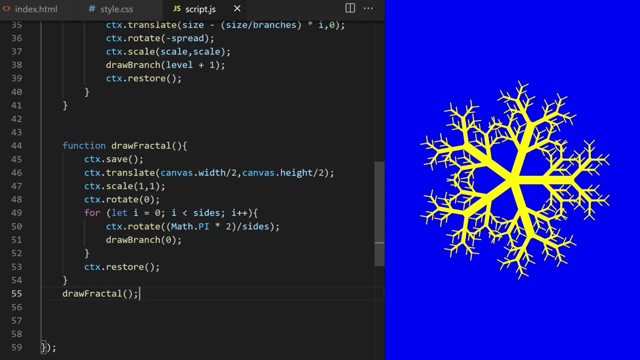 is how you make fractal snowflake. There are many ways we can distort it, randomize it and make it look really cool. Let me show you some of them. Click like if you are getting any value today and if you learn something new, I can. 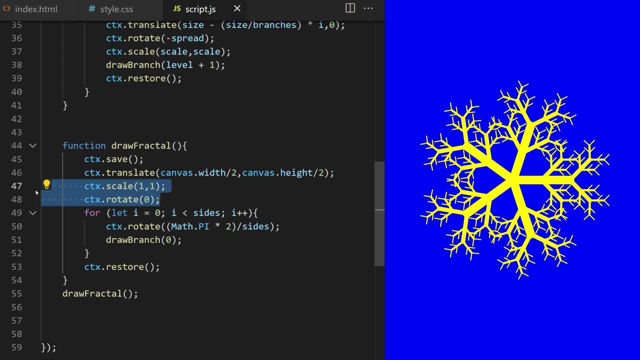 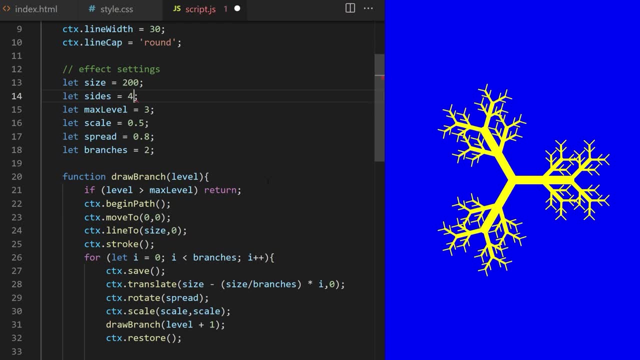 actually remove this scale and rotate as they are set to default values and don't do anything right now. If we change value of size variable, we will get different number of branches that are evenly distributed to form a full circle. Max level determines depth of the fractal. How many times will branches 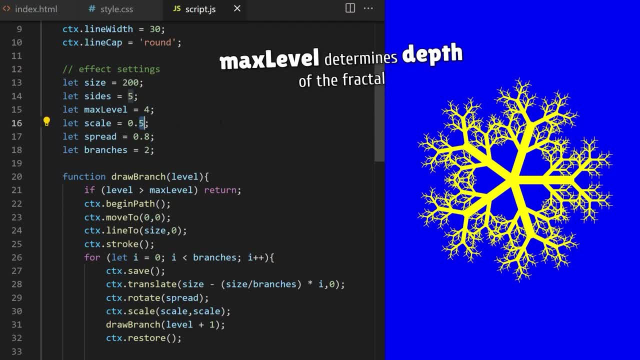 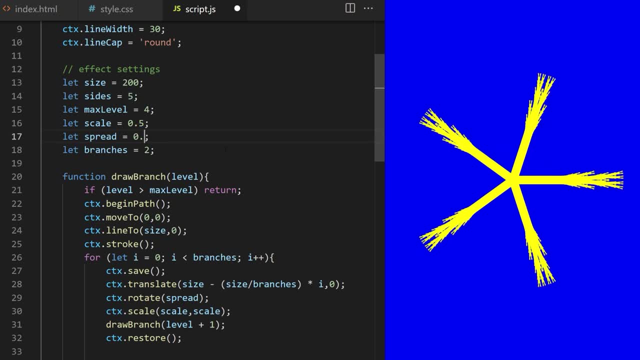 split into smaller segments before fractal shape is finished. Scale determines how much smaller are these segments compared to their parent branch. Spread value is the angle in radiance between parent branches and their segments. I think reasonable range is somewhere between 0.1 radiance and, I guess, 2.9. 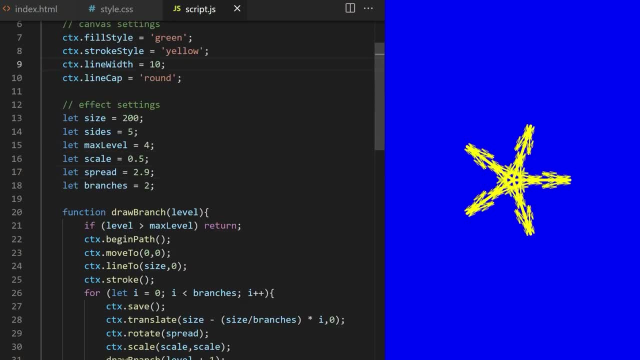 radiance, So almost half a circle. I change line width to 10 pixels so we can see more details in the shape. Spread can be 0.5, for now. I can change stroke style to different colors. I set canvas background to black. Let's give it some shadow If. 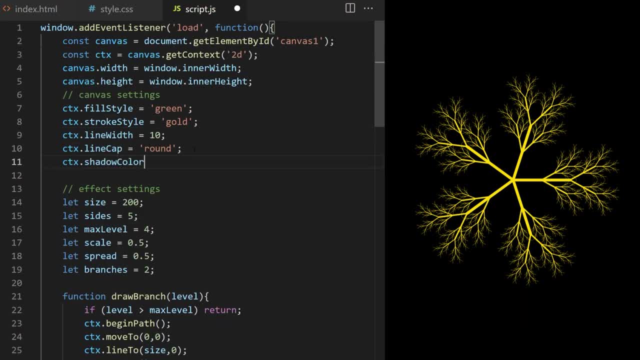 you are using canvas shadows in Firefox or Safari browsers, you might experience minor lag. I hope these browsers catch up soon and start to fully support canvas shadows. It's a feature that's been around for a long time. Shadow would be more visible if background wasn't black, but I still like it that way. I can also. 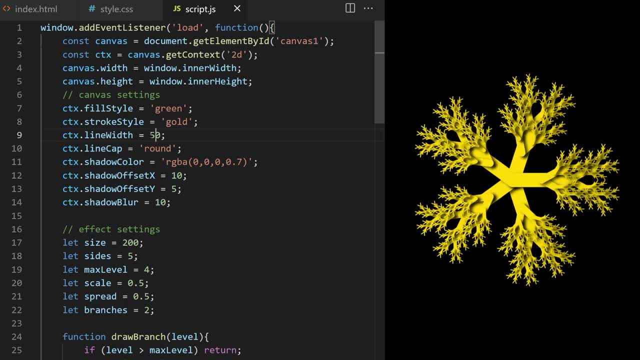 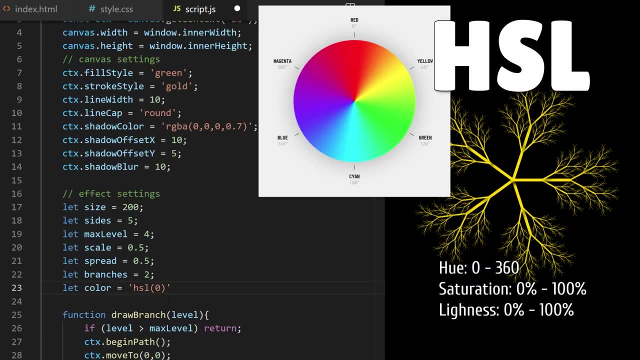 assign colors using HSL color declaration. Hue is angle on color wheel, so value between 0 and 360 will cycle through the entire color spectrum. Saturation: 0% is grayscale. 100% is fully saturated. color Lightness goes from 0 dark to 100% light. 50% is full color, not 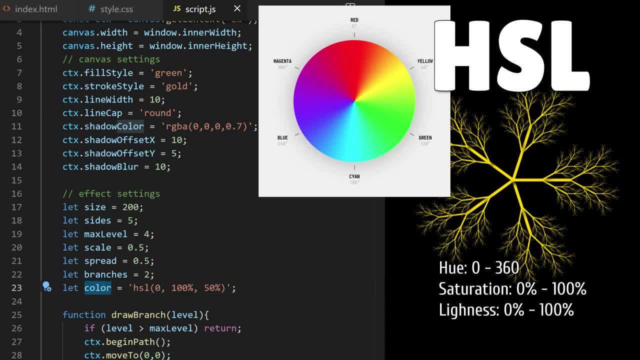 affected by light or dark at all. Angle 0 on HSL color wheel is red color. You can also assign colors using HSL color declaration. You can also assign colors using HSL color. I cut stroke style from line 8 and I pasted inside draw fractal function. I. 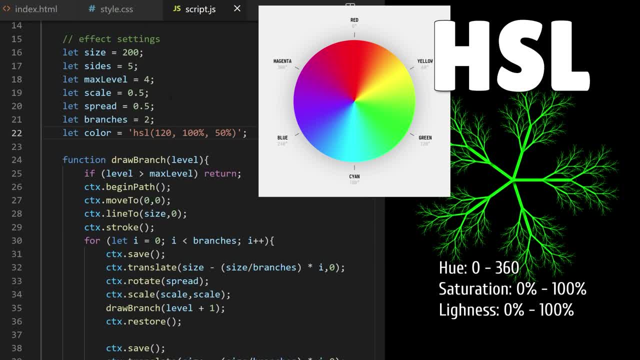 set it to this new color variable. By changing angle value we pass as hue to HSL color declaration. we can cycle through color spectrum. It doesn't even stop at 360 degrees. we can increase it more and more and it will just keep. 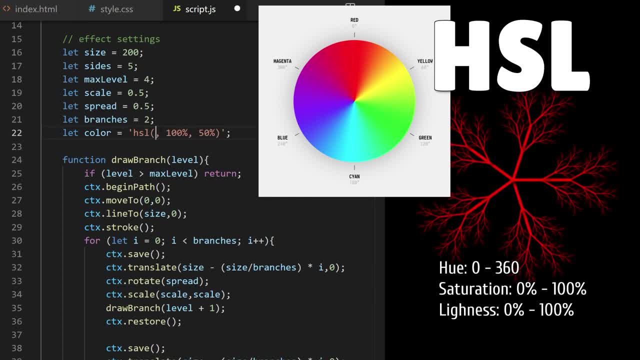 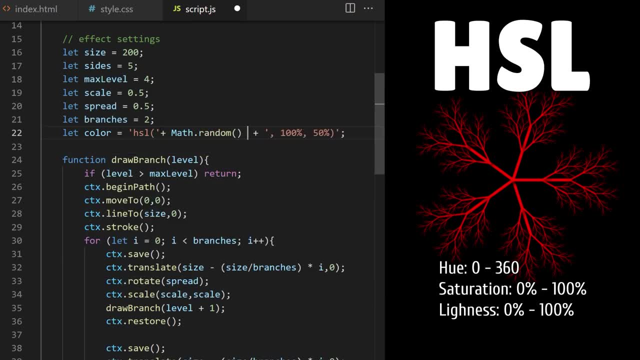 circling around. 0 is red and 360 is red as well because it circled back again. Let's randomize hue value like this On each page: reload: hue will be a random number between 0 and 360 to cover all possible colors. 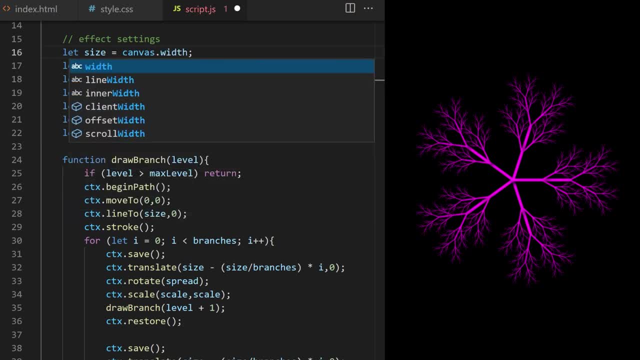 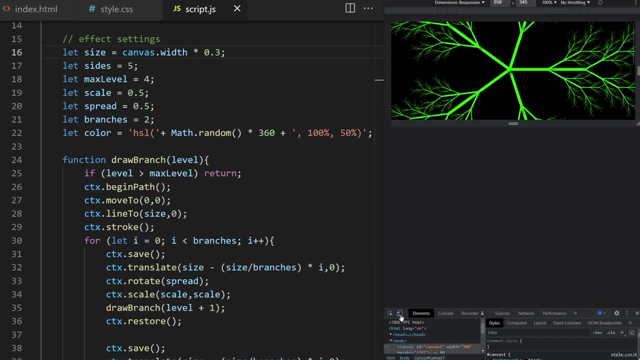 What if I make size of the base branch relative to canvas width so it covers similar portion of canvas on different screen sizes? This works, but if I use my browser developer tools and I flip the screen, it's alright on portrait mode, because that one is restricted by width. 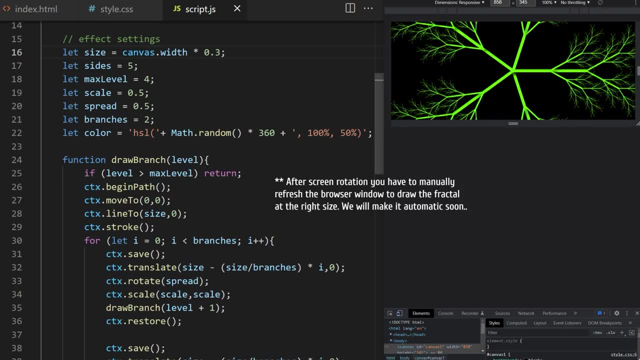 In landscape mode on widescreen the fractal is too big because on this canvas I would like the size to be restricted by height of available canvas area. I always have to refresh page to resize canvas. there is no automatic resizing but we will do that a bit later. 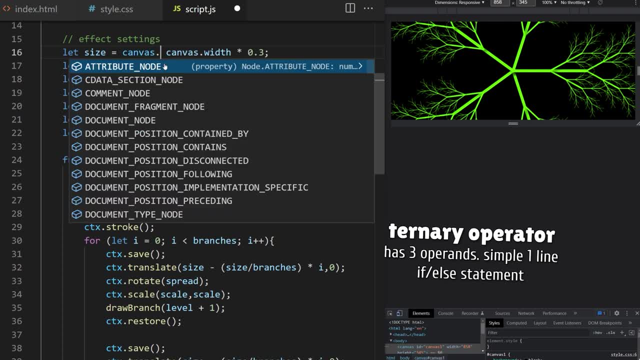 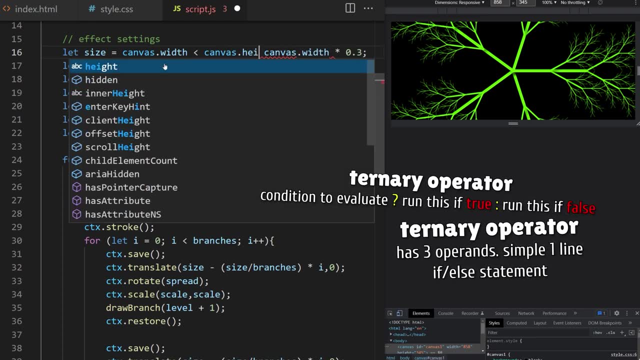 I will use ternary operator, which simply means operator with three operands. In this use case it's just a simple one line. if else statement. If condition is true, question mark: run this code. else colon: run this code. So if canvas width is less than canvas height, 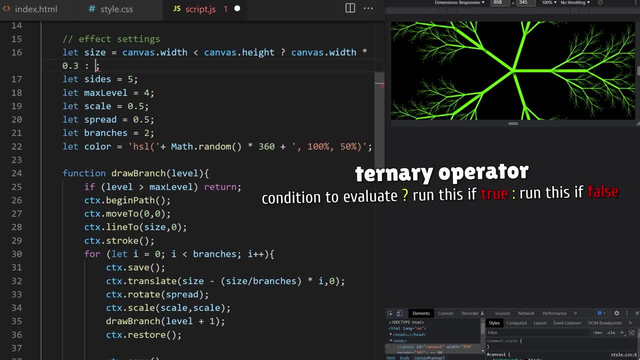 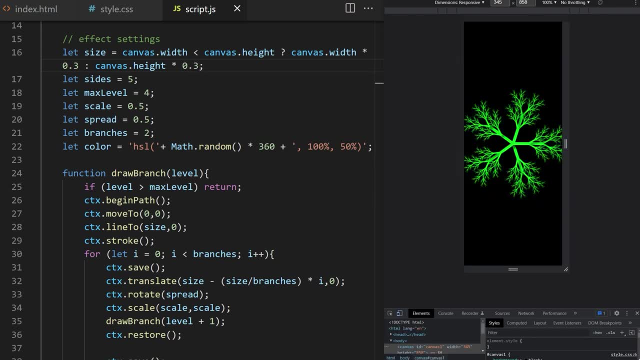 Set the size variable to canvas height: Canvas width times 0.3.. Else, set size to canvas height times 0.3.. Now the size of our fractal will be restricted by either width or height of canvas, depending on which one is smaller. 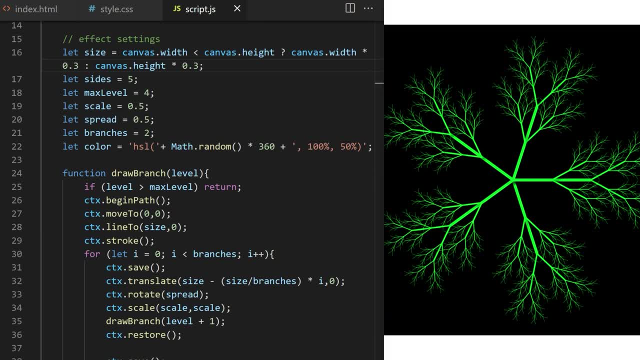 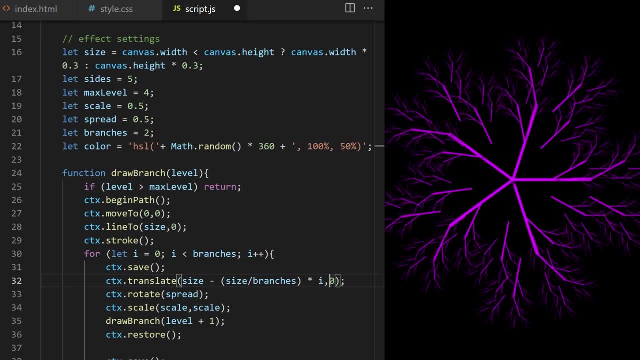 This means we can always see the entire fractal shape on wide and on tall screens. I can distort fractal shape in many different ways, For example by translating it to a different vertical y coordinate. here Let's give the effect. some buttons and sliders. 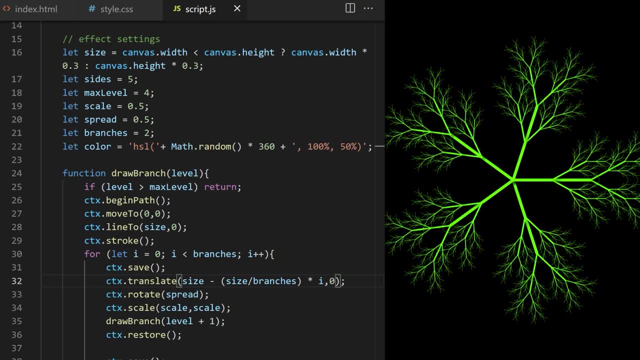 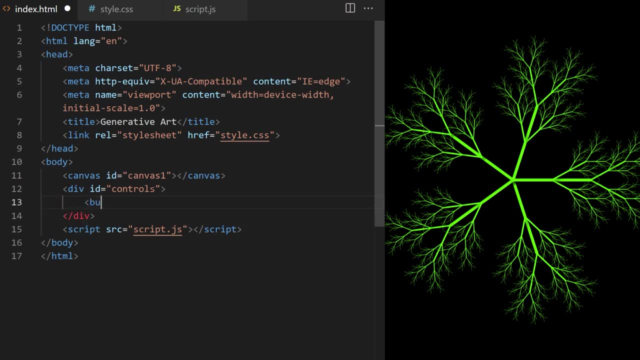 So that we can change it and randomize it from a browser window rather than by manually changing code. I create a div with an id of controls Button, element with an id of randomize button and text randomize. We can't see it because canvas has position absolute, so it's on top of it. 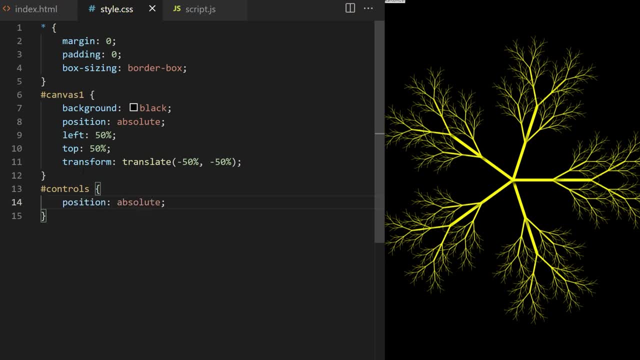 If I set controls to position absolute as well, now it's visible. Padding: 10 pixels. Border: 2 pixels. solid white. Left: 20 pixels. Top, 20 pixels. Width will be 250 pixels. Background: semi-transparent white color. I give buttons some padding. 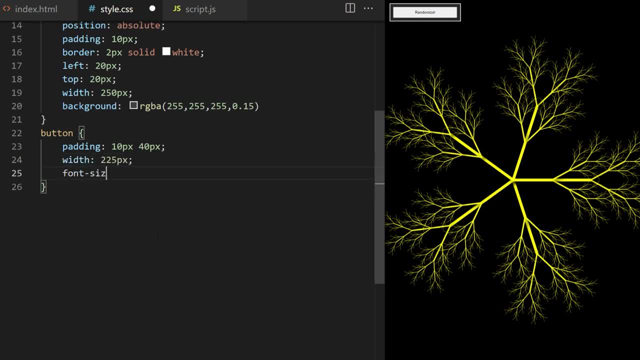 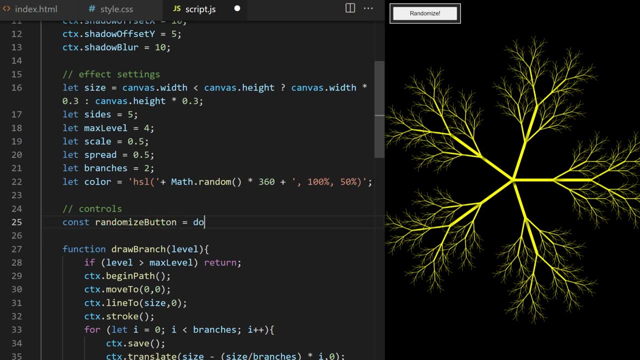 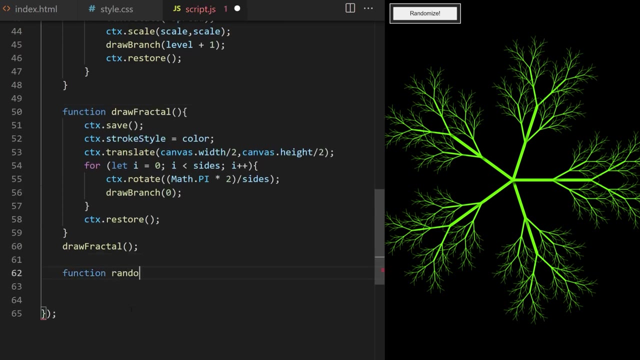 Width will be 225 pixels. Font size: 20 pixels. Let's create an area in script file for controls. I bring my randomize button into the project. I create a custom function. I call, for example, randomize fractal. Whenever this function runs, some of the effect settings will be randomized to a different. 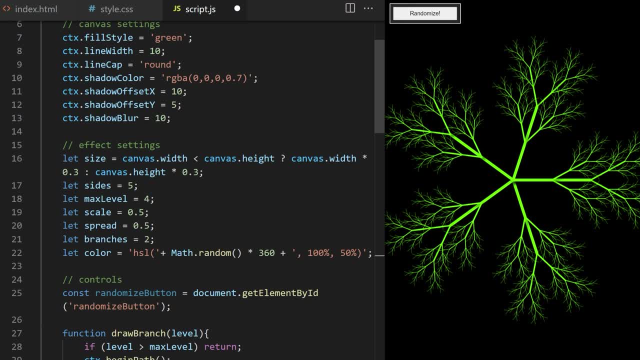 value change in shape of the fractal. Some of these settings I don't want to be randomized. For example, I want max level to stay the same, so I set it to const. Remember that if it takes too long to render fractal shapes on your computers, the easiest 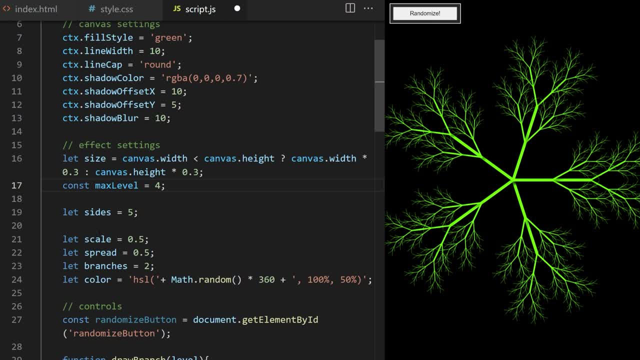 fixed is to come here and set max level to 3.. This will decrease the depth of fractal by one level and it will massively reduce the number of calculations And draw calls needed to create the final shape. I also want two branches per segment, so this will also be const. 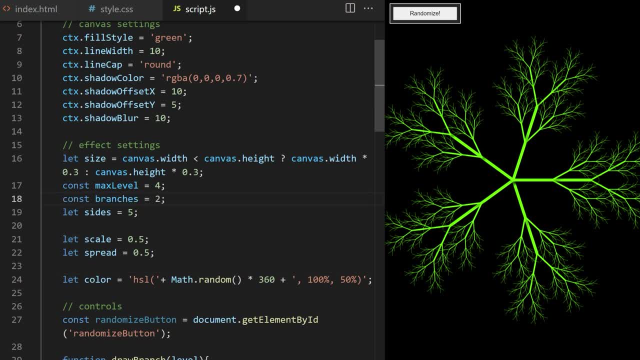 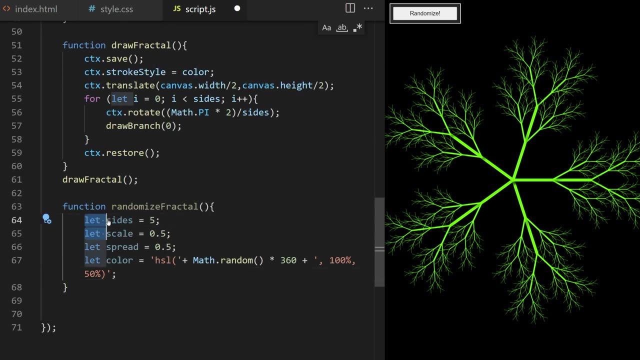 You can experiment with different values here to see what happens. Try 1 or 3.. You might get some interesting unique shapes. These remaining 4 values will stay as let variables and we will randomize them each time randomized button is pressed. So let's copy them and delete let keywords, because we are not declaring new variables. 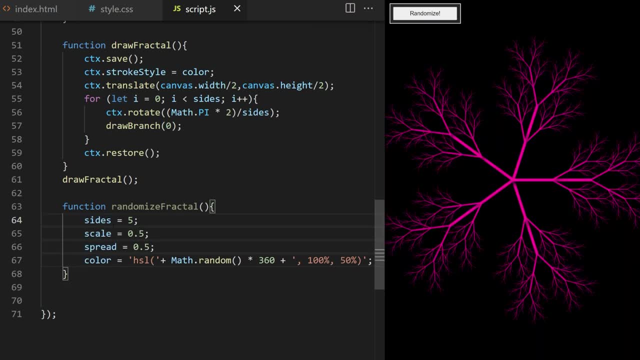 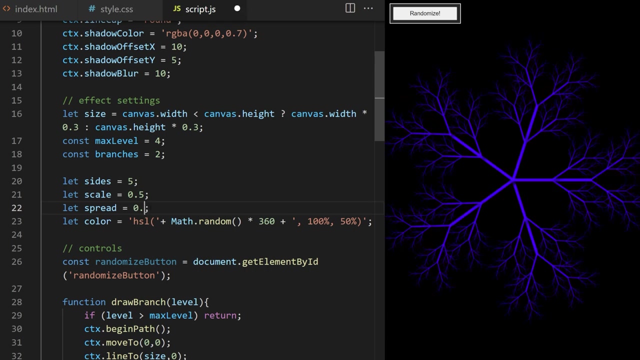 We are reassigning values to existing variables here. Sides could be a random number between 2 and 9, for example. Scale will be random value between 0.4 and 0.6.. Spread angle will be- hmmm, I guess we start from this shape, so 0.1 and we go all the way. 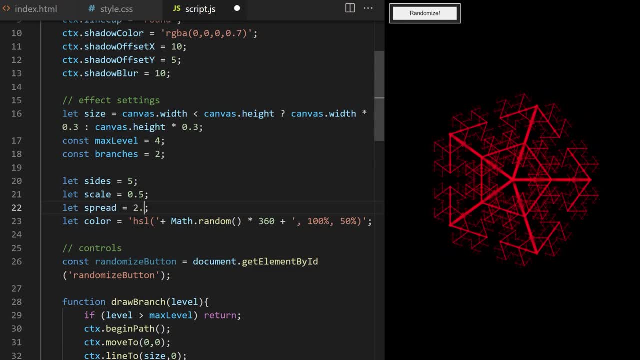 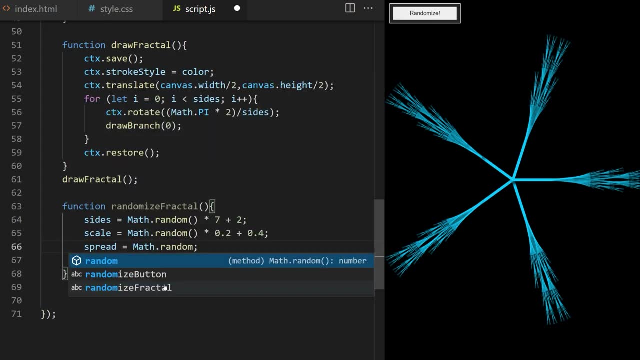 to until the branches rotate almost half circle around, which is around 3 radians, Almost 180 degrees, but not quite. Spread will be a random number between 0.1 and 3.. Color is already randomized. since we are using mathrandom on hue argument, we pass. 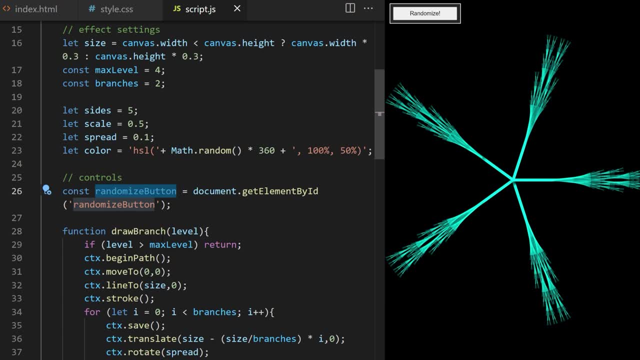 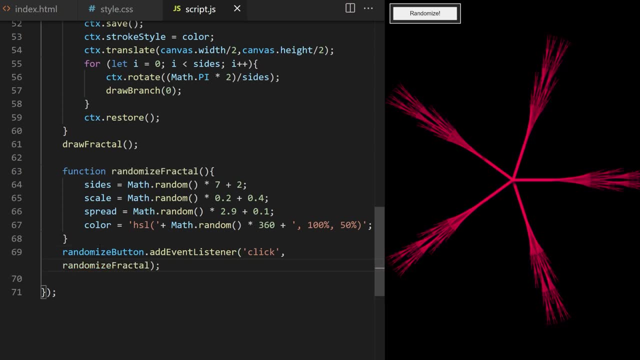 to HSL color declaration. I take randomize button and I add event listener to it. We will listen for click event and we will run randomize fractal function. After we randomize fractal, we also need to draw the new one with updated values. 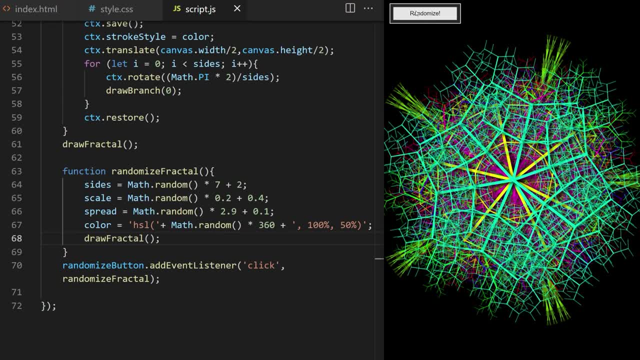 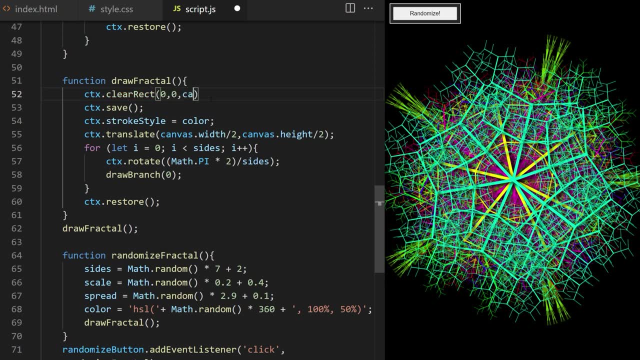 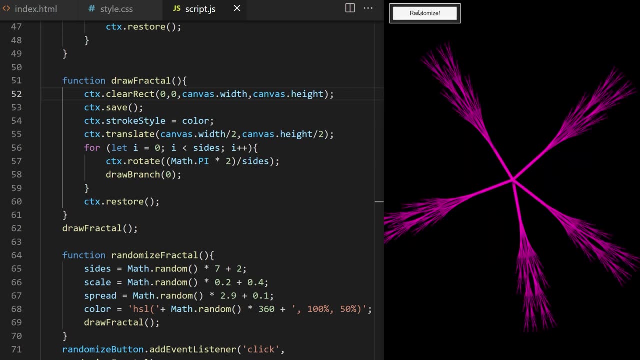 Nice, this works. I also have to delete canvas every time I generate new fractal. so I call built in clear rectangle method And I clear the entire canvas. I will add new coordinate 00 to canvas width. canvas height. You can see there is one branch here that is off. 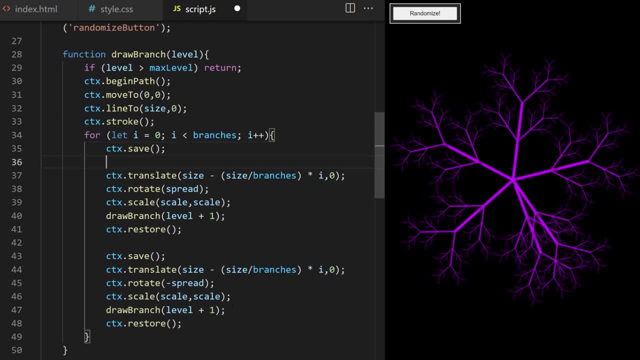 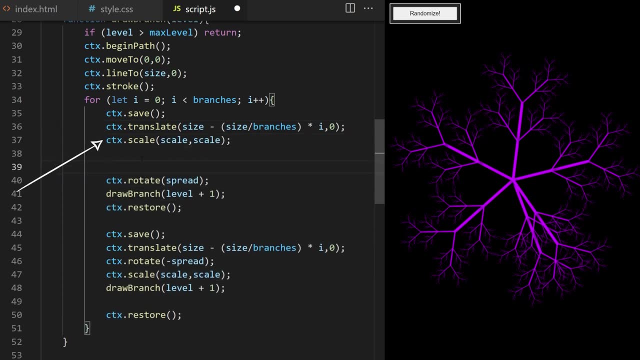 Hmm, strange. Let's see what I did. Is it because I am not doing save and restore here correctly? Well, I can see that I can put translate and scale here and I call save here. I can delete this translate and this scale because now, by adding that additional save, 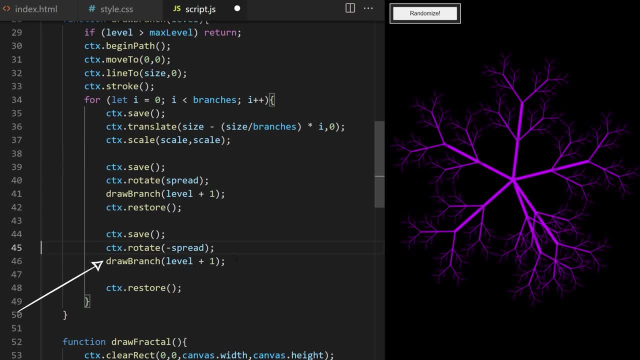 this translate and scale will still have effect on this. I can delete this translate and this scale because now, by adding that additional save, this translate and scale will still have effect on this scale. I can delete this translate and this scale will still have effect on this scale and I. 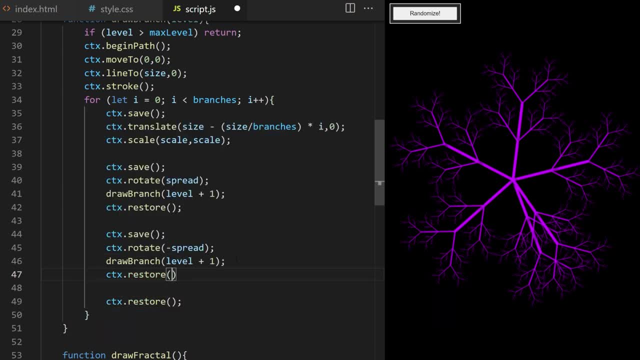 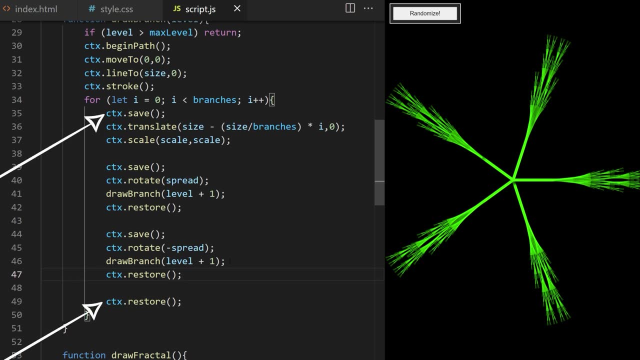 can delete this translate and this scale will still have effect on this scale. I am just playing with this. bear with me a second please. Now it needs to restore again here, So we have this outer save and restore and then we have these two pairs of save and restore. 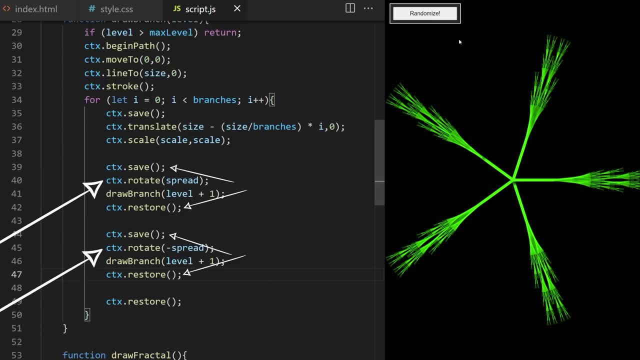 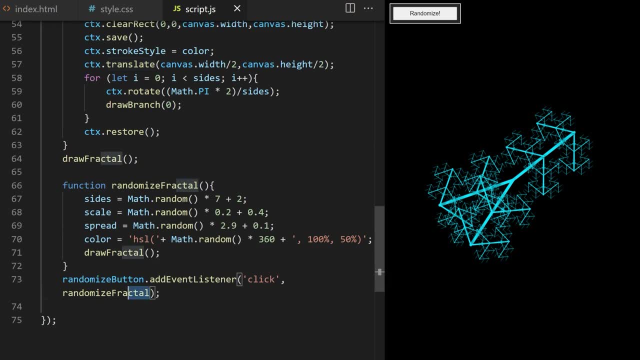 for each branch to separate positive and negative rotate from each other. I prefer this code, but I am still getting the off branch, so this wasn't a problem. Let's actually turn this into call back function, because I will have to do that for sliders soon anyway. 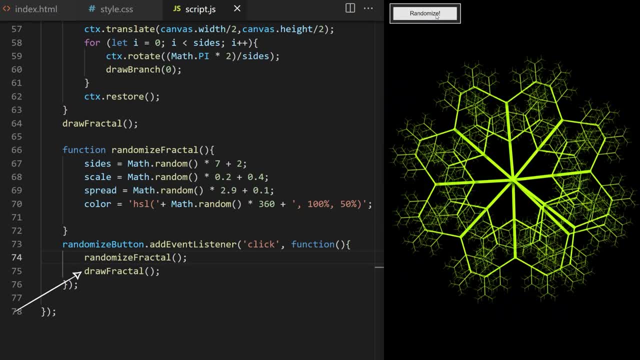 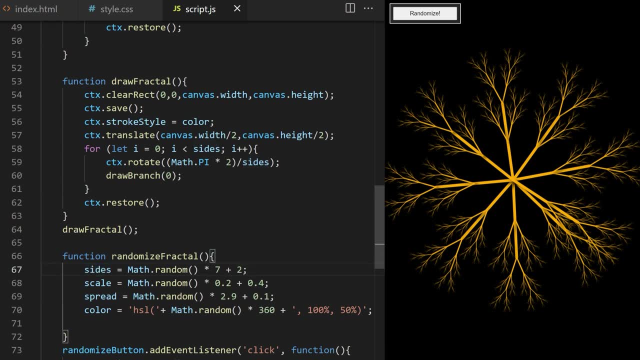 is clicked, we call randomize fractal and draw fractal. and now I can finally see what the problem was. some of you probably already realized it. number of sites needs to be an integer number without decimal points. here I'm randomizing and getting values like 8.3, so my fractal has 8.3 sites. let's wrap it. 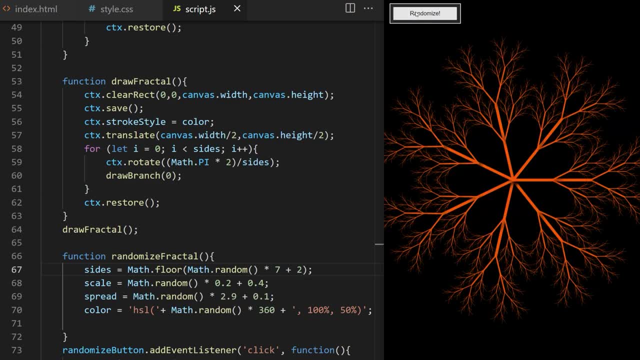 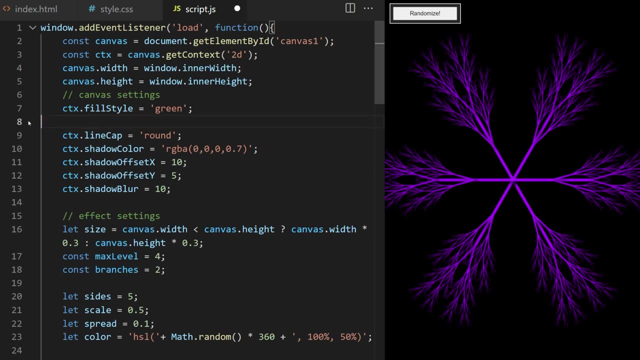 in mathfloor so that we get even slices of a circle. we are randomizing our fractal. this is really good, but it can be so much better. let's also randomize line width. I cut it here and I paste it inside draw fractal. it will be equal to. 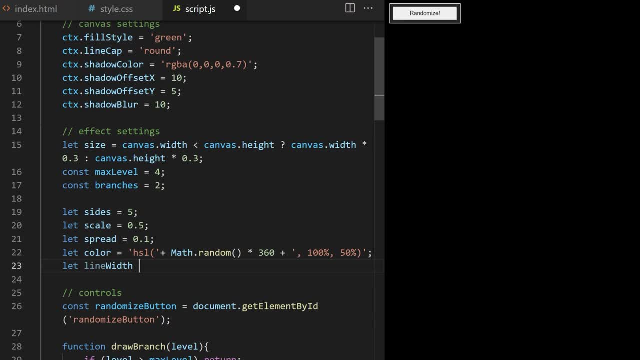 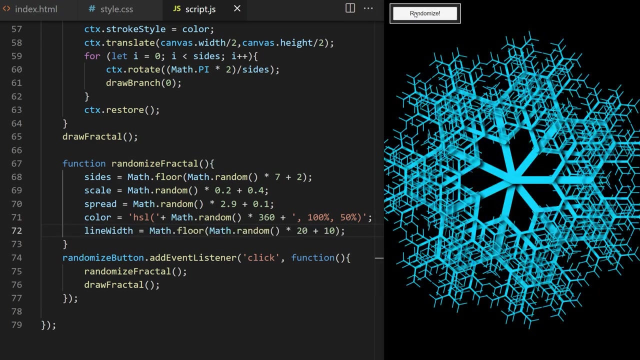 line width variable. I need to declare it here in effect settings and I set it to random number between 10 and 20, and I also randomize it every time we call randomizeFractal function. we are getting some really cool unique fractal shapes every time we press randomize. 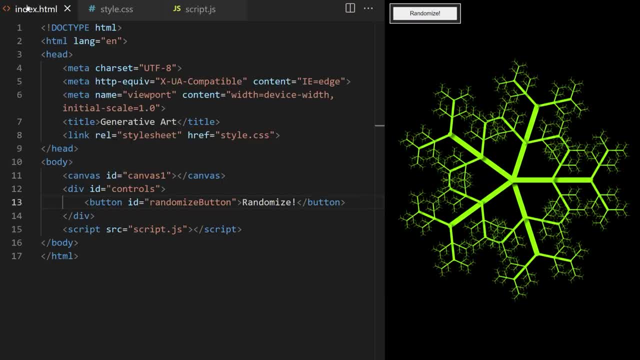 button. let's create a slider in index HTML. I create a div Inside. we will have input element with id of spread type range: min value 0.1,. max value 3.1,. the amount by which the value changes for each step will be 0.02, for example, The: 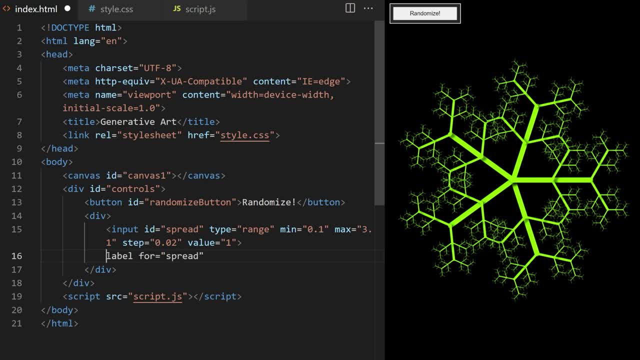 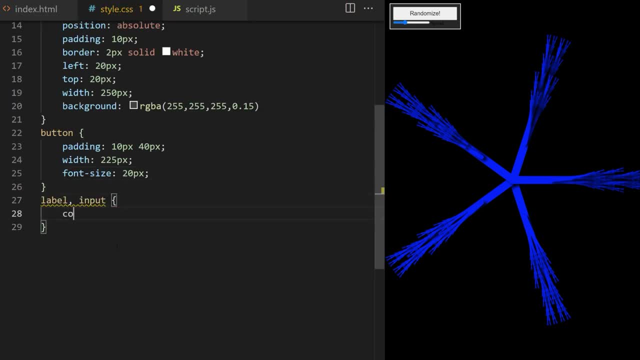 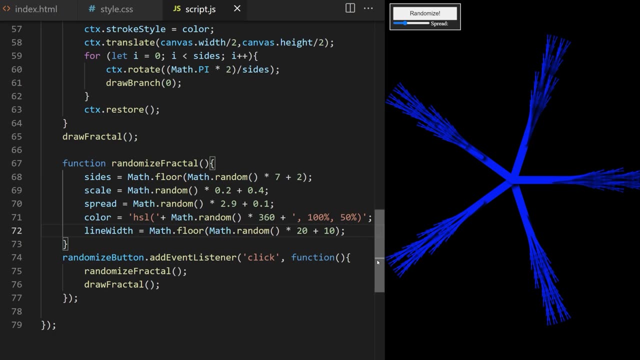 initial value will be 1.. I also create a label for this spread input element. In CSS. I take label and input and I set text color to white and font size to 15px- 20px. I bring the slider into my JavaScript file. I call it, for example: slider- underscore- spread. I also need a variable. 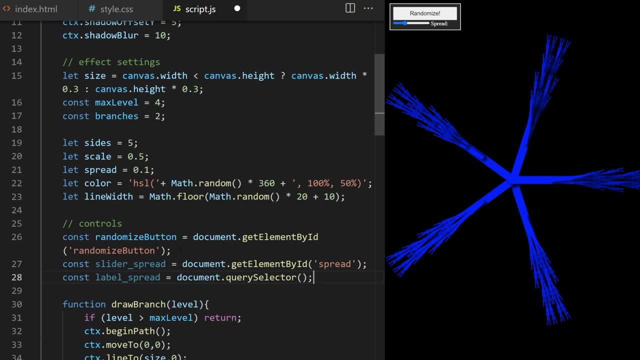 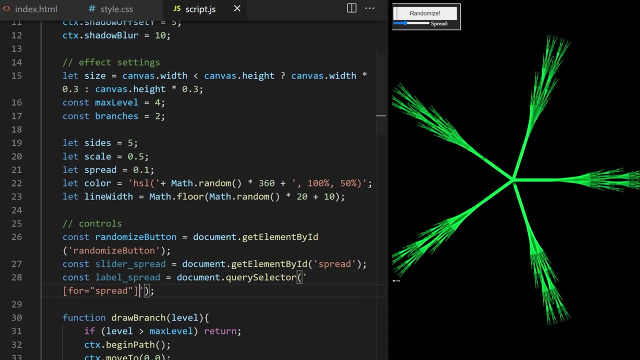 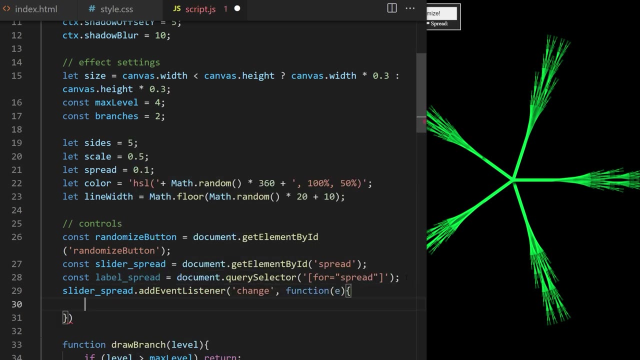 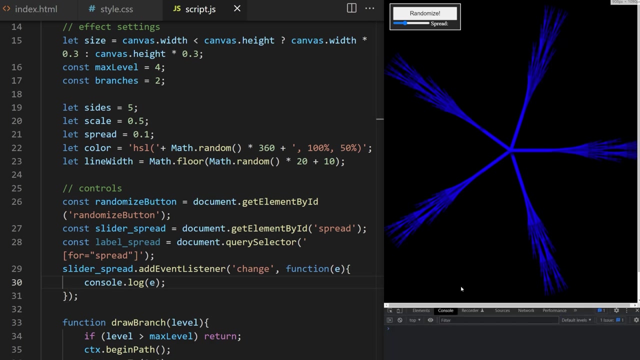 for label. We can target label element using its for attribute like this: Now I can give the slider an event listener for change. event Event listener has access to this built-in auto-generated event object. I will assign it a variable name, for example e. If I interact with the slider now, it console logs this change. 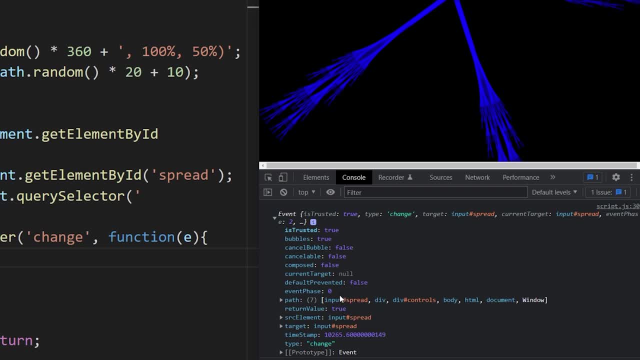 event. There is lot of information about the event in here. What I am interested in is this target object, which means target of the event, in our case the input slider. Inside we have value property which holds the current value. this slider was set to Notice that. 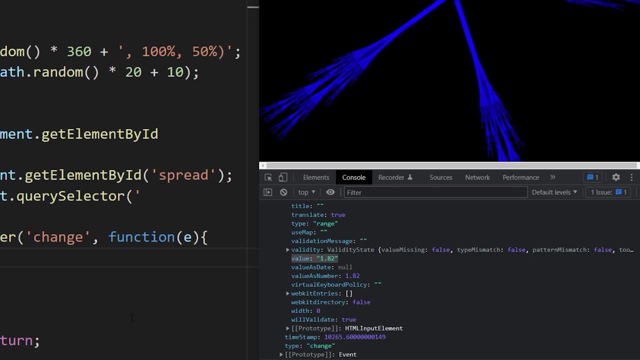 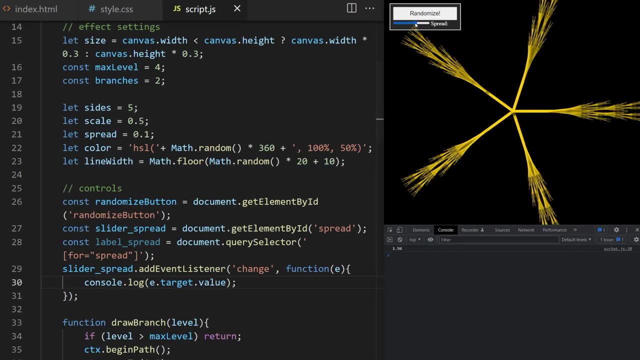 data type of this value is not a number, It is a string, So JavaScript considers this number to be a line of text. It will be important in a minute. Now, when I move slider around, I am triggering its change event and its console login current. 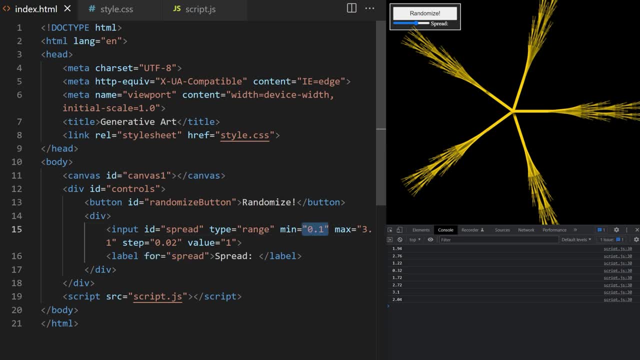 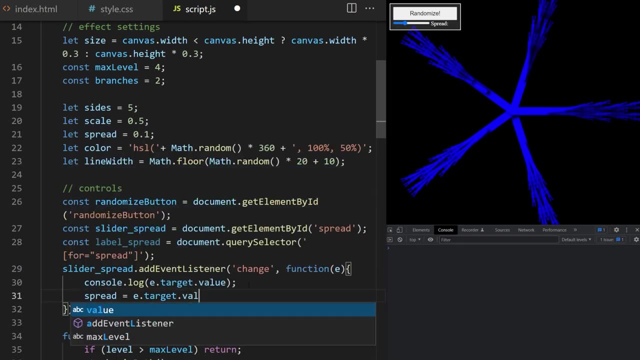 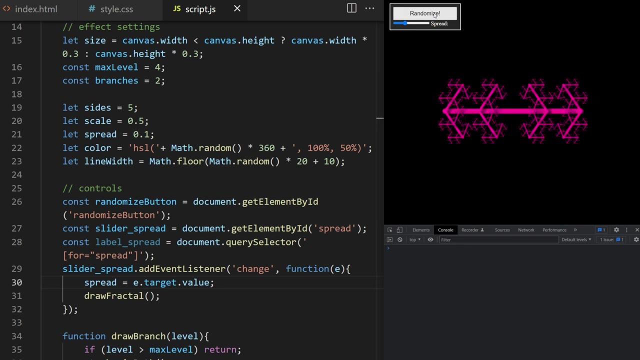 value of that slider. That value is anything between this min and this max range. I can take that new value and assign it to spread variable And once spread is updated I redraw the entire fractal. with these new settings You can see how fractal reacts when I change that angle. Let's make it move in bigger steps. 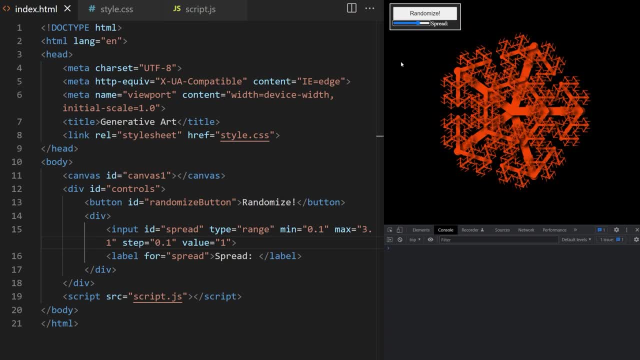 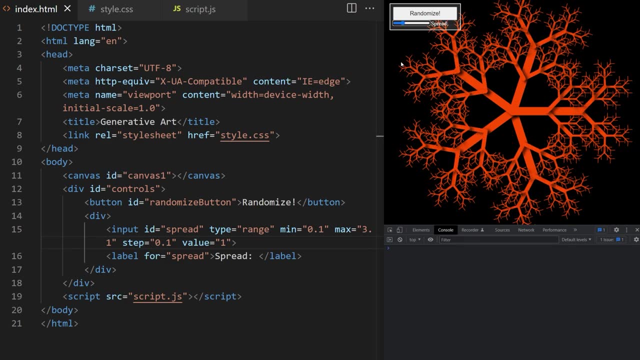 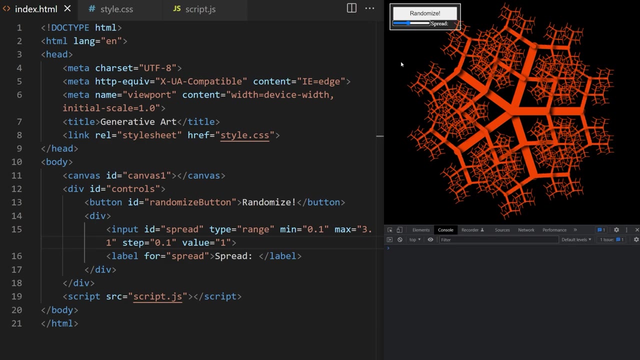 Maybe one step will be 0.1 radians. I think this makes it very clear how spread value, which is the angle at which the new set of branches grows from its associated parent branch, how it affects the entire fractal shape. I like what's happening when I change it step by step. like this Might be a good idea to. 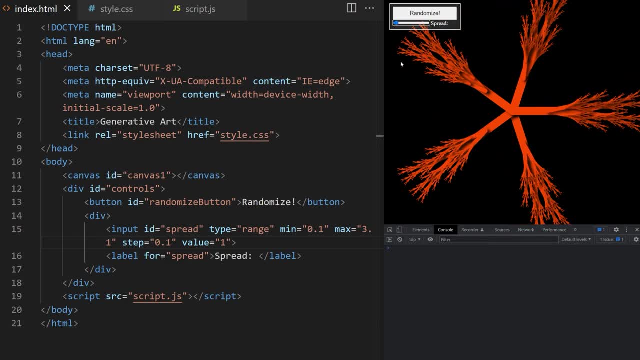 connect it to an automated animation and have the fractal transform on its own. You will notice that when I click randomize button, all the values are changing, including the angle value in spread variable, But the spread slider doesn't react. What if I wanted? 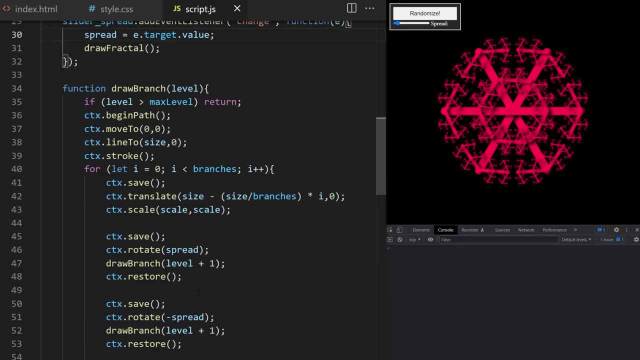 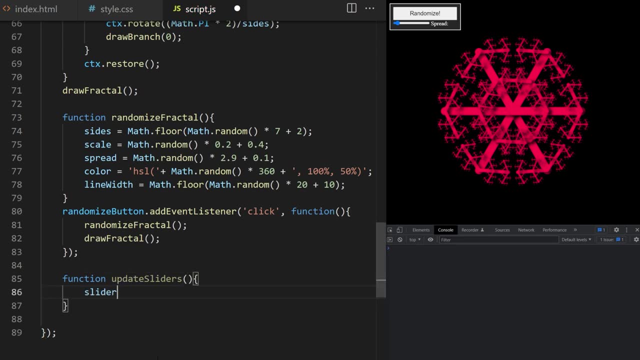 to work both ways and I wanted to always update as we click randomize, I create a custom function. I call, for example, update sliders Inside. I take slider spread and I set its value to the current value of my value. I set the value 0.1 radians and I set the value of my value. 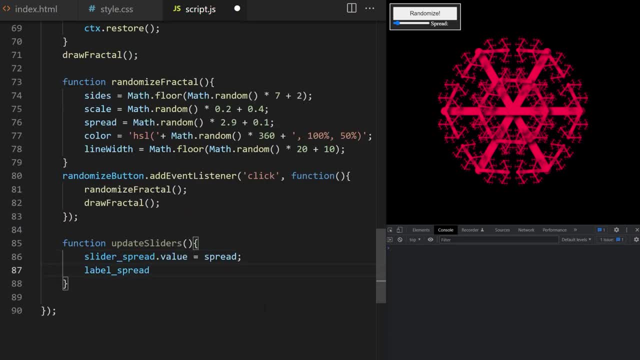 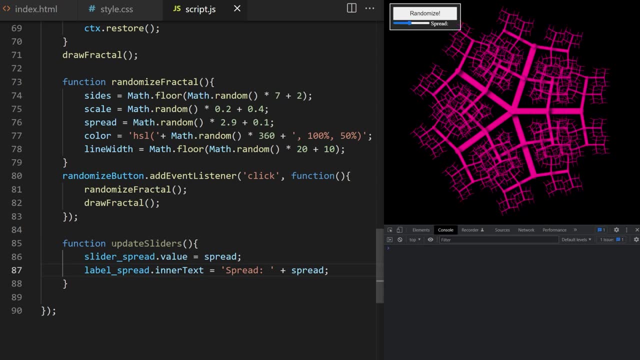 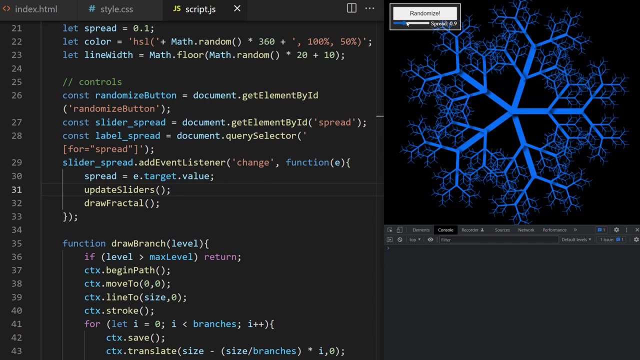 of spread variable. I also take label and I set its inner text property to spread colon space plus the value of spread variable like this: Now I can take this new function and call it every time spread slider changes value. You can see that it works and label is updating. I want the same thing to happen when we click. 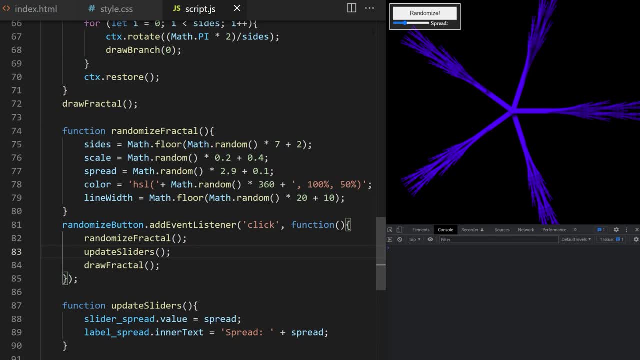 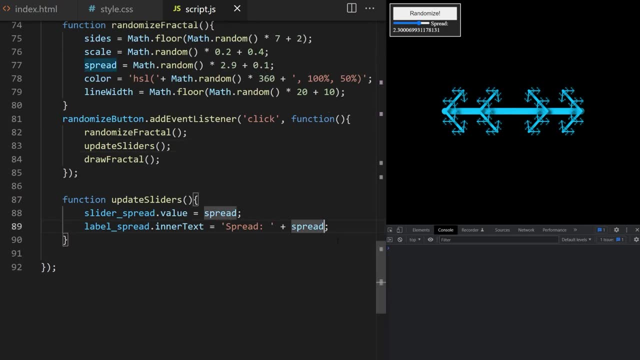 randomize button, so I put it in here. It does work, but we are getting many digits after the decimal point. as that value is being randomized, I can use built-in JavaScript to fixed method. This can be called on any variable that holds a number type and it will. 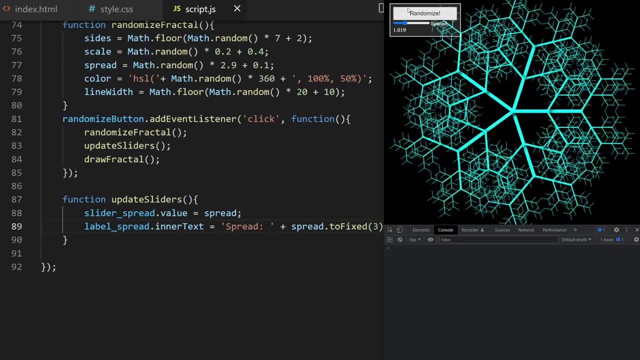 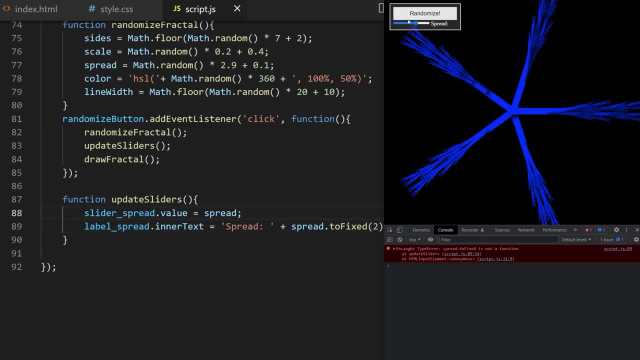 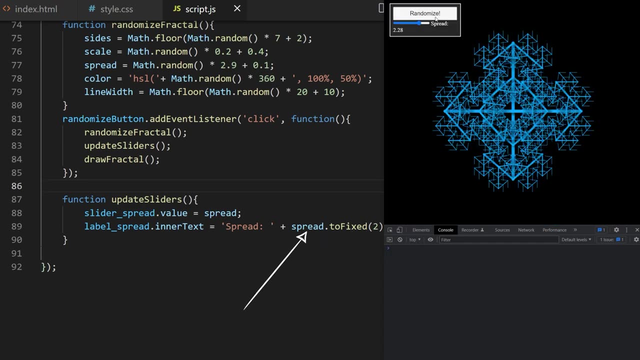 format a number using fixed point notation. Let's say I want to have only three decimal points. That works, maybe just two. When I change input slider I get an error. The reason for that is that as I call update sliders, I'm trying to call to fixed method on a value coming from that slider. 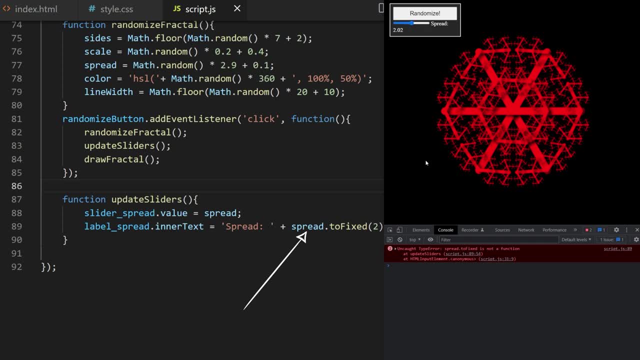 And, as we said before, that value is not number type, it is a string text type. So we get a type error. We can easily fix that by using number constructor. It will take that string value coming from slider and it will convert it to a number type. I need to make sure I 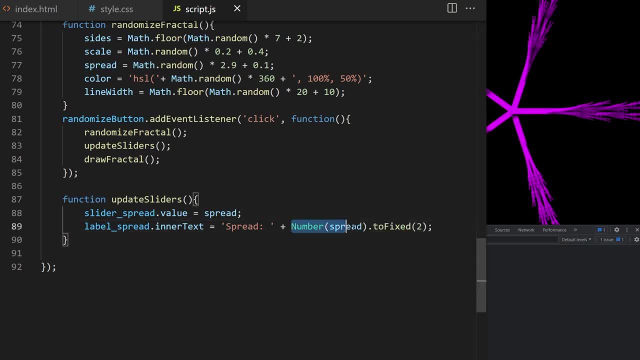 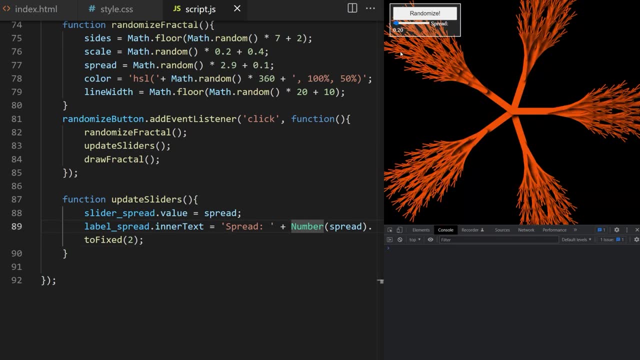 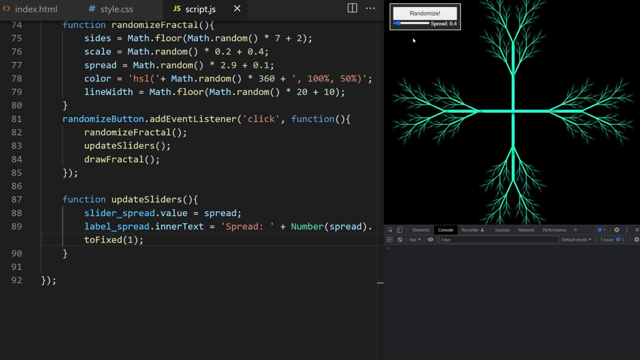 do the brackets correctly, Like this: Now I can click randomize and I can interact with the slider. Both actions will correctly update, label and slider when needed. Maybe it's enough just to give it one decimal point. So this is a very simple way to add sliders to your project. I'm using procedural programming. 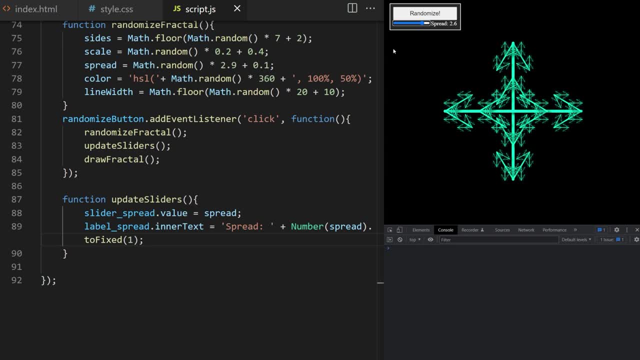 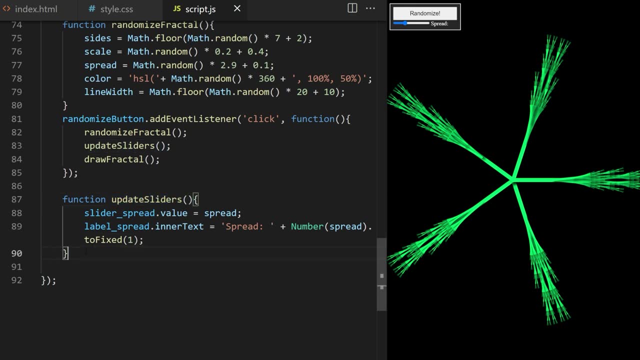 paradigm to keep the code simple. today I'm pulling global variables into my functions, but I think for clarity and for learning purposes, this is fine. I will also call update sliders on the first page load so that slider values and labels are always correct even before we start interacting with controls. 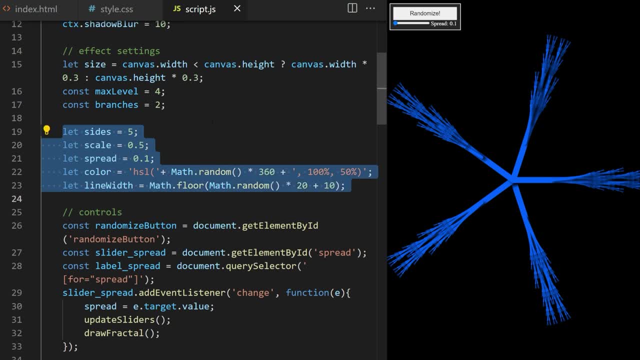 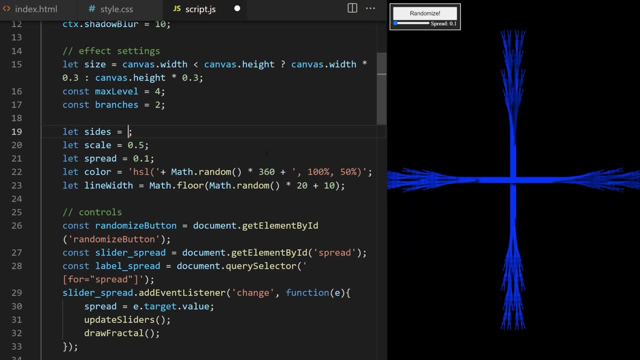 We can create sliders for any of these settings we assigned to let variables. We can also change max level and branches. But both of these settings will rapidly increase the number of draw calls and calculations needed to render the final fractal shape With this particular project. it's ok to have some render time. These complex fractal shapes. 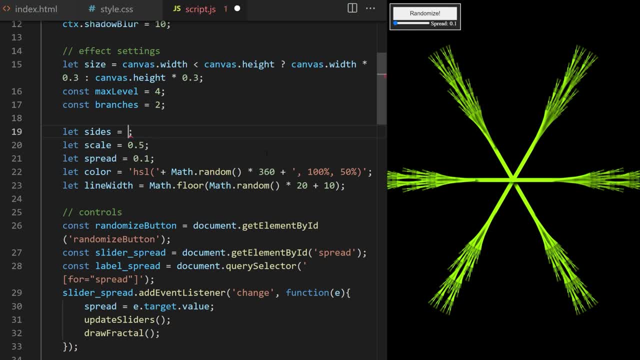 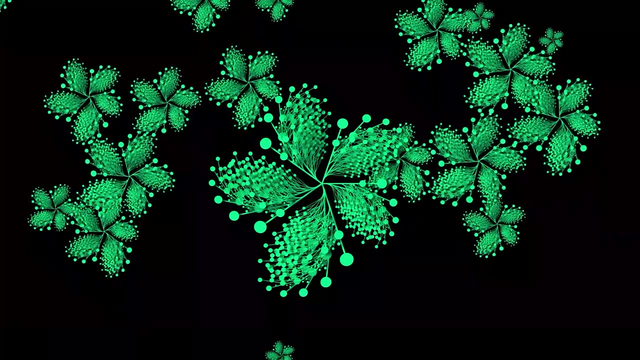 are not meant to be drawn instantly. It's ok that there is some wait time. My computer is very strong and still it takes some time to render more complex shapes. That being said, there is a way to do effects like this. Normally, on canvas, we draw everything. 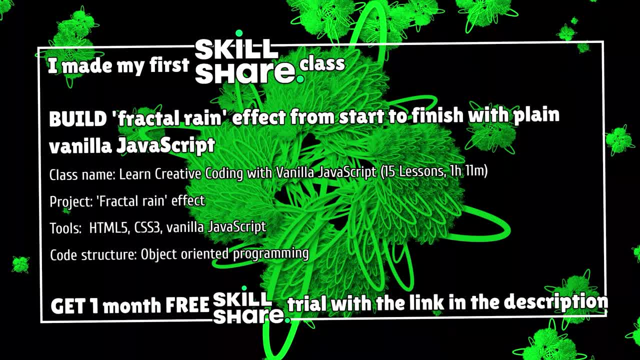 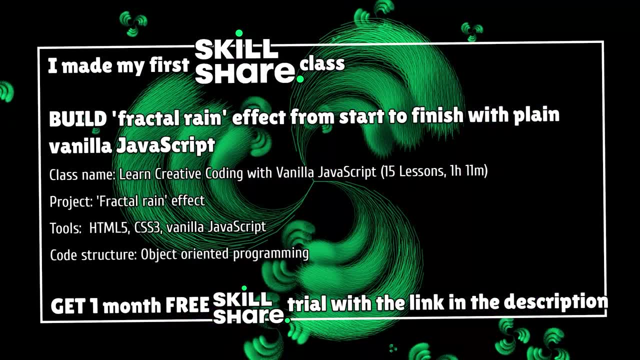 delete the entire canvas, Update positions and redraw everything. Add these updated positions. This cannot be done with complex fractal shapes. It's not possible to simply draw all these shapes 60 times per second. That would be a lot of operations. But there is an easy trick to do that, using 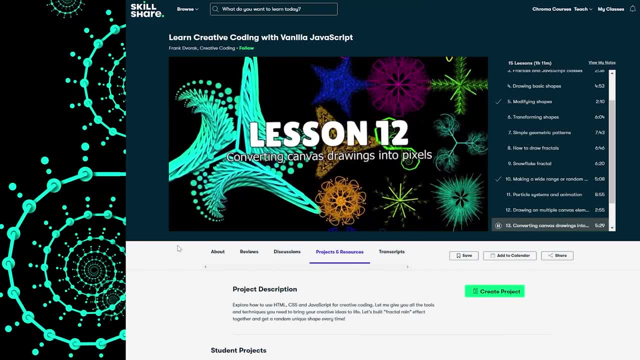 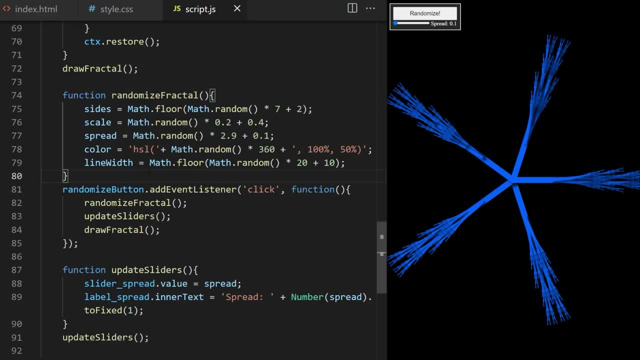 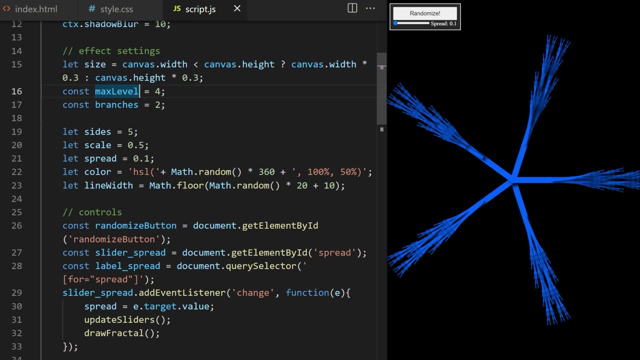 built-in javascript 2 data URL method. I explain exactly how to do that step by step in my first Skillshare course Link in the video description. If you want your fractals to render faster, decrease the value of maxLevel. If you want more elaborate, complex shapes, increase these values, but do it slowly, Don't. 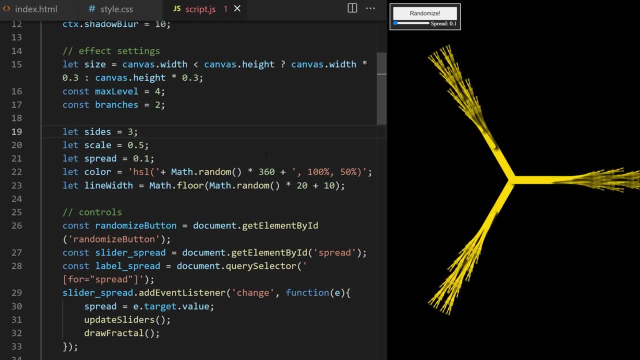 set these to very high values. We also have this sides property which determines how many branches we will get. These branches will always be evenly split in a circle area, Doesn't matter if we have 3 sides or 20 sides. Let's do one more slider for sides. 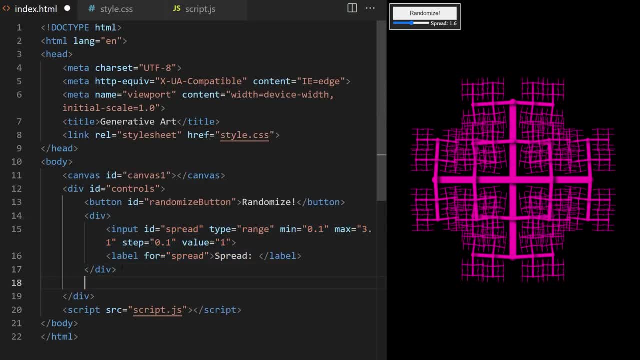 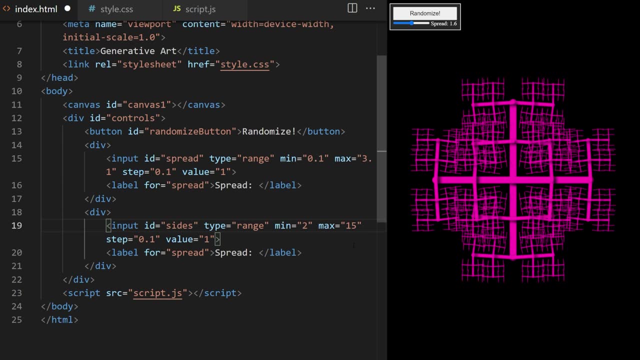 We will just repeat steps we did for spread slider. I copy and adjust this code. block Id is sides. Minimum value is 2.. Maximum value is 15.. The number of sides will also affect render time, but not as much as maxLevel or branches. property Step will be 1 and initial value 5.. 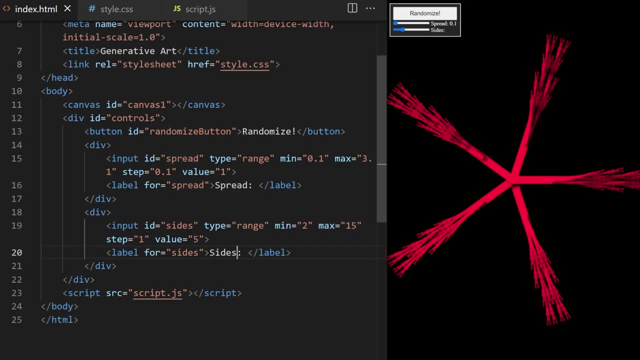 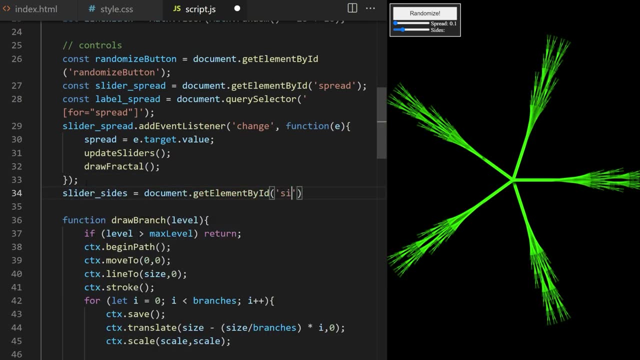 Label for sides will say sides, colon space. I bring it into my javascript file. I will call it slider underscore sides and label underscore sides, And that's it. Thanks for watching. I attach event listener to the slider and on change event we set sides property to the 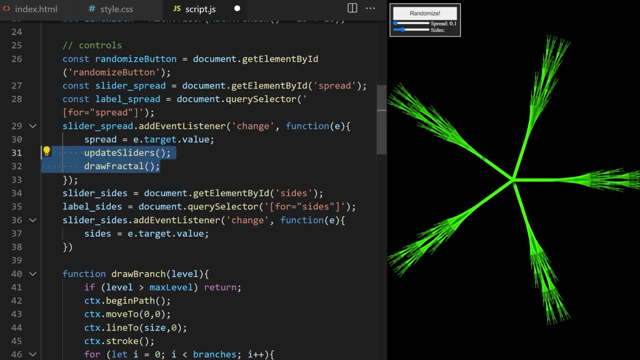 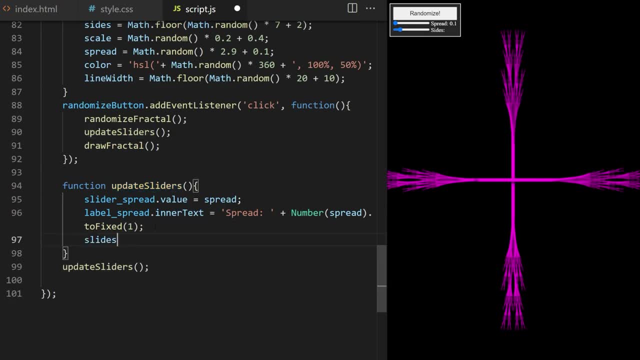 current value of slider. We update sliders and we draw a fractal. I also have to go inside my update sliders function and I update the value of slider and sides. We don't need to convert this one to number. It doesn't work. so I check my console. 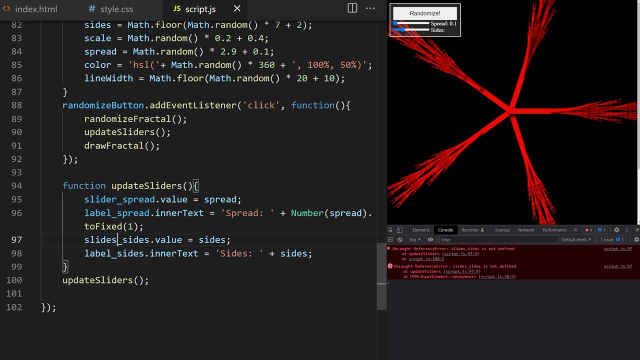 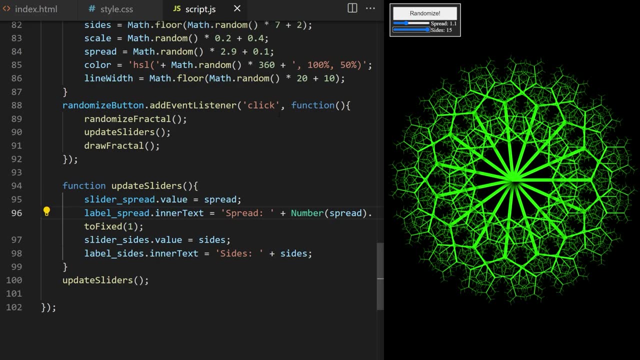 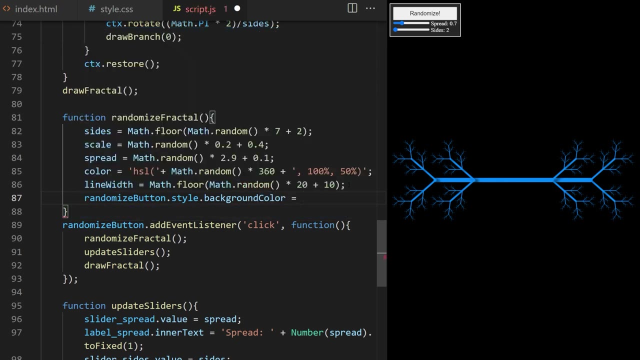 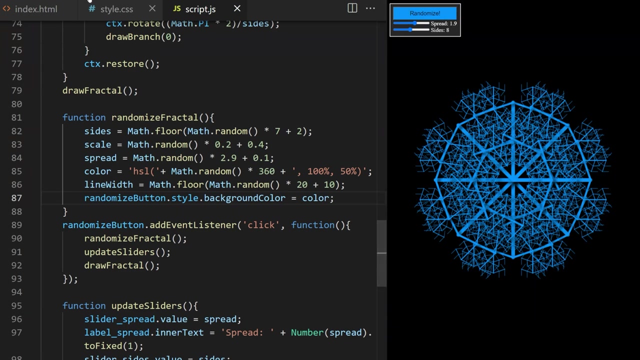 I can see we have an error on line 97. Here's my typo. Now it works perfect. When I press randomize button, I can, for example, set its background color to the current color of the fractal. like this, I can also create a reset button which will return our fractal to the default state in. 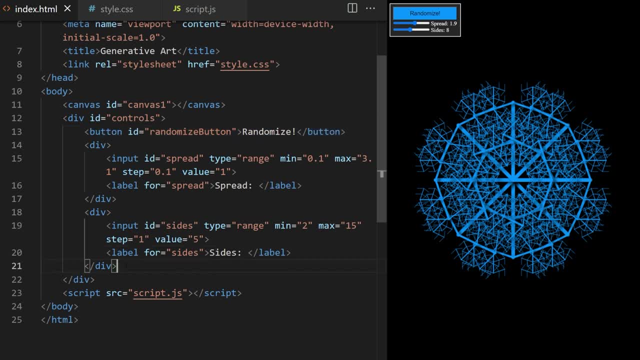 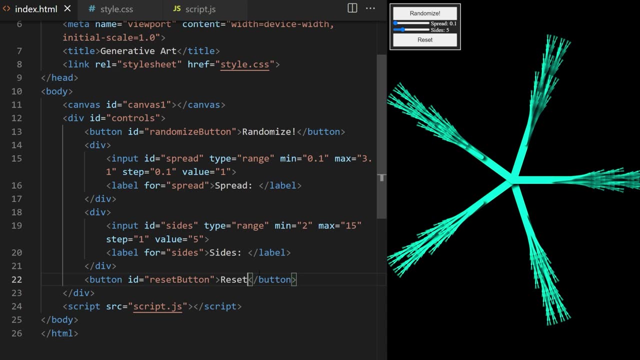 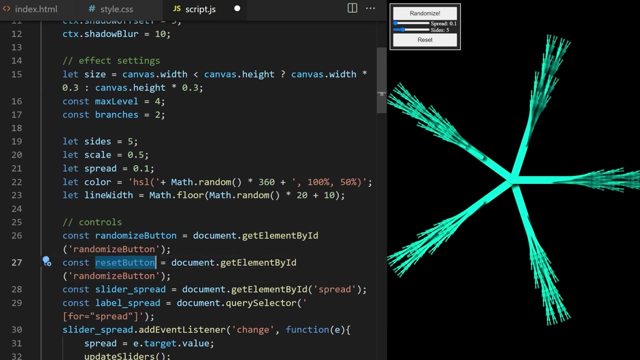 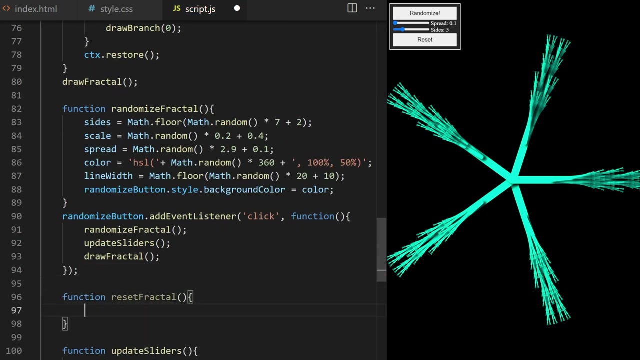 case we distorted too much. This is especially useful if you have more sliders than just create a button element with an id of reset button and text that says reset. I bring that button to my javascript project up here On line 97. I create a function called reset, fractal. Down here we will. 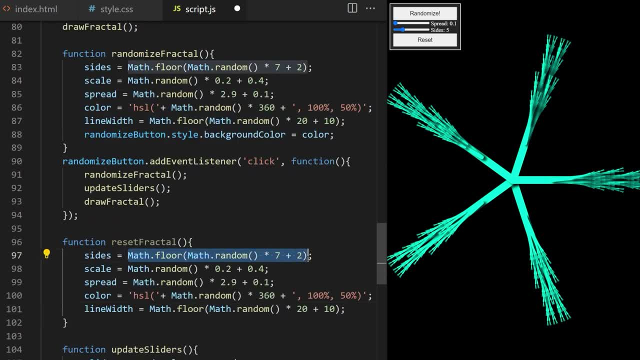 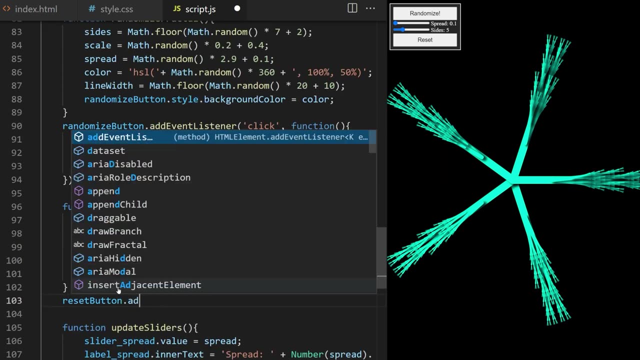 define some base values. our fractal will reset back to. I set size to 5, scale to 0.5, spread to 0.7, color to something close to purple or magenta and line width to 15 pixels. Add event listener. on reset button and on click I call reset fractal. 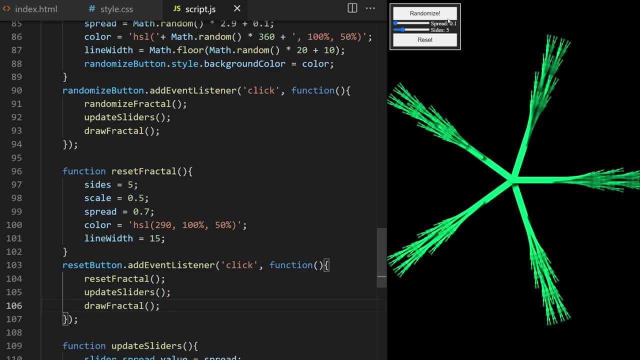 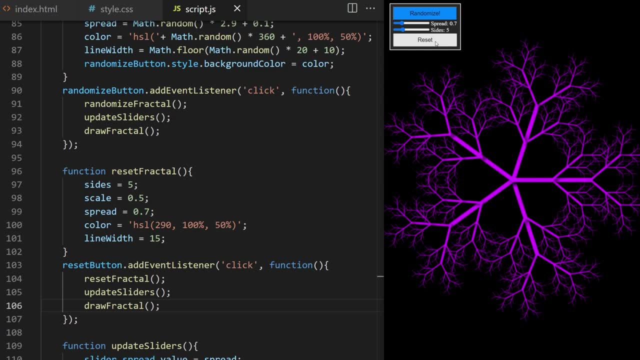 I update sliders and I draw fractal. This code can be optimized and cleaned up in many ways. For example, I can call update sliders from inside, draw fractal, because I want slider to update every time fractal is drawn. I'm writing the code like this in procedural way because I think hopefully it's easier to navigate. 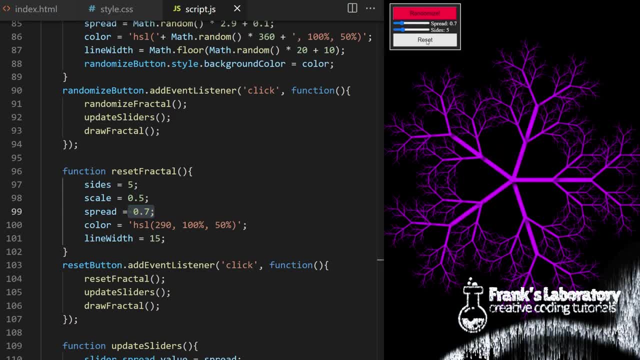 in it for beginners I will do object oriented version of similar code in other class. The main purpose of this class is to build something cool to get used to canvas drawing methods and also to really understand how fractals are made from scratch. You can see I use randomize button and 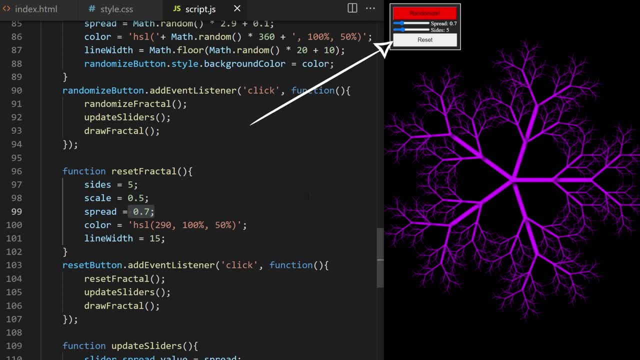 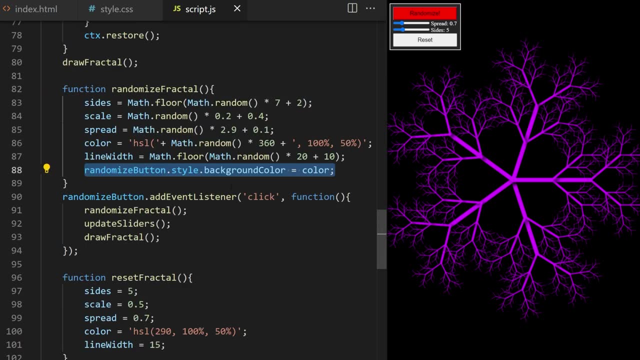 sliders to change fractal shape and I can reset it back to these values by pressing the reset button we just created. I take this line of code that changes color and I add a new one to it. I can see that the fractal is now in the color of randomize button and I put it inside: draw fractal. 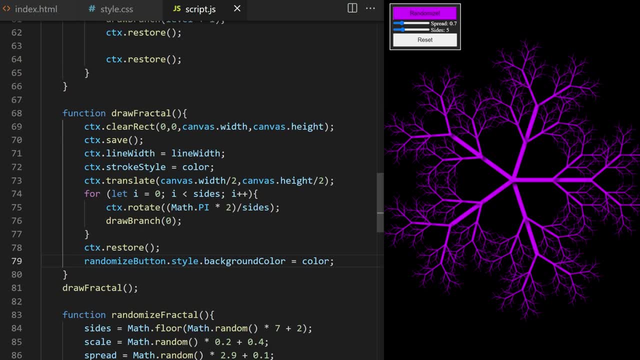 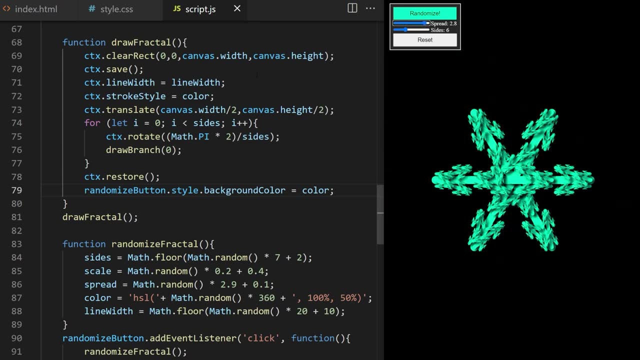 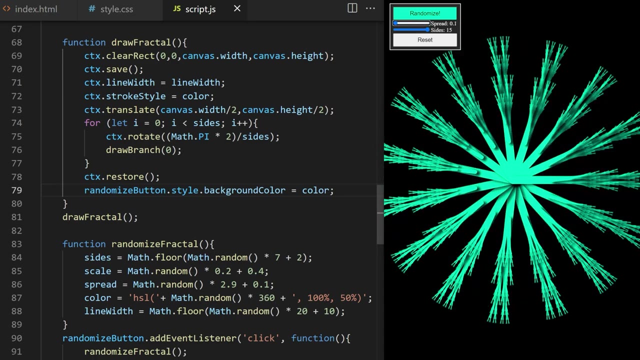 function. That way. button reacts even to reset, not just to randomize. We can randomize our fractal. We have slider for how spread out the branches are. We have a slider for how many sides our fractal is made out of and we have a reset button to undo all our experiments and reset the fractal. 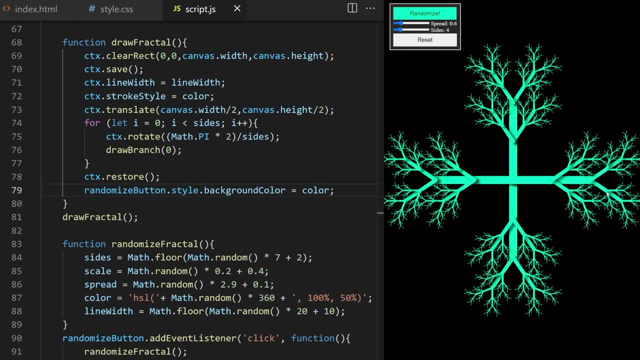 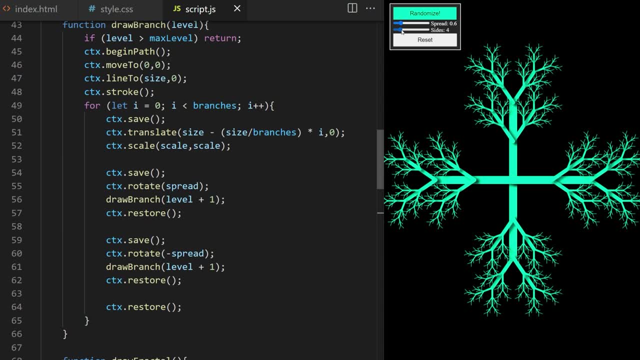 back to its default state. Let me show you one really cool thing you can do. now that you understand how fractals are made Inside draw branch, we are going to create a new fractal. We are going to start defining the base logic of how our fractal branches out. We have the main branch here and we 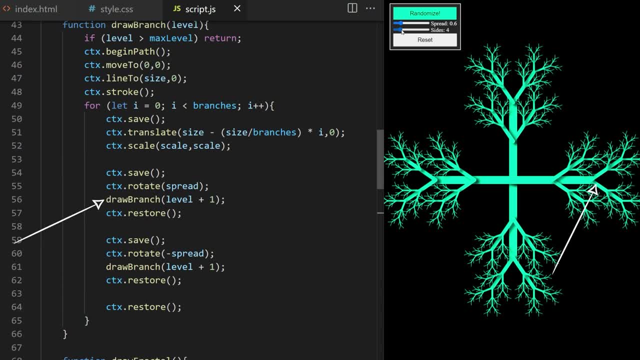 have two smaller branches coming out of it, One in the positive angle, one in the negative angle. There are many things we can change here to get completely different shapes. I will make some radical changes to the fractal now and I will delete some code. If you want, you can make a. 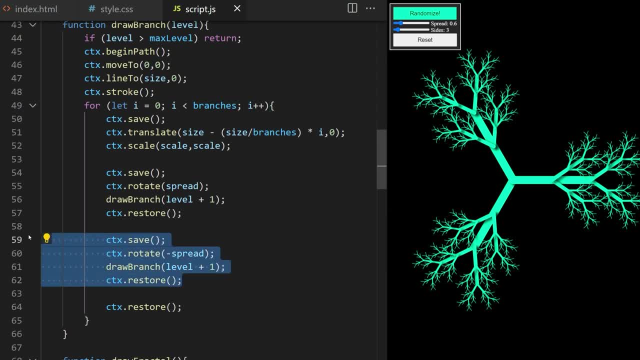 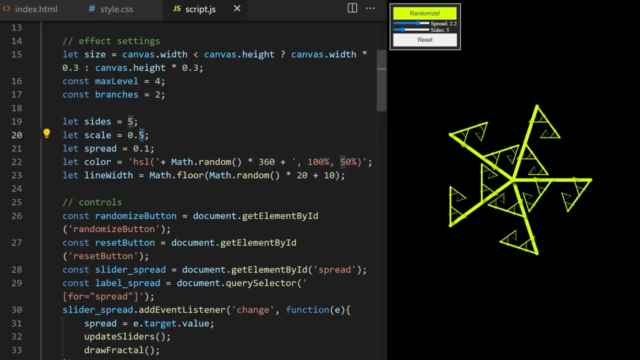 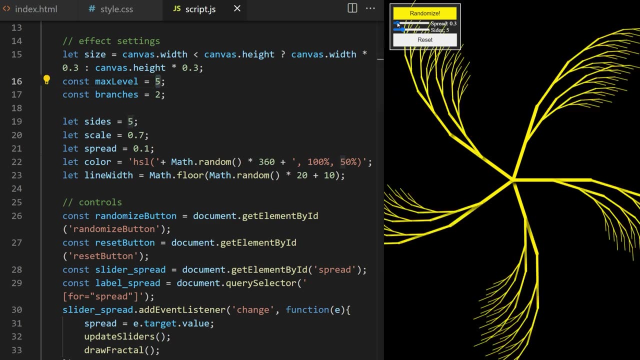 backup copy of this code base so you don't lose anything. I start by deleting this code block. I set scale to a different value. I set max level to 5.. Spread to 0.6. maybe You can see how max level 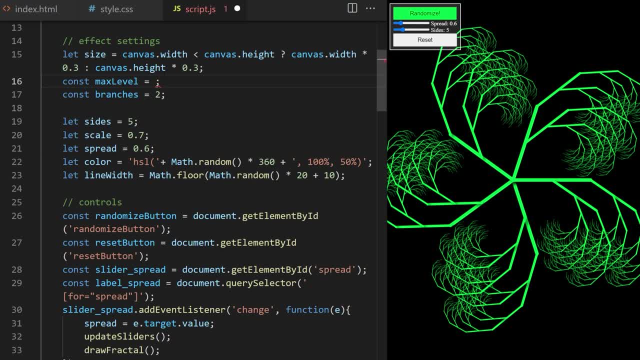 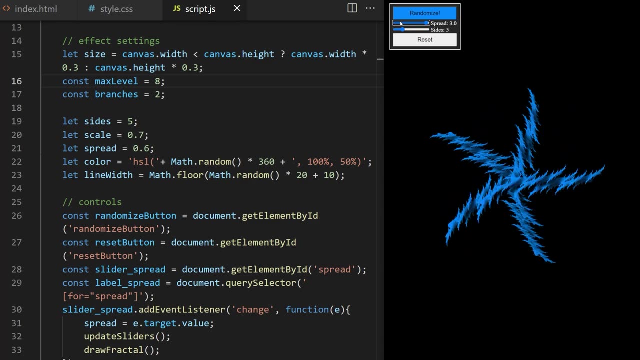 creates more depth in our fractal 7,, 8, 9.. I can afford to go a bit higher here because I'm only calling draw branch once from within itself. but be careful when changing this value. Don't go too high. it will affect performance At a certain point. increasing max level will add branches that are so. 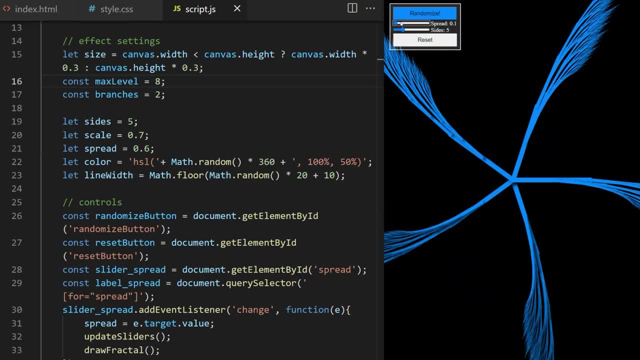 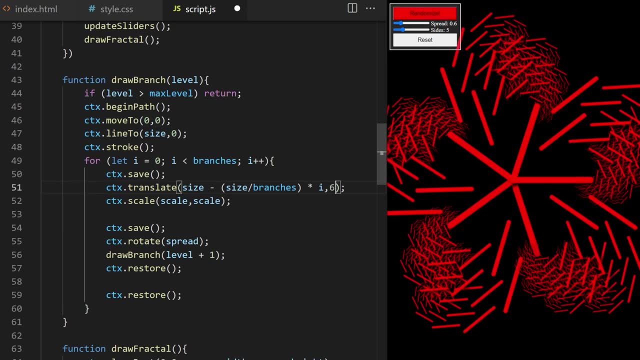 small, they are invisible, so it doesn't really make any visual difference. I get really interesting shapes when I play with spread slider. You can also create this broken floating fractal shape by increasing y coordinate argument. passed the translate method, I set it back to zero. I can. 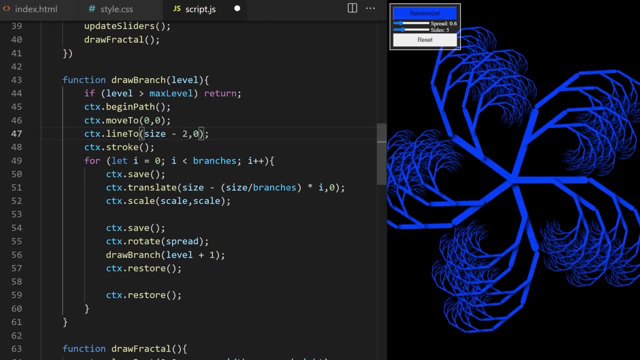 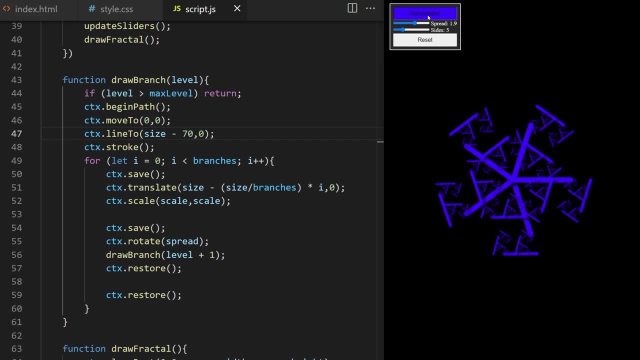 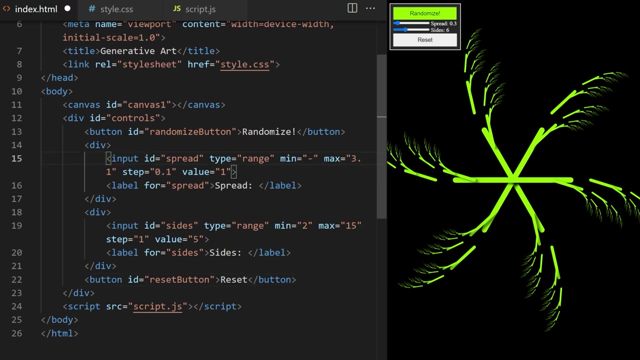 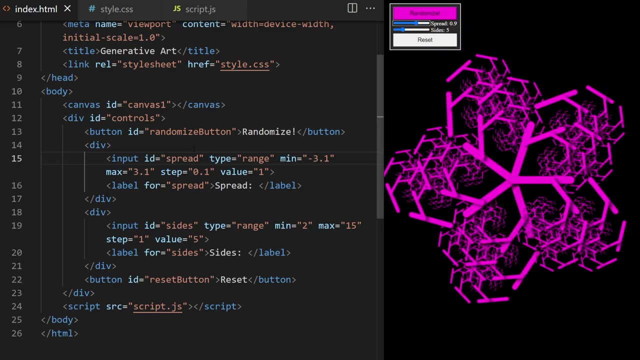 create overlap of spaces between branches here. This could also look interesting. I like this. What if I let spread range to go to negative values? let's say minimum is minus 3.1 and the maximum is plus 3.1. i go from the maximum down and around zero. we get this flip to the negative. really cool. what else i 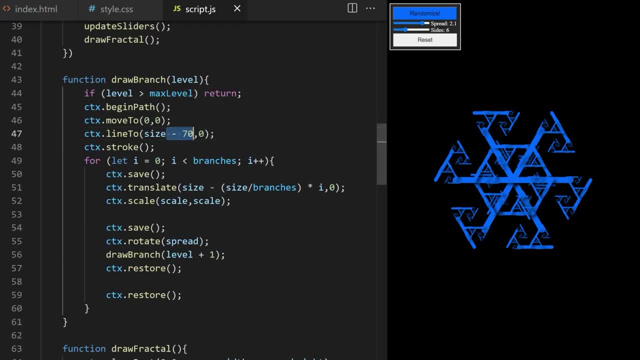 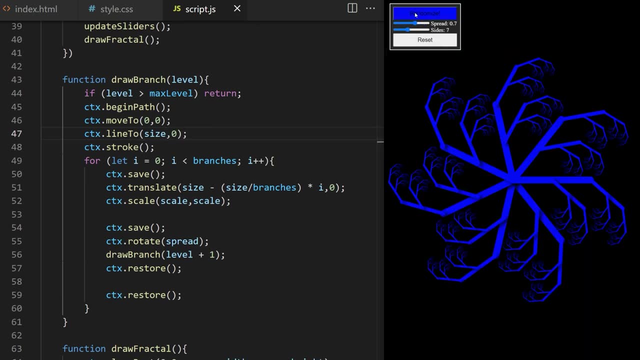 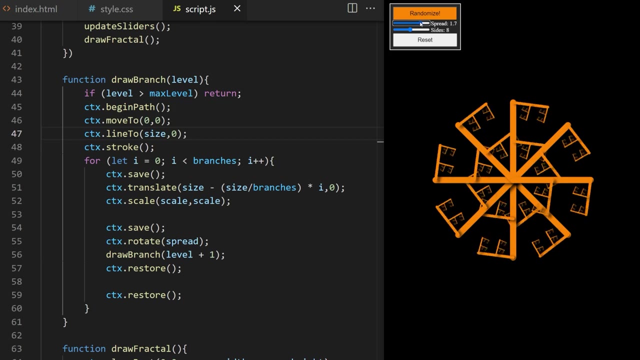 could do here. i set line 47 back to how it was. i can also add additional shapes to our fractal. it doesn't have to be made out of lines. we can use circles, rectangles, images, patterns. try to combine this with all canvas techniques. you know you might get something unique. 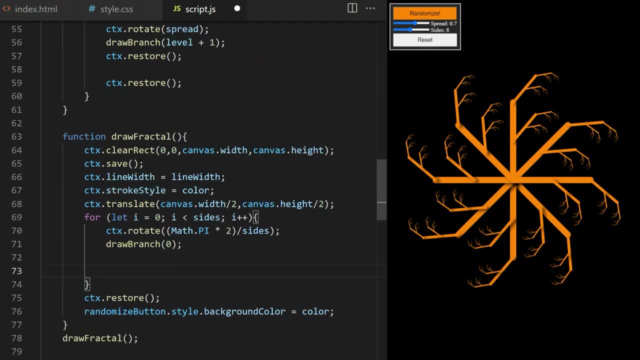 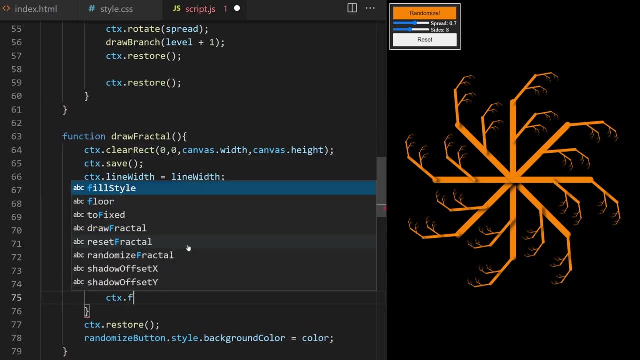 now i want to draw a circle, so begin path arc method and we draw that circle at coordinate 0, 0, radius 50, start angle 0 and angle 360 degrees. so math dot pi times 2 and i call fill. i adjust vertical y coordinate to match the size of branches. 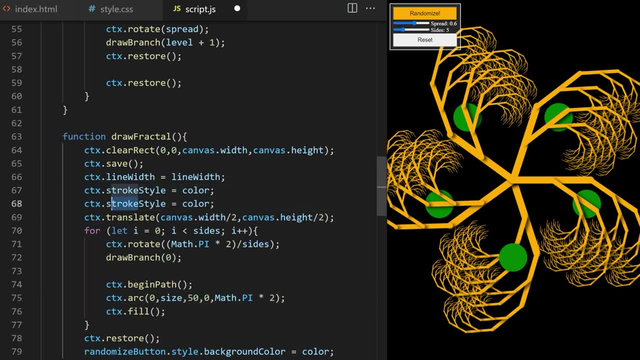 i set fill style to the same color as the circle and i call fill. i set fill style to the same color as the circle and i call fill. i adjust vertical y coordinate to match the size of branches. i set fill style to the same color as the circle and i call fill. i adjust vertical y coordinate to match the size of branches. stroke style. 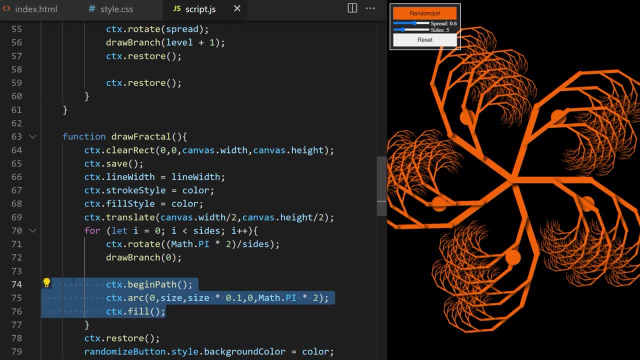 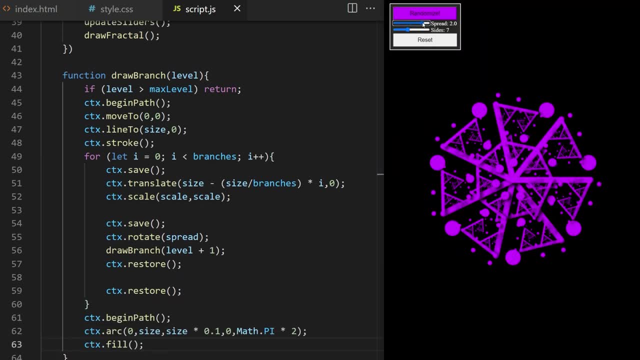 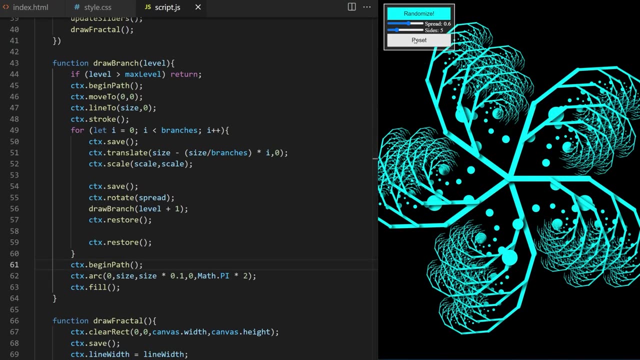 i make the radius relative to size. i cut this code from here completely and i paste it inside draw branch outside this for loop. yeah, this is what i was going for. let's quickly fix a few things we have here. when i take the spread slider to the negative values, 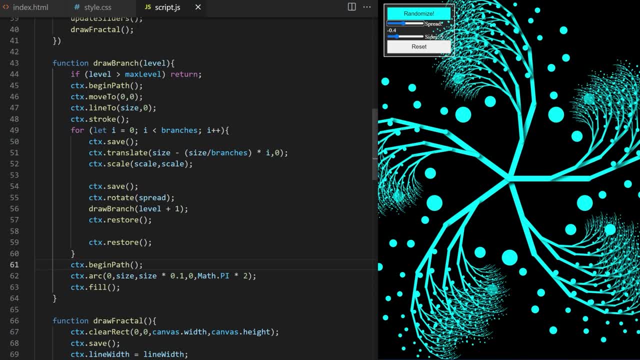 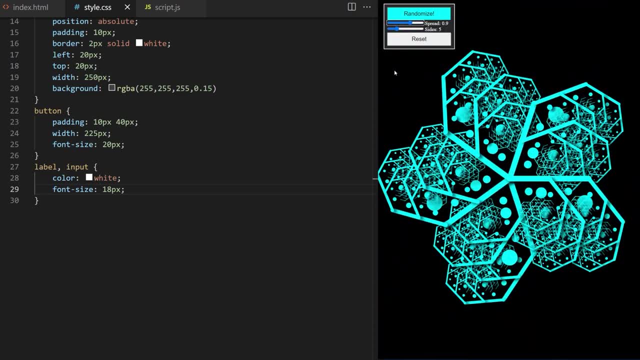 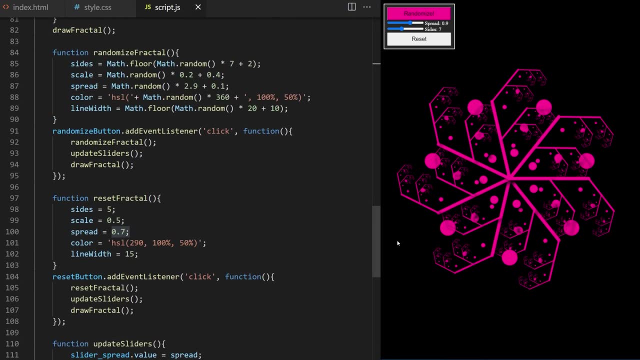 the minus sign pushes label to the next line. i can reduce font size to 80 pixels to fix that. when i press randomized with this new shape, i feel that this scale is set too low. i set scale to a random number between 0.4 and 0.8, maybe. yeah, that's better. 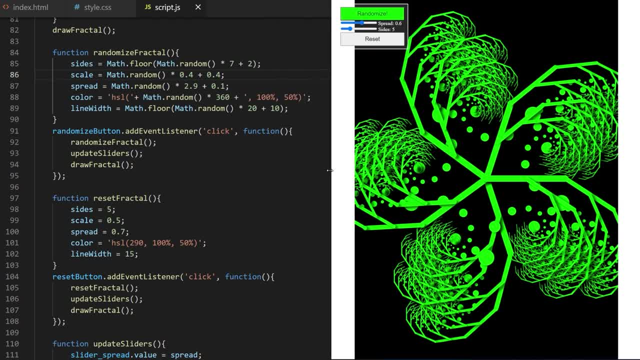 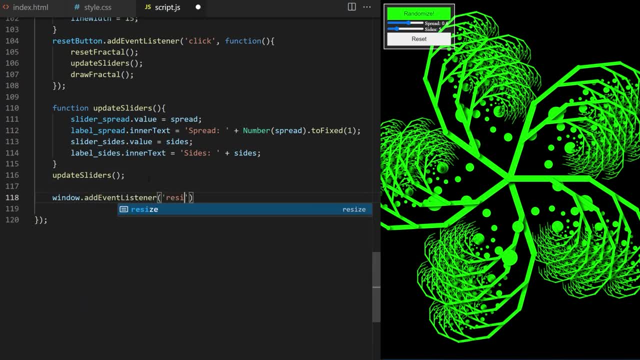 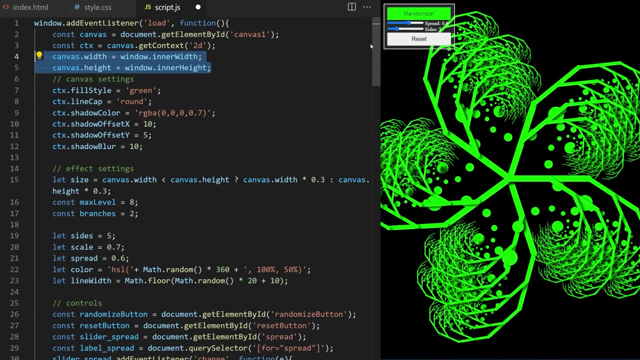 the effect is currently not responsive when we resize browser window. this is also easy to fix. it's similar for all canvas projects. i create an event listener for window resize event. when the browser window is resized, we have to resize canvas so we set its width and height to the current dimensions of the browser window. resizing canvas deletes everything. 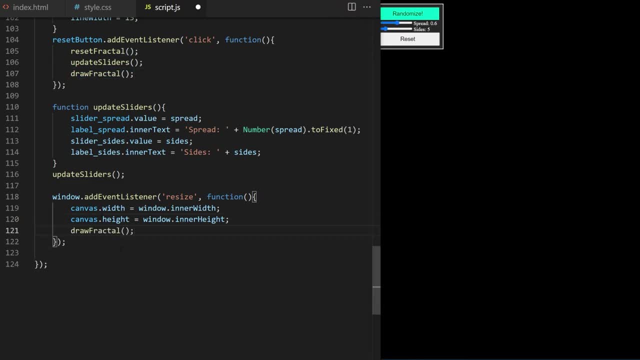 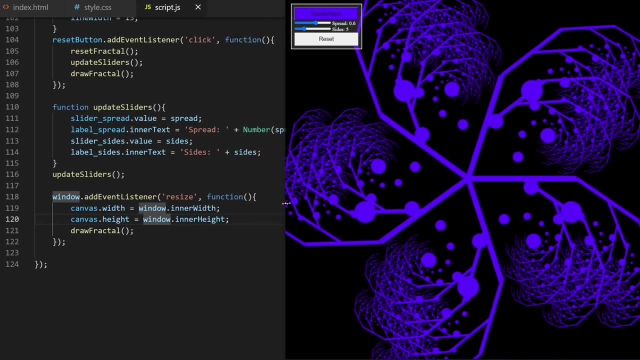 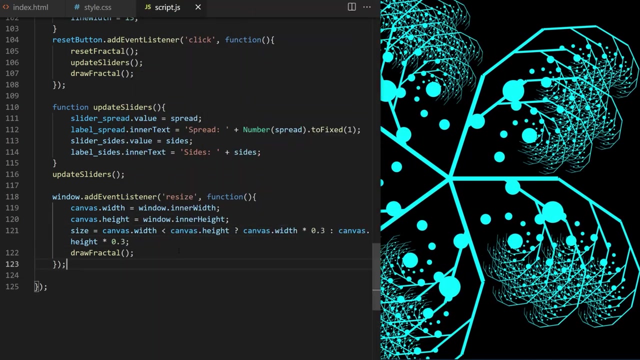 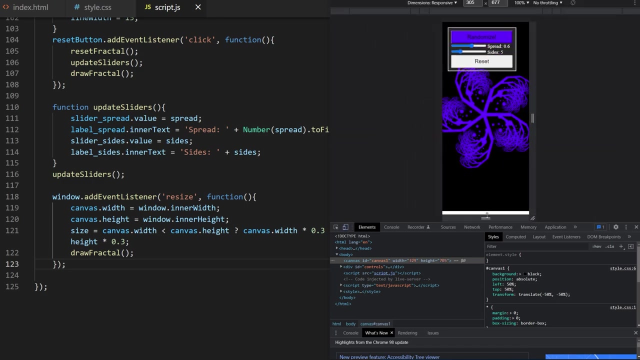 that's drawn on it. so i have to call draw fractal after. i would like the fractal to change size based on width and height of available space. if the width is smaller than height in portrait mode, it will be restricted by screen width. if we have a wide landscape screen, we will be limited by its height. this line of code will make: 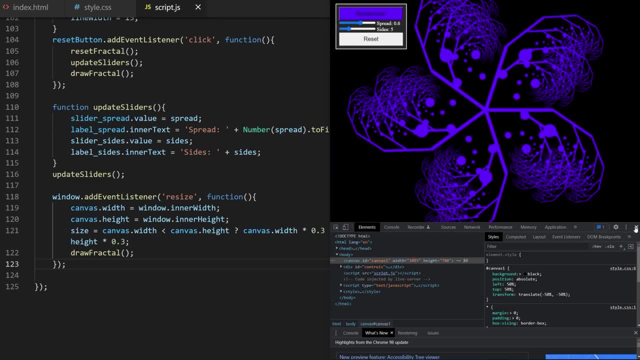 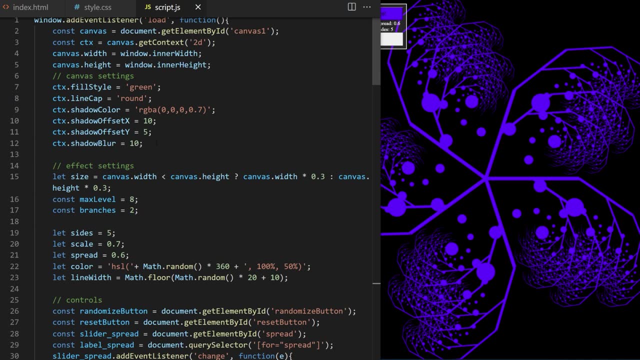 it work on all screen sizes. another quick reminder: if you want this to render faster on mobile, the easiest way is to decrease value of max level variable on line 16.. i notice that when fractal resizes we lose canvas shadows for some reason. you don't have to use shadows on this effect, but if you 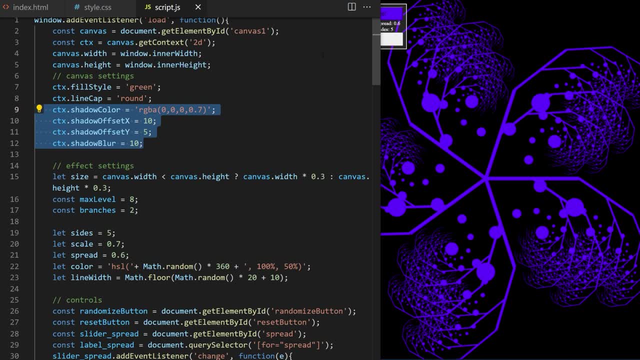 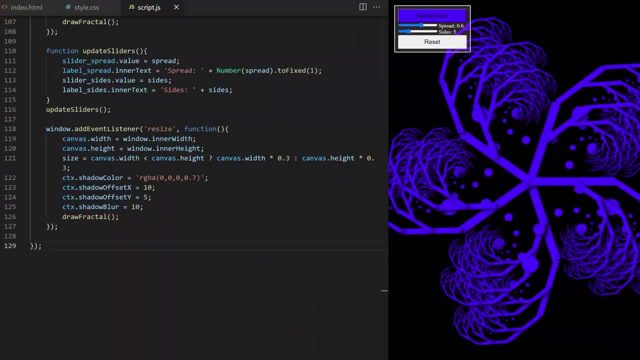 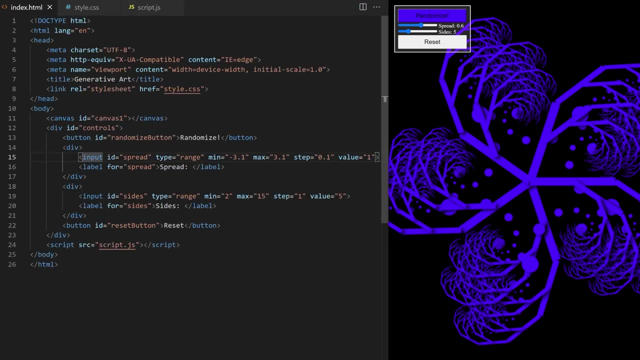 want to use them, we just have to redeclare these properties inside resize event. with some fractal shapes, shadows make it so much better. i want to show you another way to get unique and really cool shapes with this code base. again, we will make radical changes to the code now, so if you 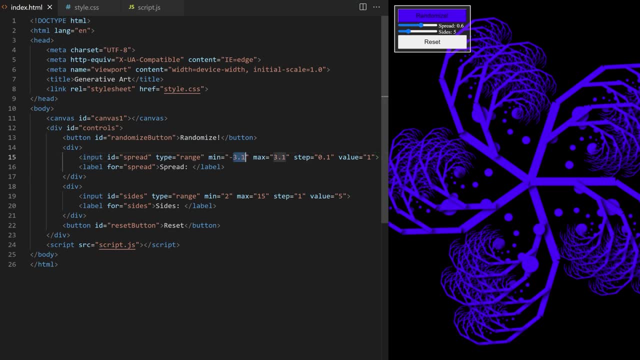 want to keep this code base as a copy. maybe save it before we start this next experiment. i go to my sliders and i set minimum on the spread slider to minus 0.3 and step will be 0.3. side slider will have maximum value of 22.. in reset fractal function i set spread. 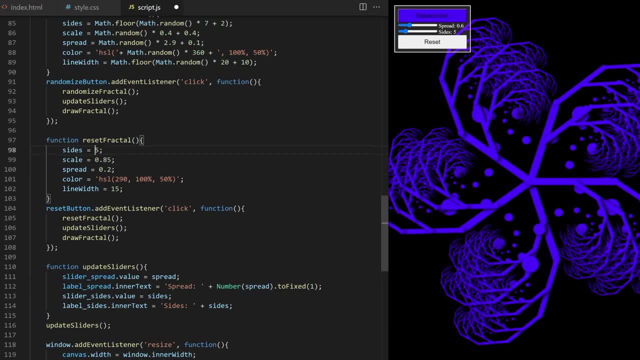 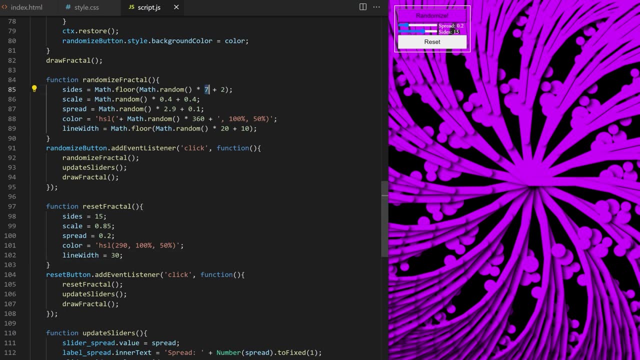 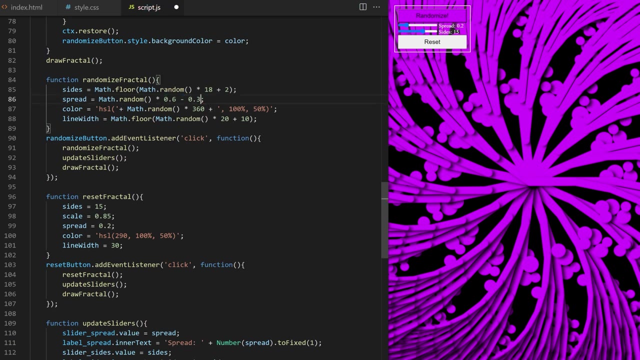 to 0.2, scale to 0.85, sides to 15 and line width to 30.. inside randomize fractal, i set sides to a range between 2 and 20.. spread will be a random value between minus 0.3 and plus 0.3. line width will be: 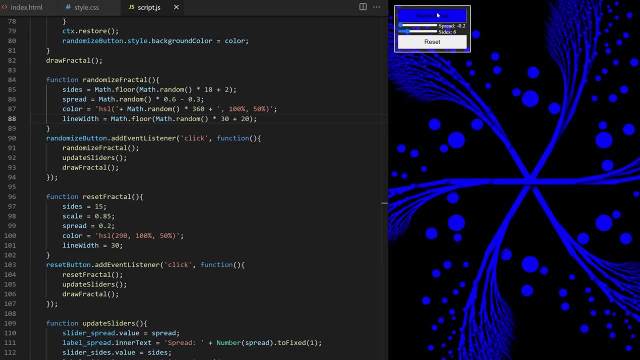 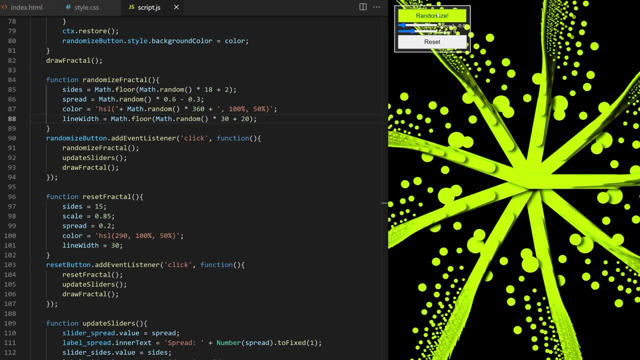 a random value between 20 and 50.. if you are getting a bit longer render times, it's not a problem. the final fractal we draw today will be efficient and fast. but i want to show you some cool shapes we get in between. complex shapes have more detail and they take longer to render. 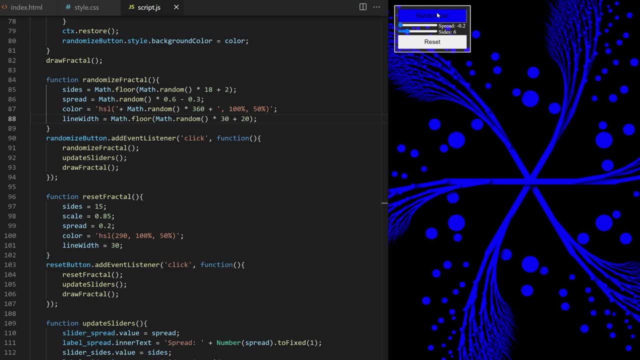 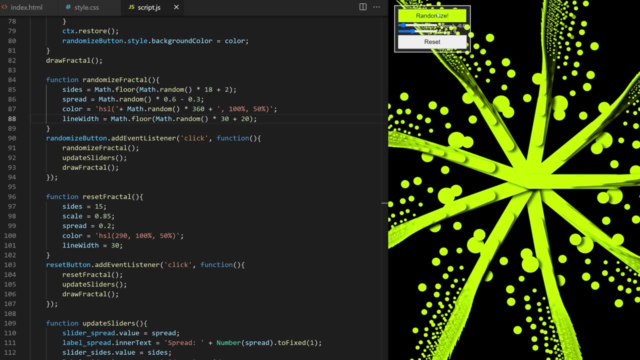 it's intentional. however, if you want your fractals to be drawn faster right now, go up to line 17 and set branches variable from 2 to 1.. when you set branches to 1, you will get much faster render times. some of the fractal shapes you will get now will be much faster than the fractal you will get. 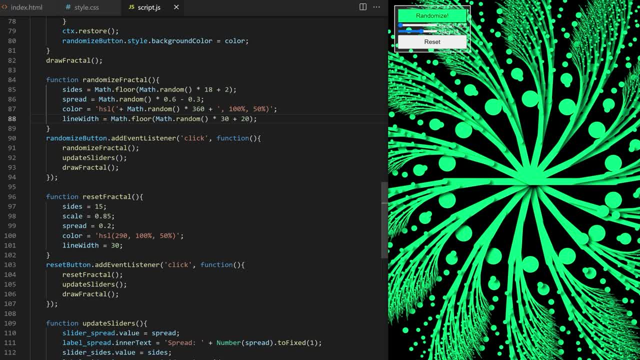 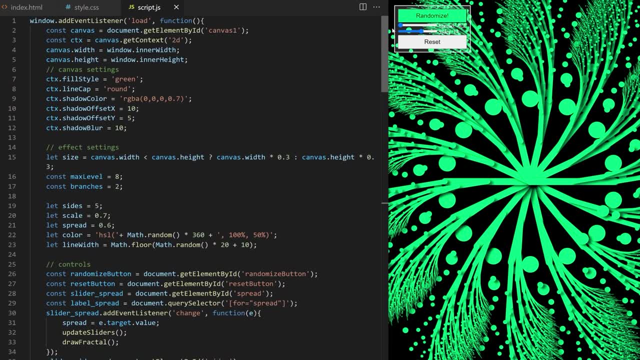 different than mine, but we will end up with the same shape. i will also reduce my branches to one. i will just do it a bit later. these are creative coding experiments, so feel free to do whatever you like at this point. effect settings are global variables that affect the shape of the fractal. 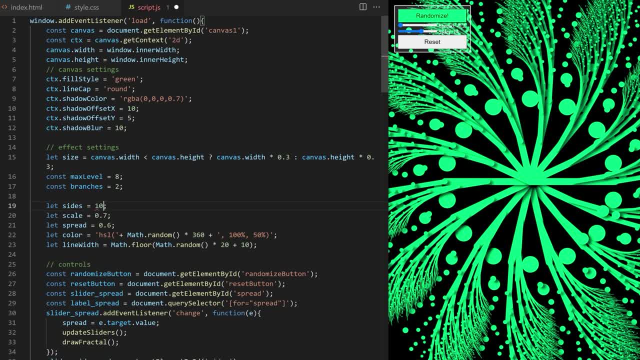 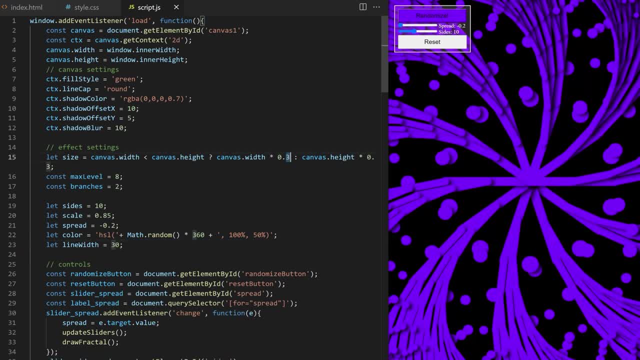 on the initial page load. i want to start with 10 sides, scale 0.85, spread minus 0.2 and line width 30.. i also want to make it much smaller, so size modifier here will be 0.1 and size modifier will be. 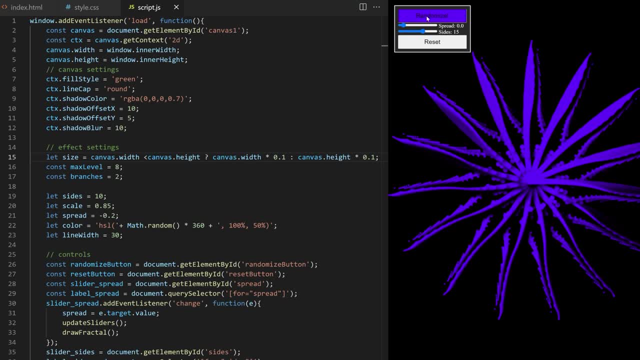 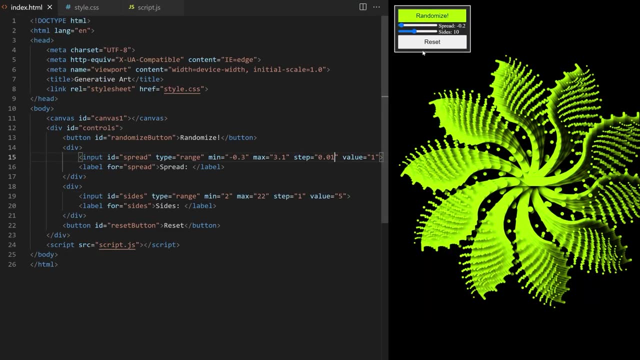 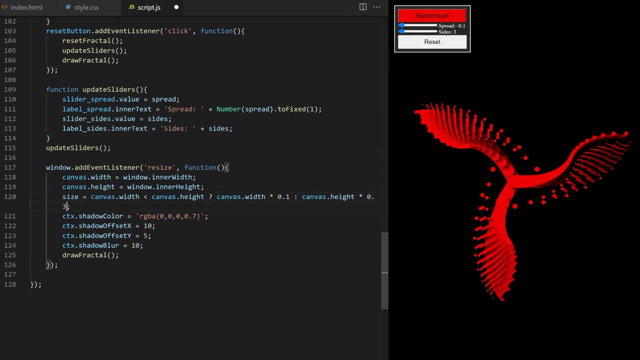 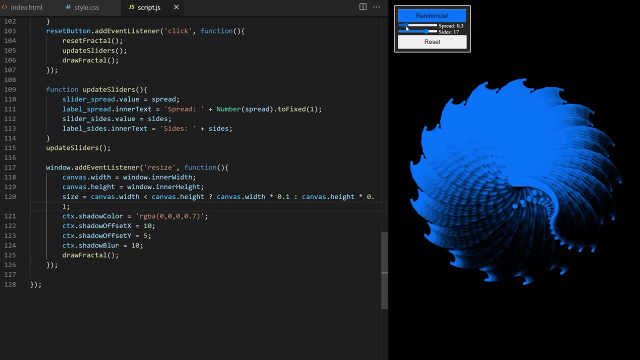 1. i really like these shapes. what do you think? i change step on spread slider to 0.01. i set size modifier inside resize event to 0.1 as well. this fractal shape has a lot of individual draw calls. it takes a while to render, but we get this. 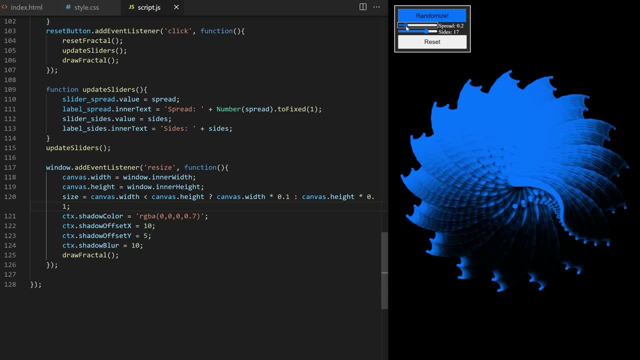 beautiful result, actually. let me know in the comments how long does it take your computer to do this and if you want to see more videos like this, please subscribe to my channel and hit the bell icon so you don't miss any of the videos. i draw this fractal right now. does it take too long? 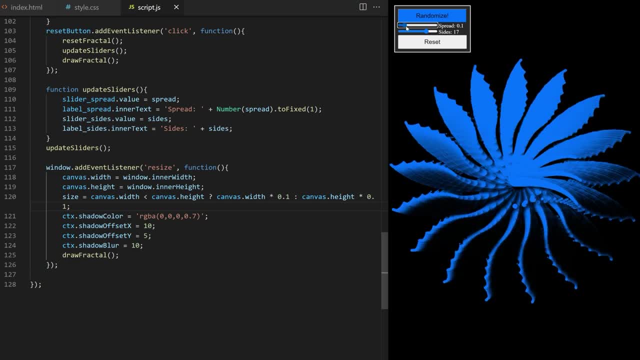 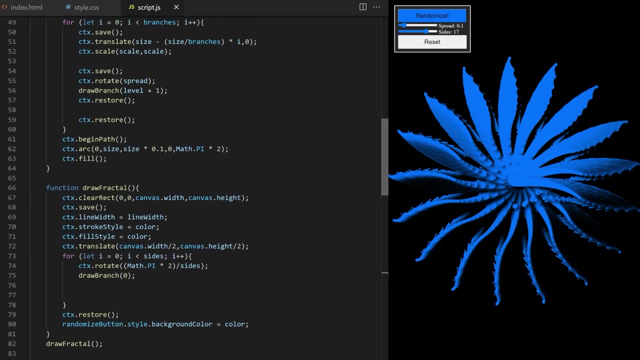 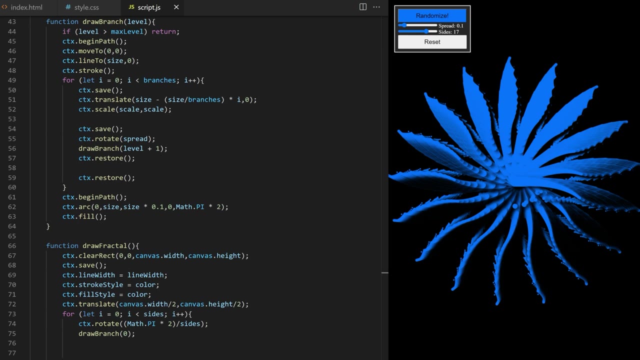 to render? if so, can you let me know the specs of your computer please? you can set branches to one or remove canvas shadows to get much faster render times. i want to replace line 2 method, which we are using to draw one straight line, with bezier curve 2 method. bezier curve 2 method allows us to specify: 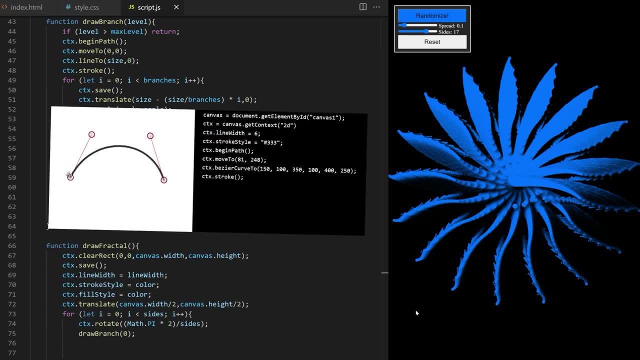 two curves. we set the starting point with move to method and then we pass it six arguments: each pair is x and y coordinates of a curve. and then we pass it six arguments: each pair is x and y coordinates of a control point. so this is control point 1, control point 2 and the end point. let me show you how to. 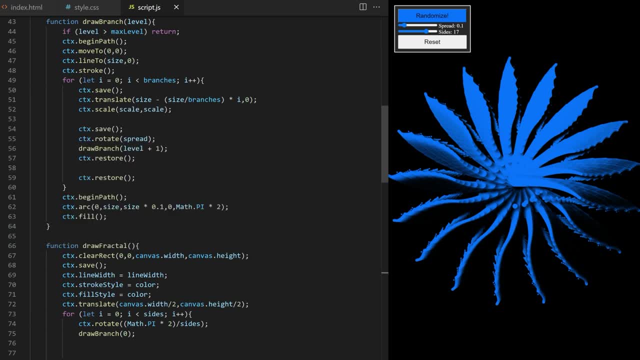 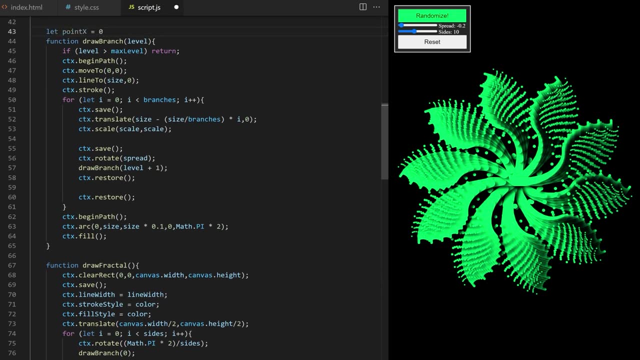 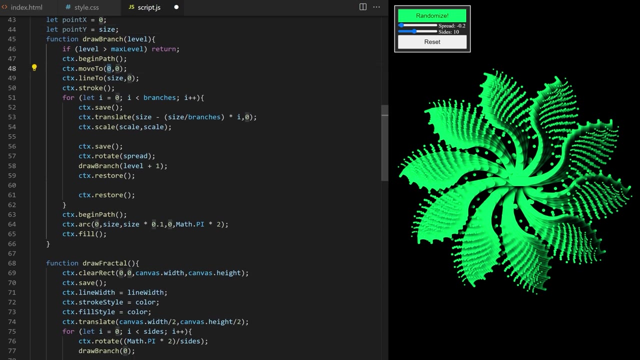 use this in an actual drawing. i want the starting coordinates and coordinates we translate to to be connected. so i create a variable. i call, for example, point x and i set it to 0 and point y and i set it to size variable. like this, i pass point x and point y as start in x and y coordinates of. the curve here in move to start u. so i just circle theanga curve and dói and do більBAČĎĎČĎĎĎČĎĎĎČĎĎĎĎĎĎĎĎĎĎĎĎĎ. 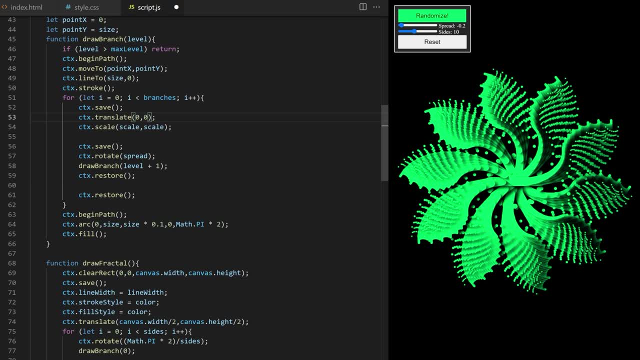 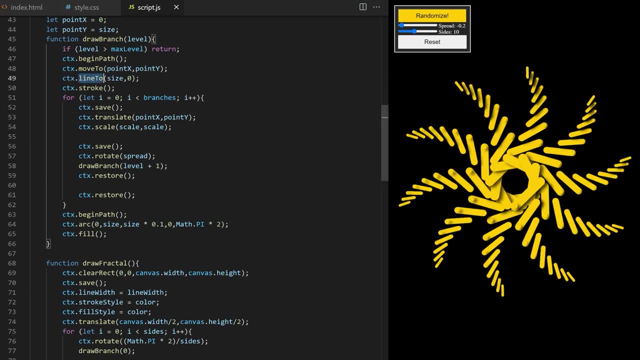 moveTo method and then, as we translate along the parent branch to draw smaller branches, I will translate to the same coordinates. You will see what it does in a minute. So, as we said, Bezier curve 2 takes 6 arguments. control: point 1 will be size and 0, control. 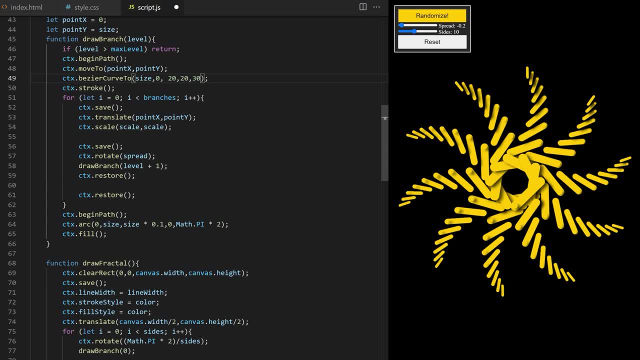 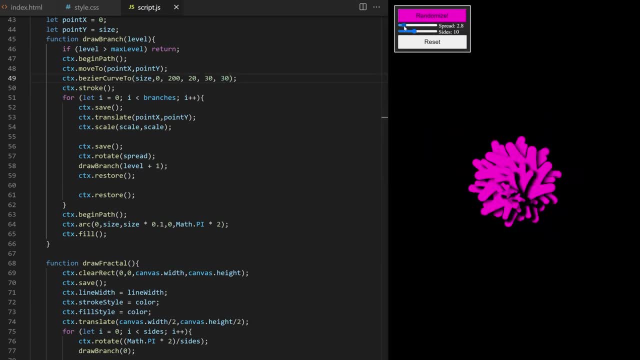 point 2 will be 20, 20, and the end point will be 30, 30.. If I increase some of these values, the curve will stretch further towards that control point. You can play with it, because that's the best way to understand how these values affect. 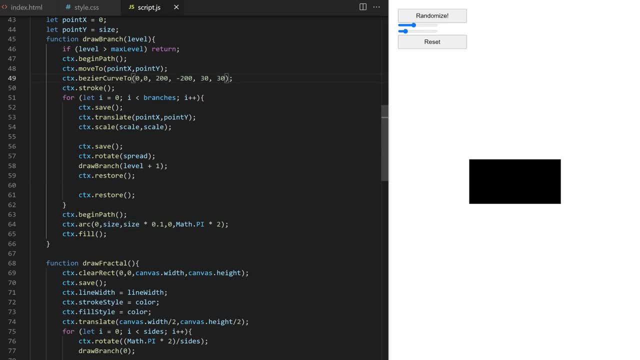 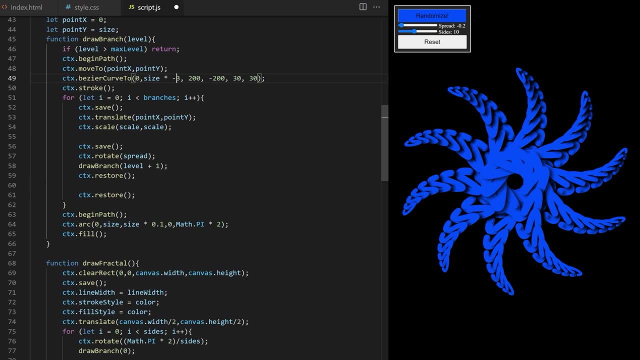 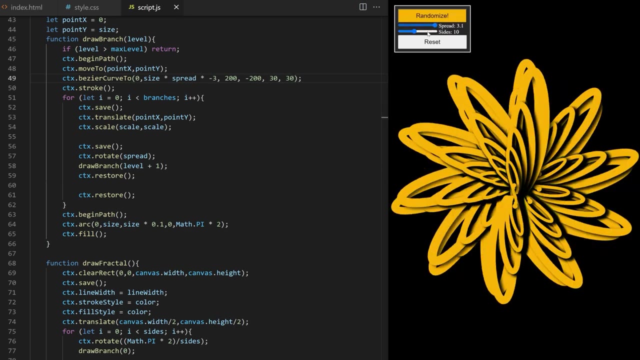 the final shape. I set the first control point to 0 and size for x and y Size times 3.. Size times minus 3 will give us better curves. I can also include spread value in that calculation. The second control point: let's try size minus 200.. 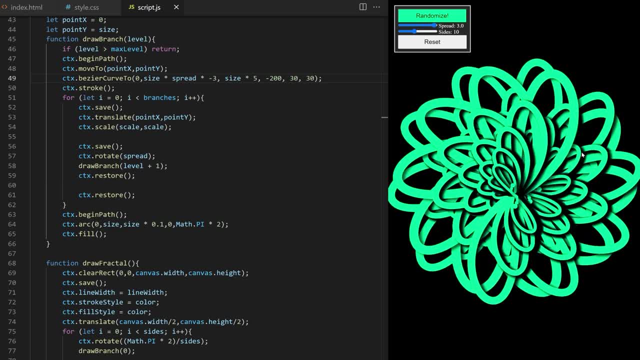 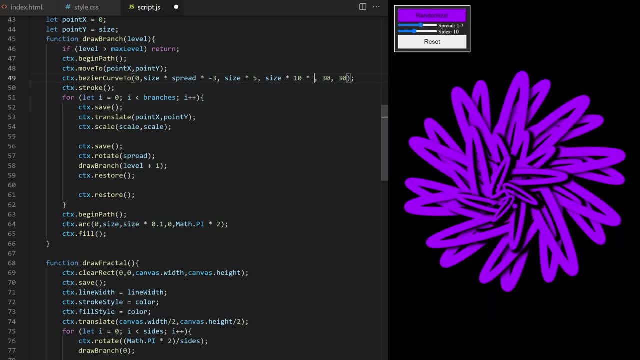 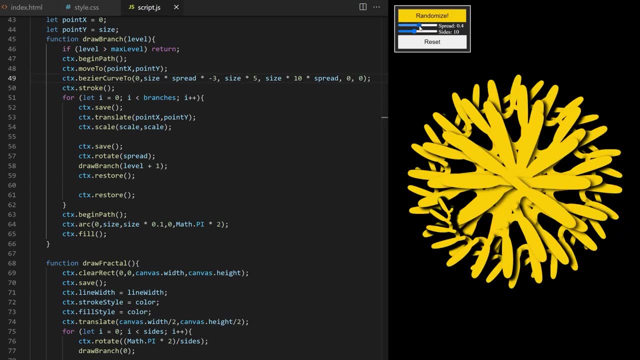 Size times 5.. Size times 5 for x and size times 10 for y. I also include spread in this. I'm just experimenting now. I set the end point to coordinate 0, 0.. We are building the octopus fractal, so I actually wanted the range to be between minus 0.3 and. 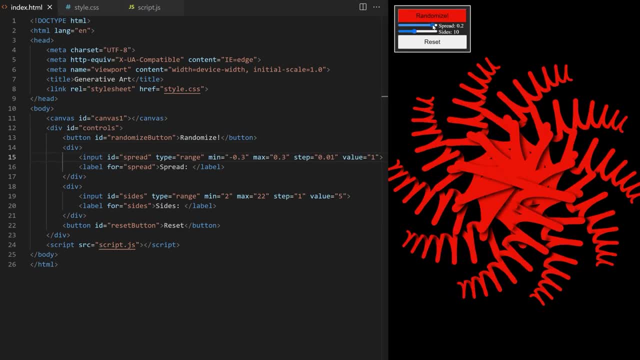 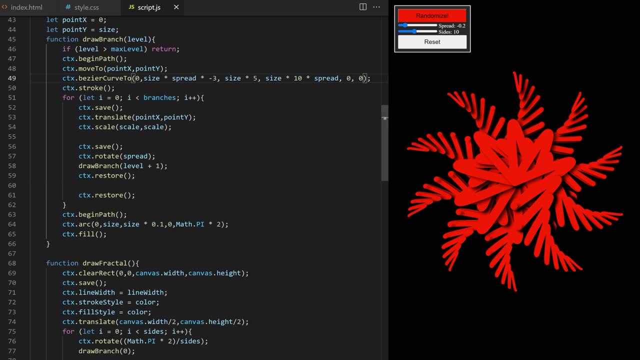 maximum plus 0.3.. Can you see the curves now? So in my head, these are tentacles, and now we need to create the suckers. I'm going to create the suckers. Octopus has suckers on its tentacles. 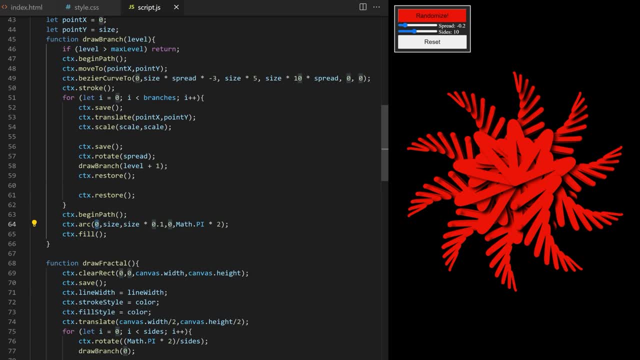 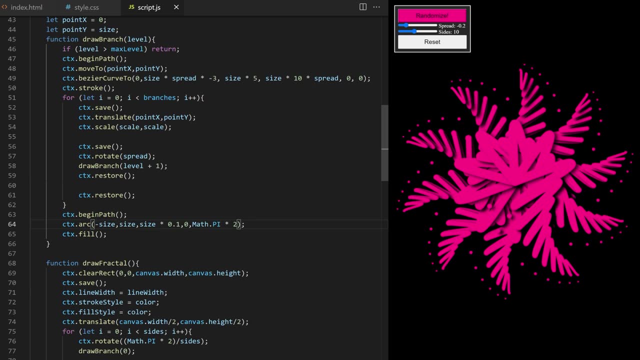 We are already drawing circles down here. If I change this x coordinate to minus size, I will push them outside like this. Nice, If I want them to be closer to the tentacles, I divide size by 2.. I set the y coordinate to 0 for better alignment. 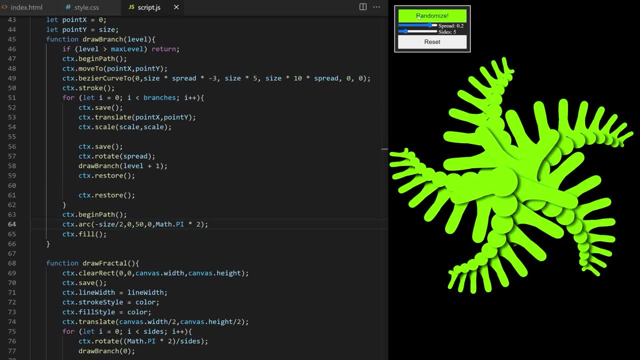 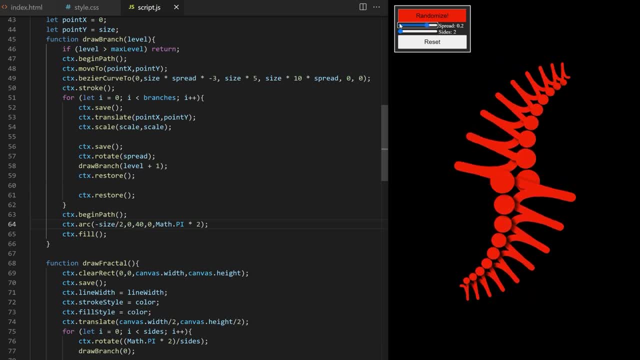 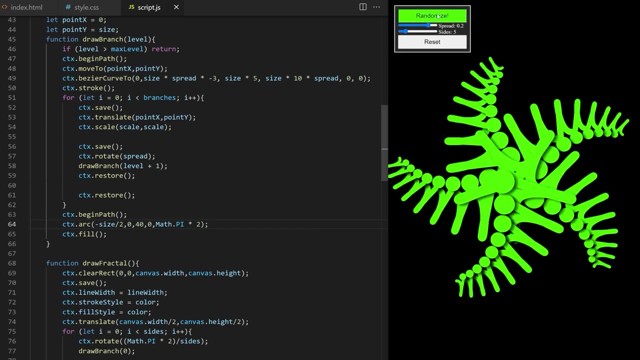 Radius of the circles will be 50 pixels. I make them a bit smaller, maybe 40 pixels. We are actually not being very efficient because I have two branches right now, as defined on line 17,. so we are drawing some shapes twice, but we can't really see them since they completely 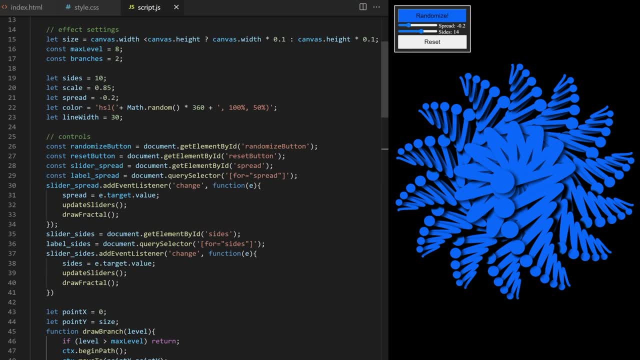 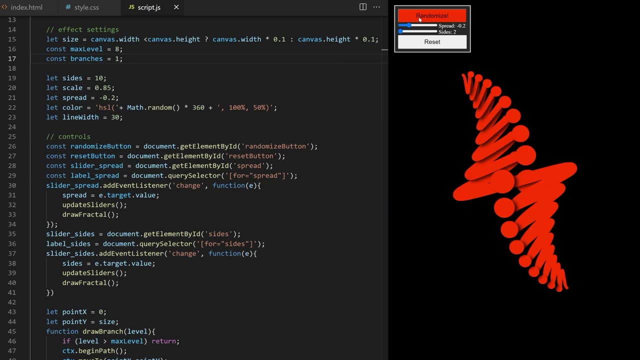 cover each other. I go up to line 17 and I set branches variable to 1.. You will notice we get the same shapes but we also get much faster render times. When I move my sliders now, the fractal responds and moves much faster. 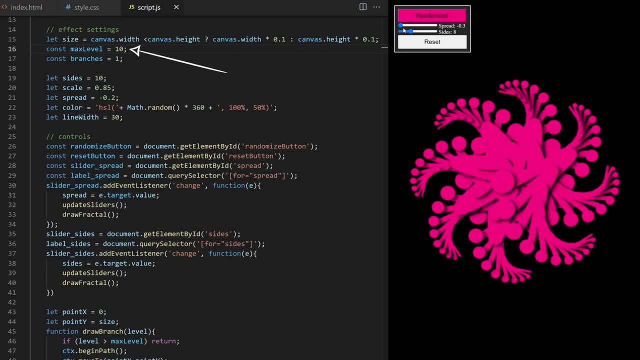 If you want the tentacles to be longer, you can also increase maximum. You can also increase the length of the tentacles. If you want the tentacles to be longer, you can also increase maximum. I will use 10 because my computer has no problem rendering that. 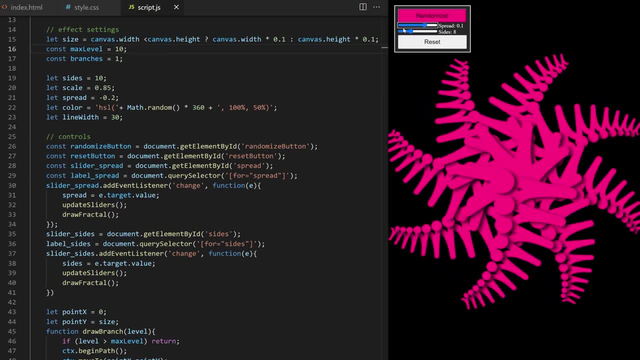 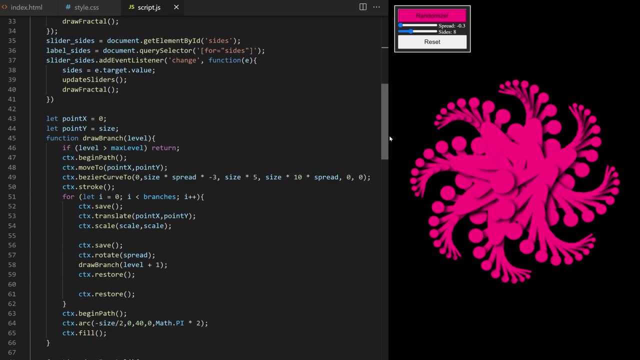 I really like this shape, but for a natural shape it's too symmetrical. I want this to look more like something that was created by nature rather than an algorithm. Let's break the radial symmetry a bit, and then we will restore it in a more complex. 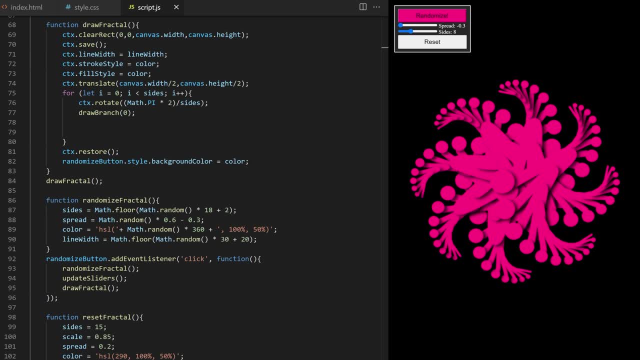 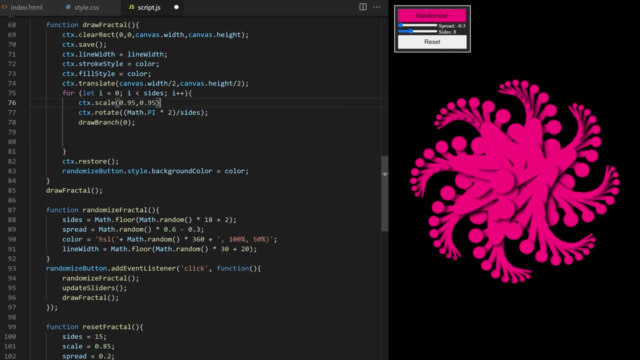 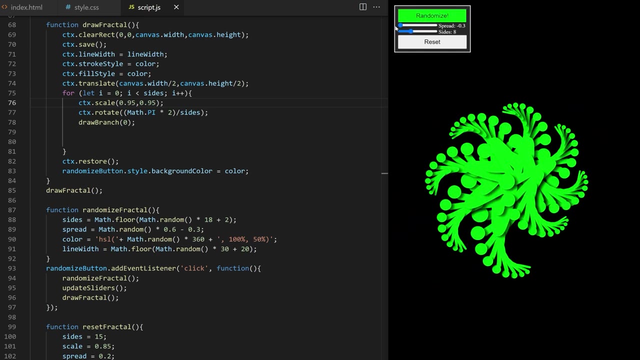 and better looking way Inside. draw fractal every time we create a new tentacle. now we have 8 tentacles between each one. we will scale canvas drawings down to 95% vertically and horizontally. This could probably be tweaked and adjusted into a pretty cool snail shell. 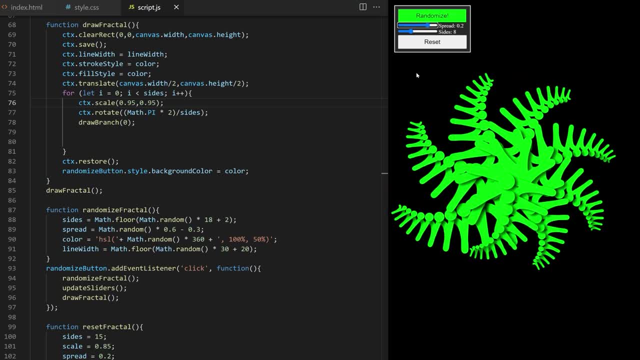 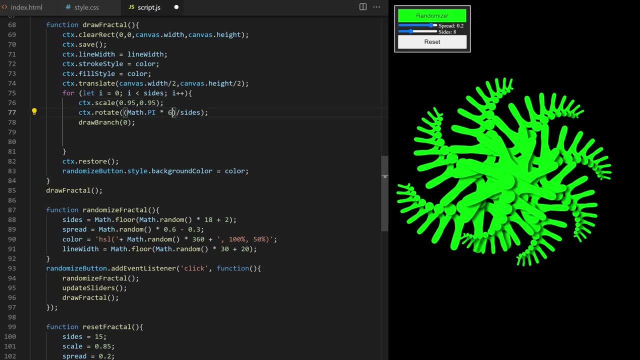 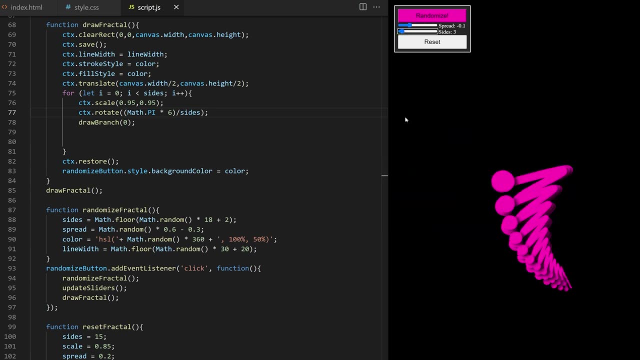 To complete our octopus fractal, instead of spreading our tentacles in an area of a circle, I split them in an area of 3 circles, so mathpy times 6, and we get shapes like this. At certain breakpoints we get really cool layers and symmetry, for example when we have 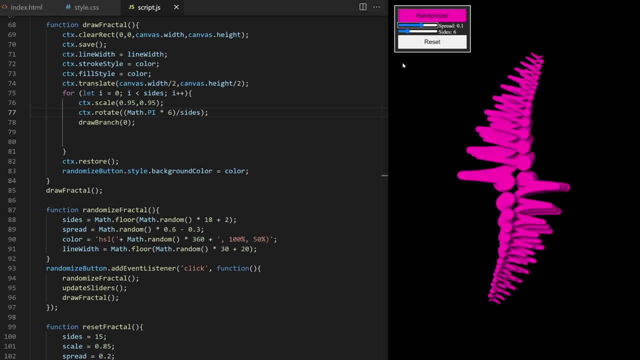 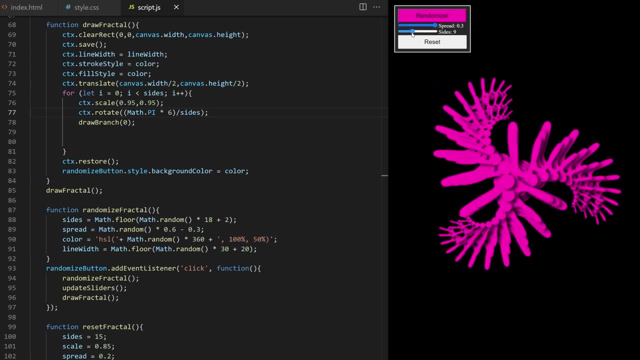 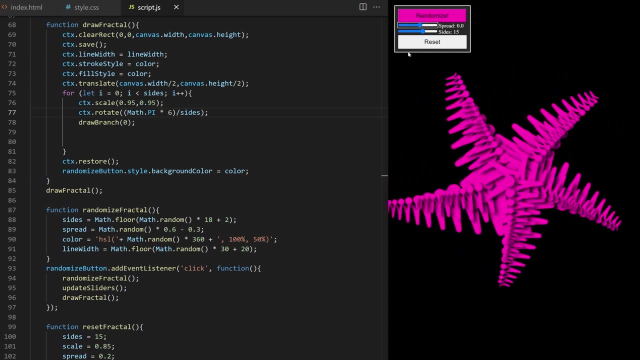 this 6 sided fractal like this, Or 9 sided. Look at how they cover each other 3 at a time. this looks so good. This one at 15 sides is my favorite. I know octopus has 8 arms, but my octopus is special. I'm taking some artistic license. 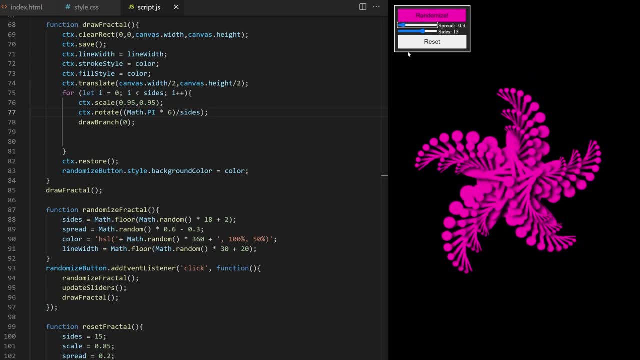 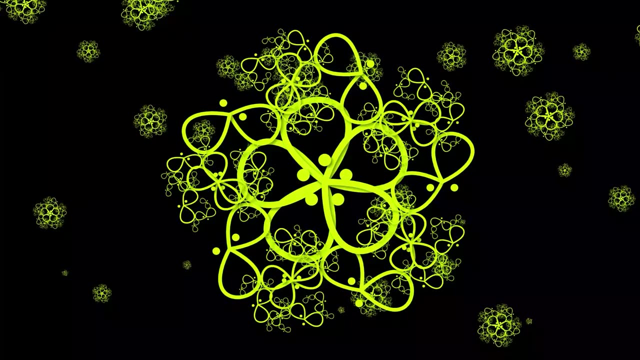 here. If you want to take what you learned today further, I have another class on fractals, where I write everything in object-oriented code structure, again with plain vanilla javascript and no libraries. If you want to take what you learned today further, I have another class on fractals. 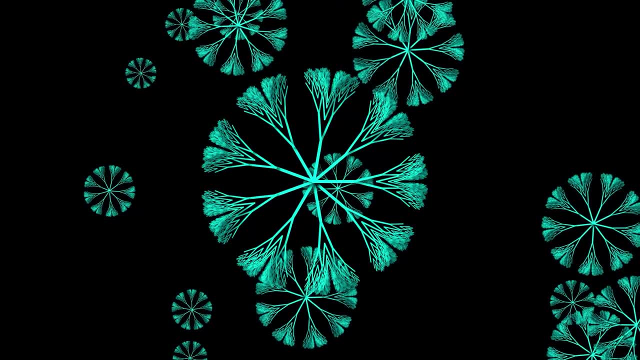 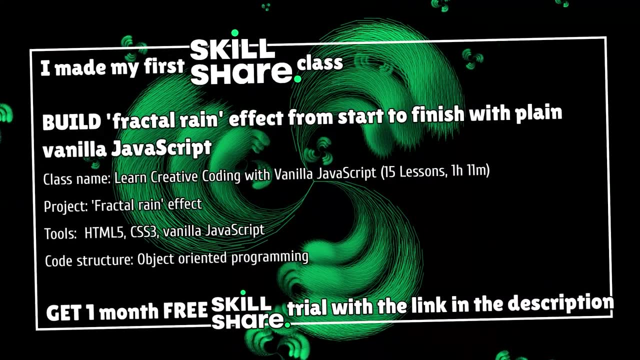 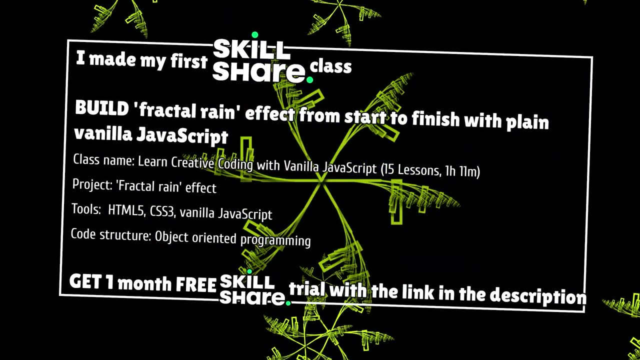 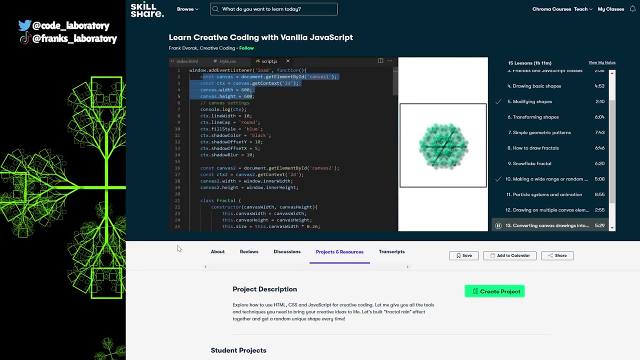 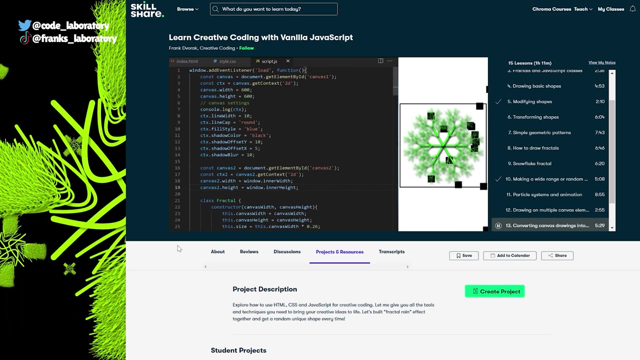 where I write everything in object-oriented code structure, again with plain vanilla javascript and no libraries. You can take what you learned today further and you can design your bloody stance randomised fractal as a PNG image by right-clicking on canvas and you can tag.